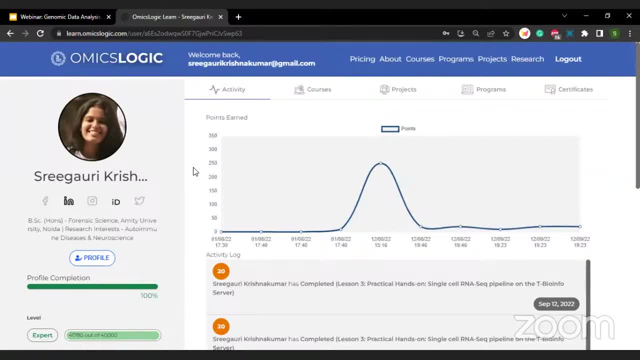 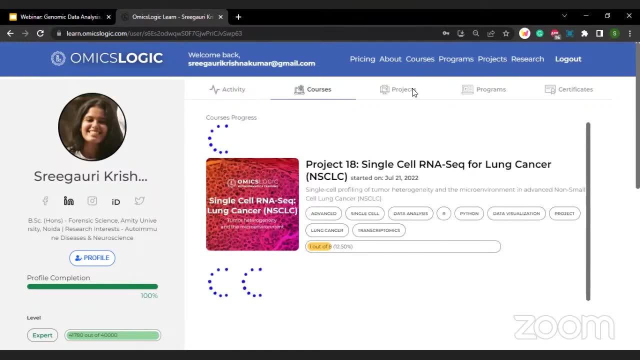 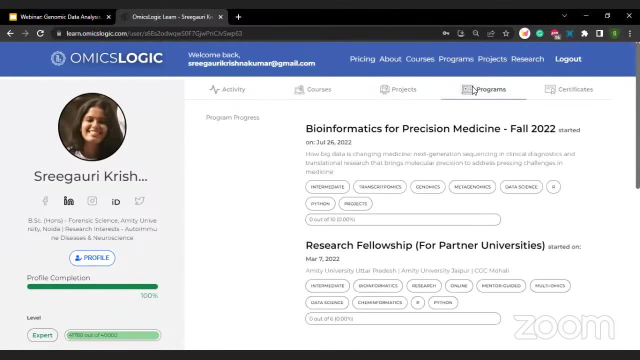 activity tab, the mentor and the community manager will be able to track your progress. Under the courses tab, you'll be able to view the present courses that you're taking and the projects will show the if you have completed any projects under any programs, and here it shows the programs that you have enrolled. So with that, now I'd like. 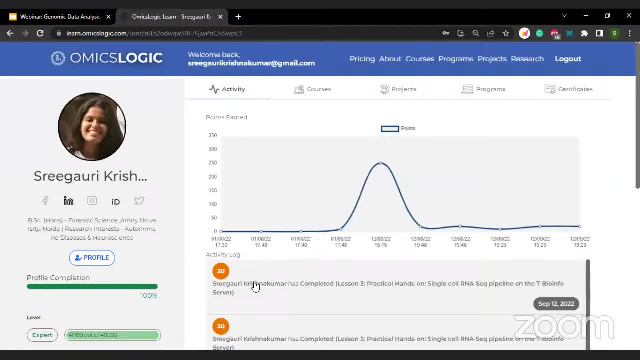 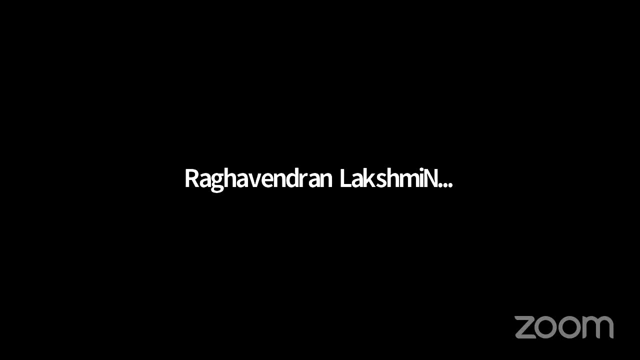 to pass on the stage to Dr Raghav to begin with today's webinar. Over to you, Dr Raghav. Thank you very much, Shri Gowri, and let me find ways to share my screen. Please confirm you can see my screen and also you can hear me. 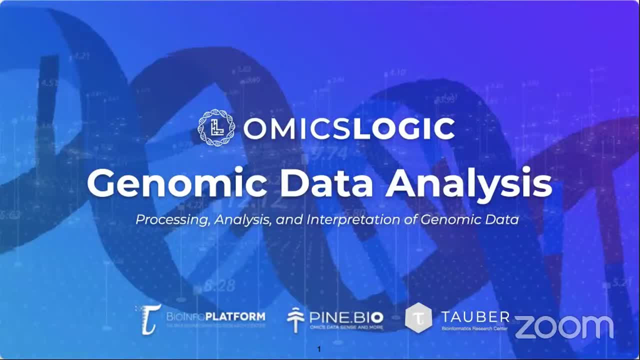 Yes, both are working fine, Thank you. Okay, perfect, Thank you very much. So welcome to the orientation, or webinar, of genomics data analysis. Let me set it up. Today we will be having an introduction to what this program has to offer to. 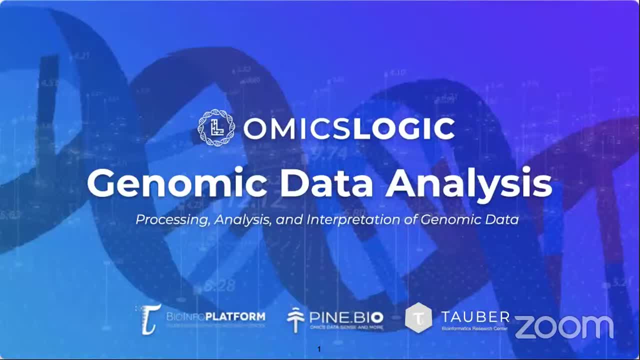 us and we will also have a good introduction to different resources in AmixLogic platform and also the associated HubBot BioInfo platform. We will also have a good introduction to different resources in AmixLogic platform and also the associated HubBot BioInfo platform and also the associated HubBot BioInfo platform. 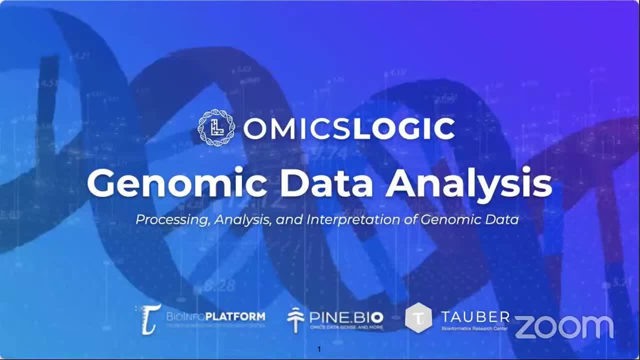 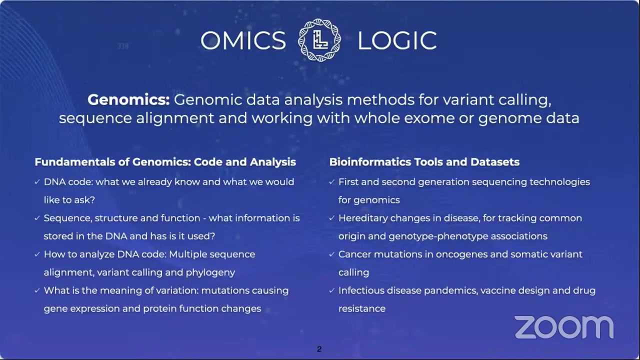 With which, what we can do with genomic data analysis, what we can learn, and we will quickly go through a couple of demonstration that will help us to annotate, let's say, for example, very well known cancer driver gene, one of the very well known cancer drivers. So we already spoke about that. We will start with what is genomics data? 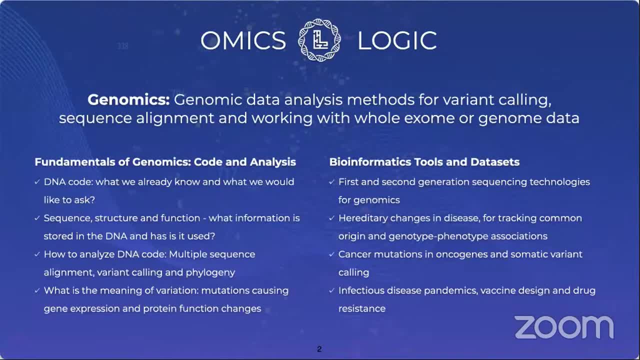 how is it organized and how is it analyzed and how is it interpreted to be such a powerful resource in the hands of researchers like you, in the hands of clinicians and also in the hands of entrepreneurs that are reading the code of DNA to battle cancer, to fight infectious? 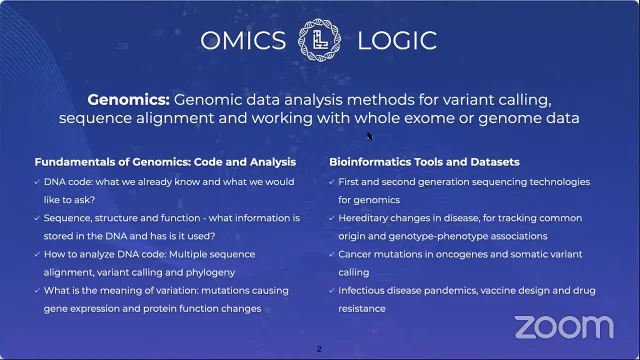 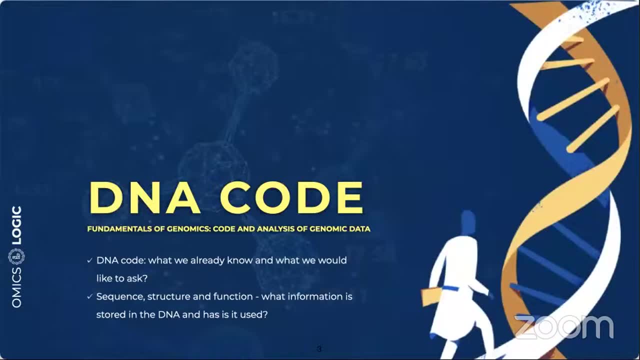 diseases and even sometimes to an extent, to solve crimes. So let's start by reviewing the fundamentals of genomics. Genomics is all about DNA, so let's review. what is this DNA code, what do we already know about it, and what kind of answers can we find there and how can we analyze? 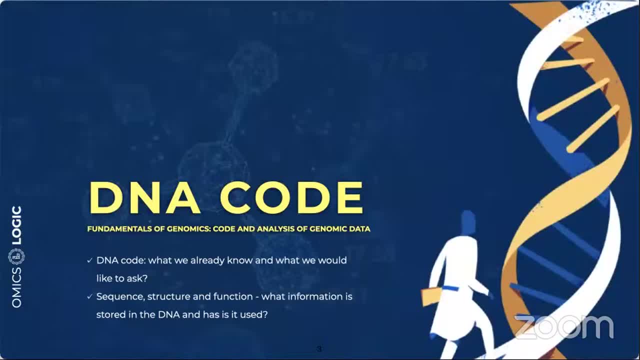 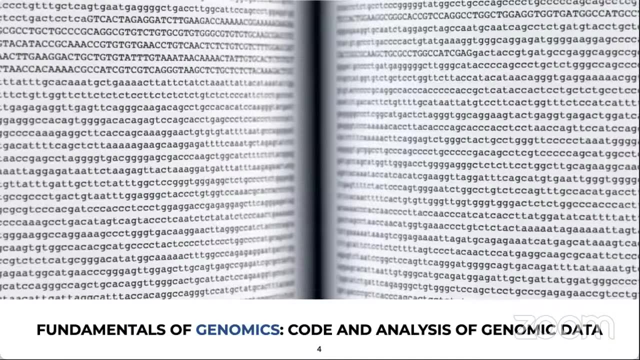 huge sequences of nucleotides stored in the DNA. and how do we make sense of them? Just pretend to be a book. just like a book, DNA code is organized letters that form sentences, and sentences could form paragraphs, and paragraphs are organized into chapters, and knowing how to read this code can actually help us decipher the full story about who we are. 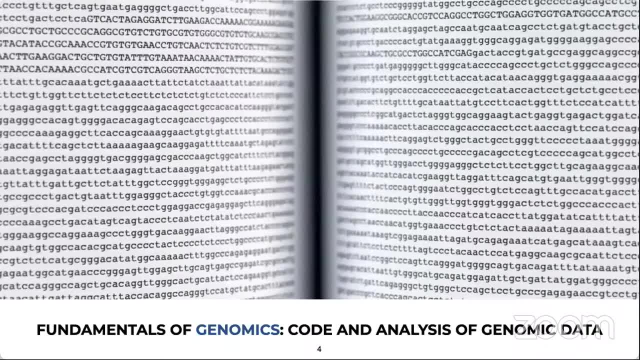 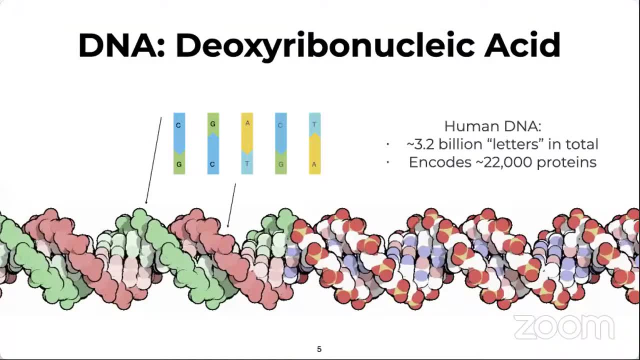 and we can look into our history, we can understand how we are connected to other living things that are living around us. so dna is short for deoxyribose nucleic acid. it is a long molecule composed of two chains of coil that go around each other to form a double. 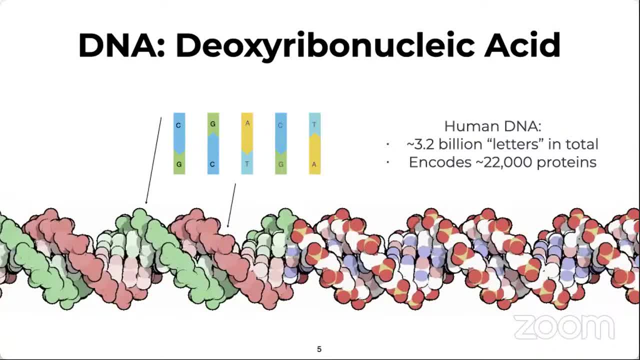 helix. this carries genetic instructions for development, for the function, growth and reproduction of all known life. right this, these all known life forms, include multi and single cellular organisms, as well as many bacteria and even some viruses. yeah, so human genome, for example, has three billion base pairs in one. uh, yeah, in one. 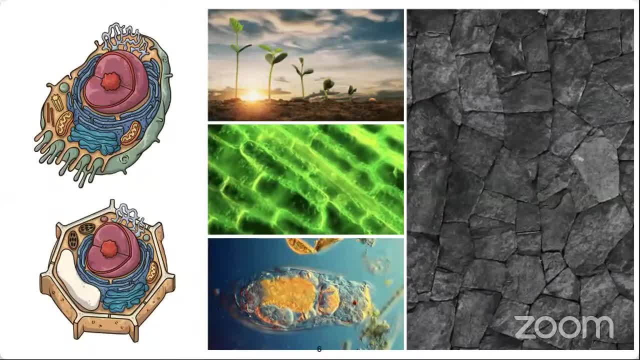 chromosome. okay, uh, so a dna code contains directions or it contains recipes for life. life is a condition. how can it be defined? it can be defined that it is a condition that distinguishes animals and meccas weighing, different kinds of animals from animals and plants from inorganic matter. 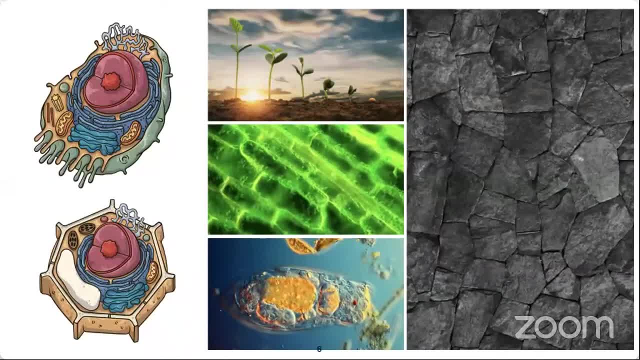 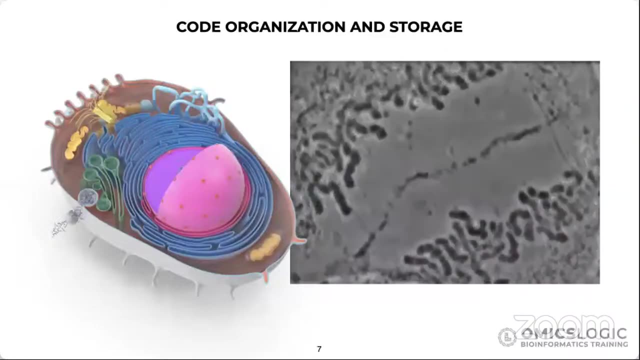 that this condition could include the capacity for growth, it could include reproduction, it could include functional activity. it could also include continual change preceding death. So this instruction for life, include life of a single cell and an organism like us humans, which contain over 37 trillion cells among us right. 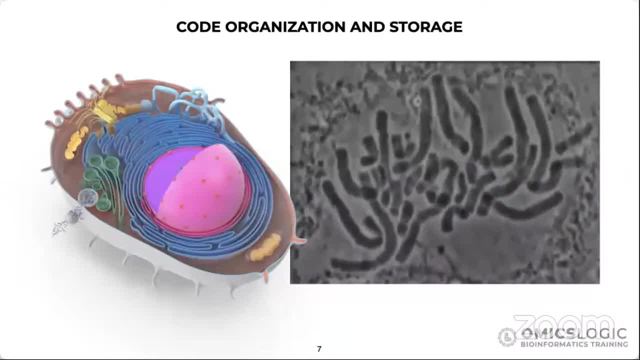 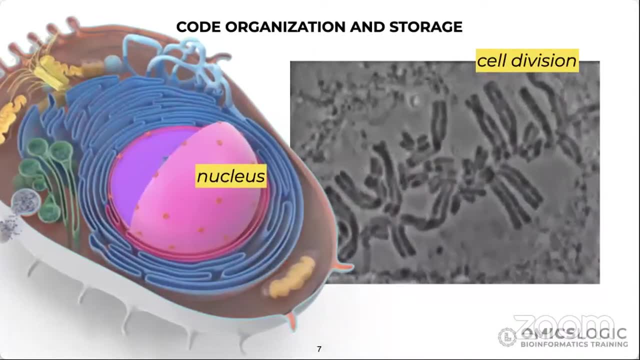 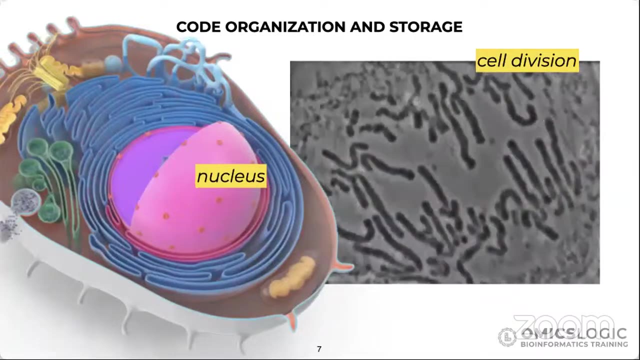 Each cell contains the same DNA, which is stored tightly inside a nucleus. When the cells divide as they do, when a new organism is formed or when a new cell has to be generated, we see how this DNA is organized. So we get a hint about this organization of this DNA. 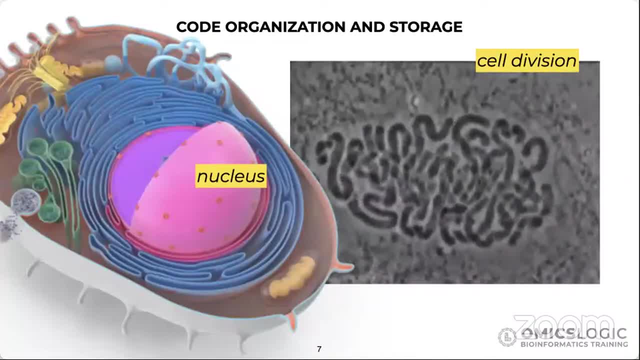 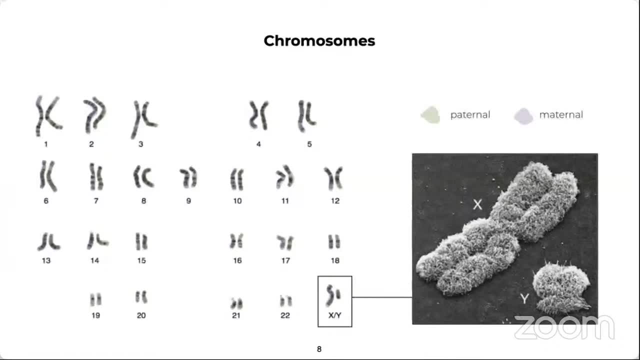 into chromatins and other forms. The nucleus is opened up and inside we discovered these tightly packed strings that can be visible under low power microscope also. So we already saw that it could be tightly packed into 23 pairs of chromosomes right. 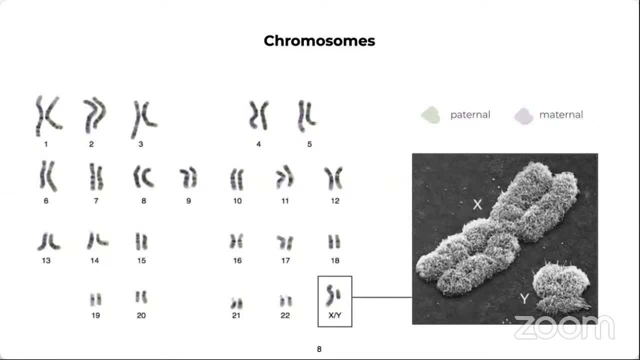 One of the chromosomes come from our mother and the others come from our father. right. The unique structures of these chromosomes will keep the DNA tightly wrapped around the spool like proteins called histones. Without such packaging, these DNA molecules would be too long to fit inside the cell. 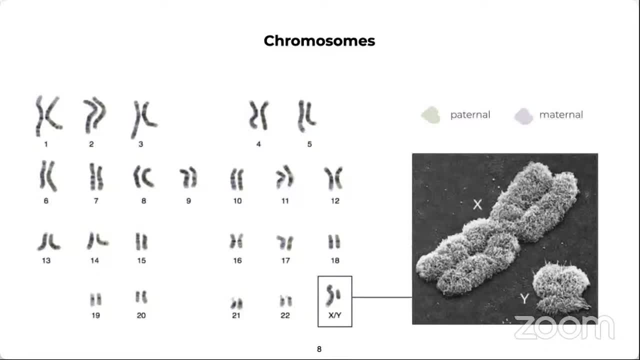 For example, if all of the DNA molecules inside a single human cell were to be unbound from their histones and placed end to end, they would stretch up to six feet. The largest chromosome, which is chromosome one, contains about 8,000 genes. 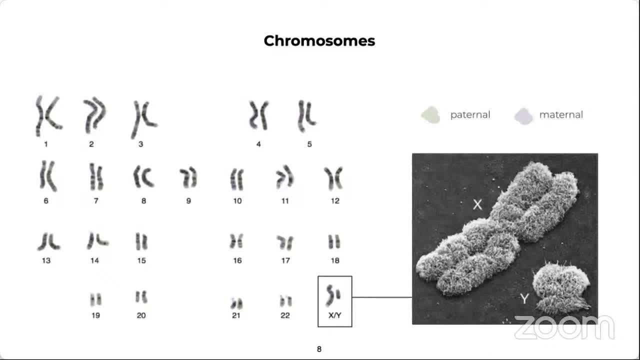 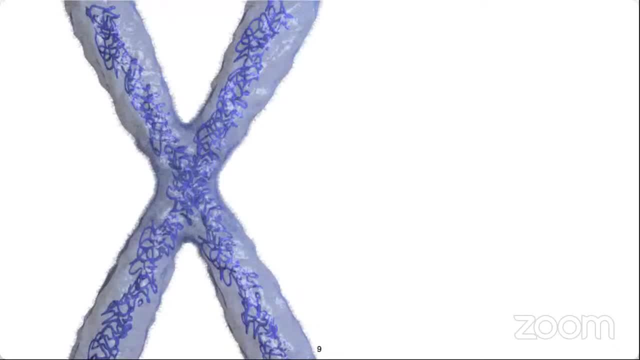 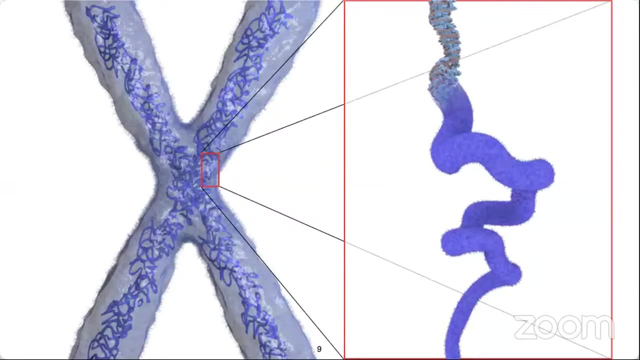 And while, to compare, the smallest chromosome- chromosome 21,, contains only about 300 genes, And once the cell division is complete, the information on the cell function stored inside the DNA gives the new cell know what to do to continue the function. 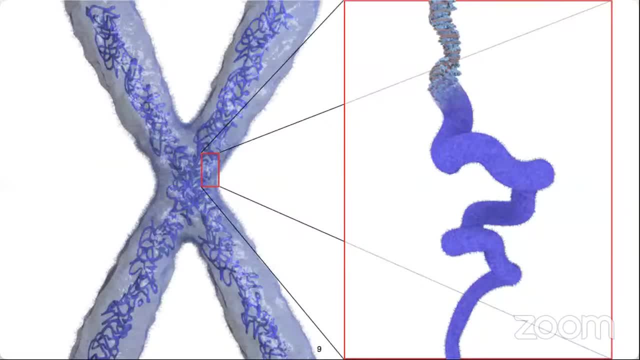 It will work on for the rest of its life and preserve the DNA to pass it onto the next cell that it will form when it divides. And in the meantime, the DNA contains instruction for various functions a cell must perform to grow and maintain this life function itself. 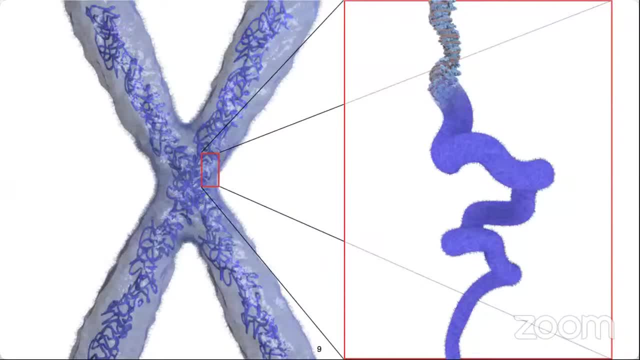 So, therefore, the DNA code contains both actively needed recipes and all kinds of other instructions that need to be stored but not necessarily used all the time. So together, all of the specific code in a chromosome can be termed as a genotype. Yeah, my animation stopped working suddenly. 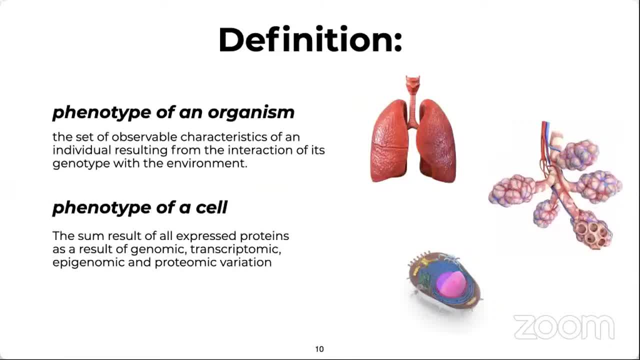 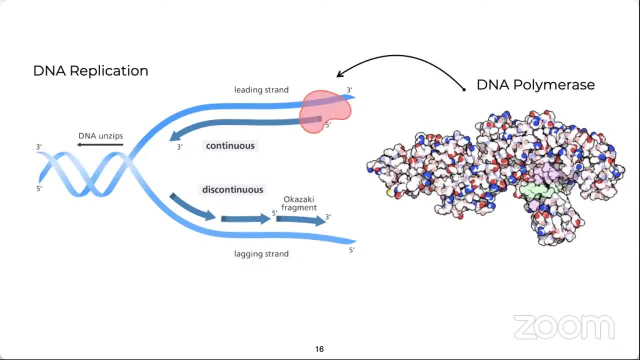 be a single cell, a tissue, an organ or the whole organism. The phenotype of an organism might in fact single strand, adding complementary basis and creating a second copy. this copied code can then be used in another cell, but is important to make such replication go. it is important to 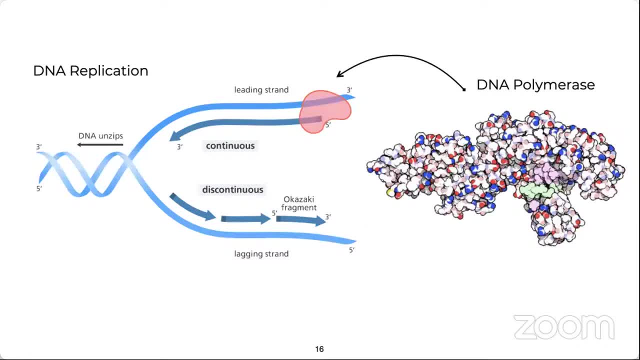 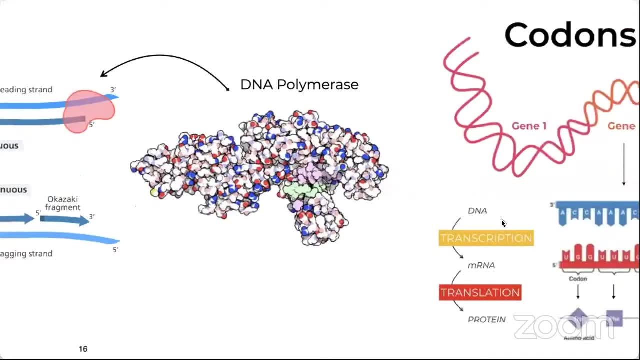 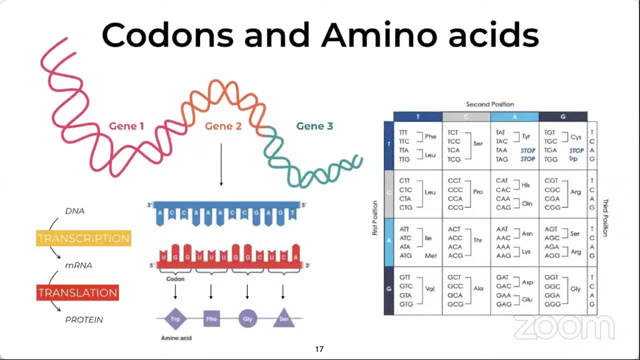 make sure that this process goes without any mistakes, so a lot of cells instrumentation are designed to prevent such mistakes while carrying out these processes. each gene is a recipe for specific protein, so it encodes instruction from this from which a protein can be made right. the proteins are actually product of amino acids which are encoded by tri-nucleotide. 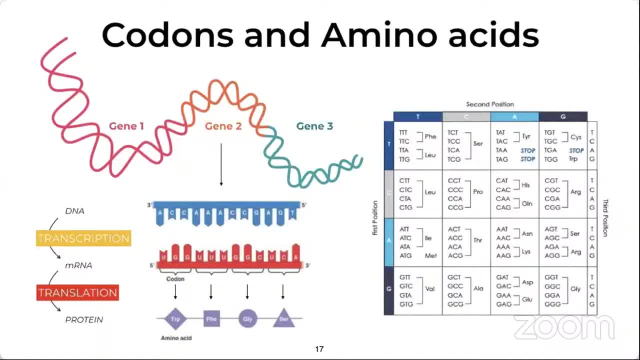 codons that are stored on the DNA. so a codon is actually a sequence of three nucleotides that corresponds to a specific amino acid or a stop signal which will stop the production of this specific protein once the right place on the DNA is copied over. it is prepared by translating: 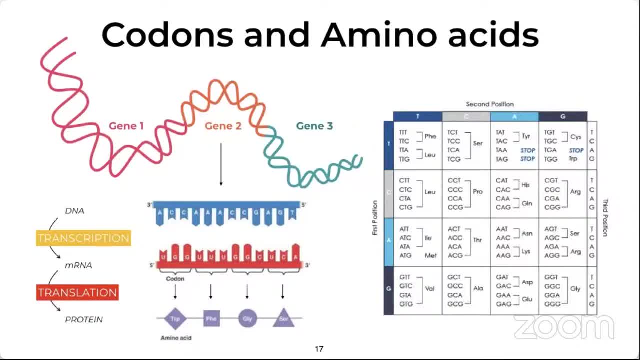 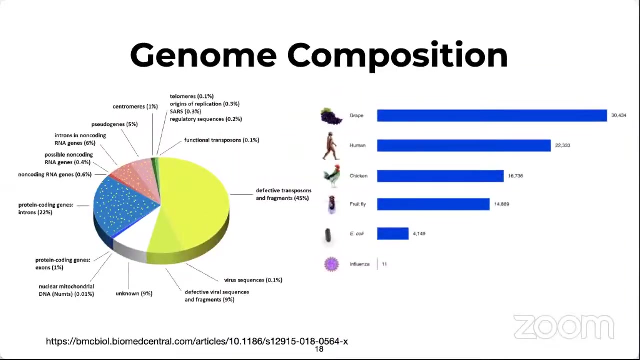 this into a. it is prepared for translation by forming a messenger RNA which is exported from the nucleus into the cytosol, where this messenger RNA is actually translated into protein. again, my this is running soft, okay. so in human cells alone, genes vary in size from few hundred. 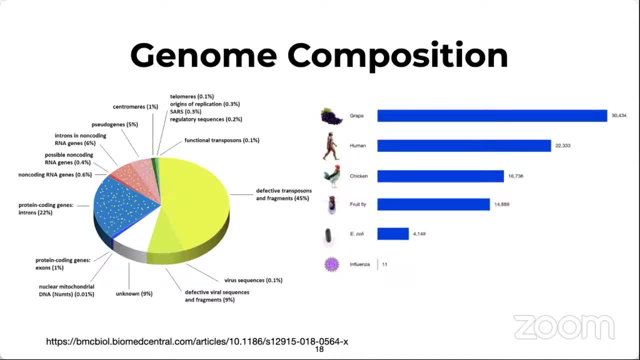 DNA bases to more than two million bases. for example, the keratin associated protein is the protein that is in the cell, and the protein that is in the cell is the protein that is in the cell and the protein that is in the cell is the protein genus. 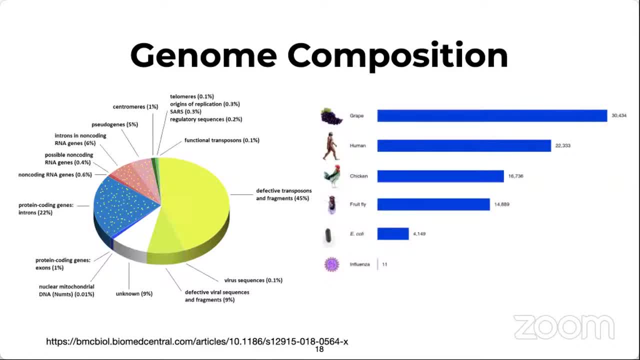 the protein gene, like kr tap, is the smallest gene that we have characterized until now. it is only 447 nucleotides long, whereas cntnap2 gene, for example, has over two million nucleotides. the number of genes also vary between various organisms. for example, influenza virus has 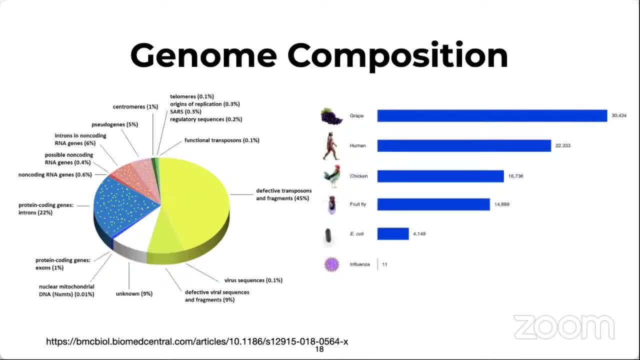 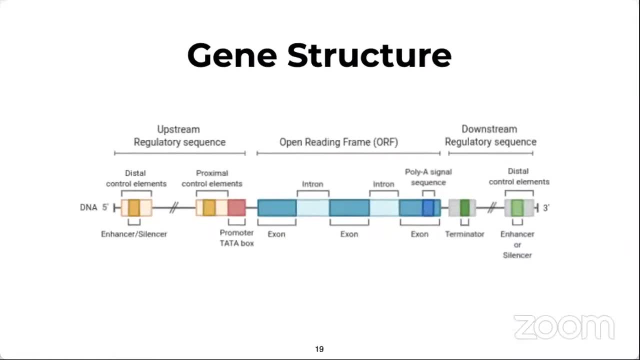 only 11 genes, while the grape genome has over 30 000 genes. genes are not just a simple organization of sequences of nucleotides. in fact, they have upstream and downstream regulatory sequences that controls the transcription of these genes. inside the gene sequence itself, there are codons and there are introns that undergo splicing. 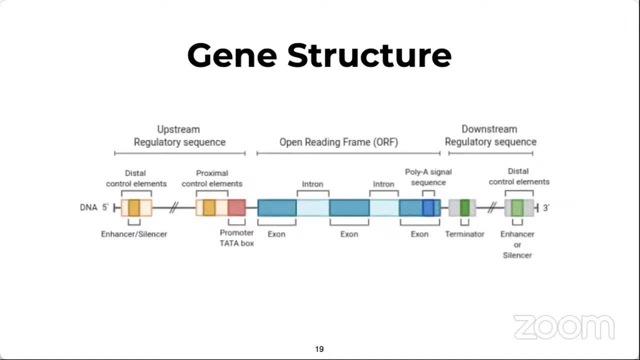 before a gene is translated into protein. the extraordinary length of some of these genes is enabled by the presence of introns which, as a substrate for which acts as a substrate for insertion and deletion of several transposable elements. this also provides a mechanism for the generation of diversity through alternative combinations of these exons, which is also known. 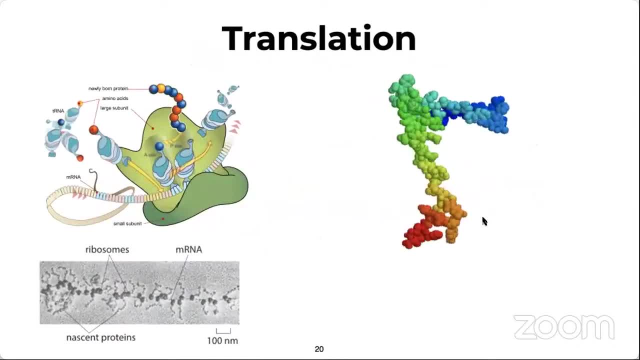 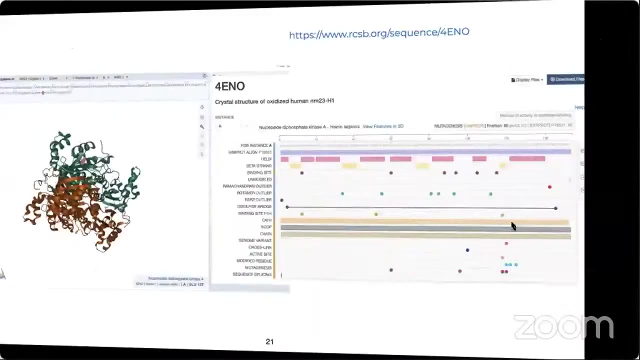 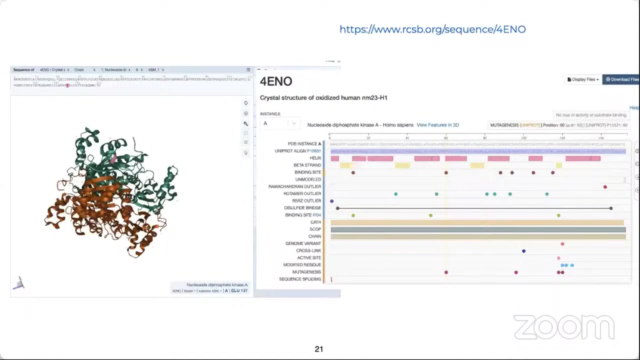 as splice forms. so the translation in the cell is done by the ribosome which can read the mRNA sequence and assemble a protein, the that will fold into a functional structure. When we want to understand the function of a particular protein, we typically combine the information about its chromosome position, its coding sequences, its regulatory region. 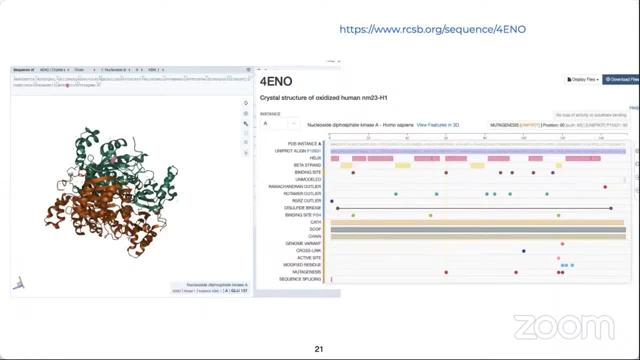 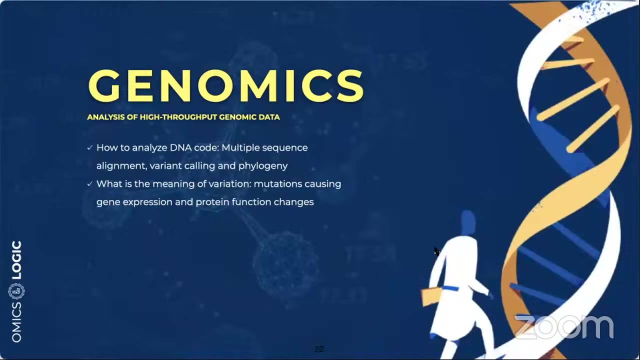 the structure of the protein, as well as the functional features of the protein through various experimental validation and through various bioinformatics comparative analysis. So before going into how this DNA could be analyzed and how they could be understood, I want to stop here and ask if you have any queries or questions. until now, 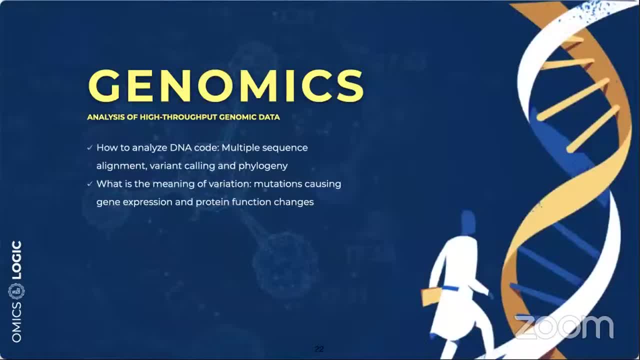 If you do not have any questions, please let me continue, And if you have questions, please put it in the chat box. I am following the chat box, so we will address your questions as we go by. So that is a short introduction about the DNA. 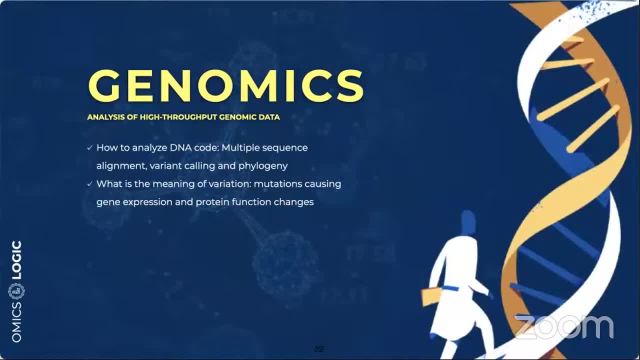 It is organization, genes, and how they form basic, fundamental element and functional element of any, each and every cell. Now let us see, or let us discuss, how to analyze this DNA code and what are the information that we are going to extract from analyzing this DNA code. 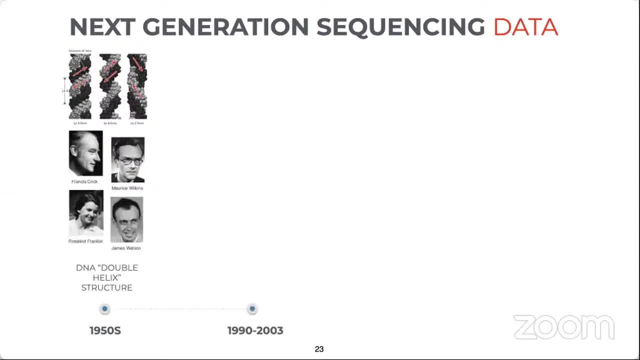 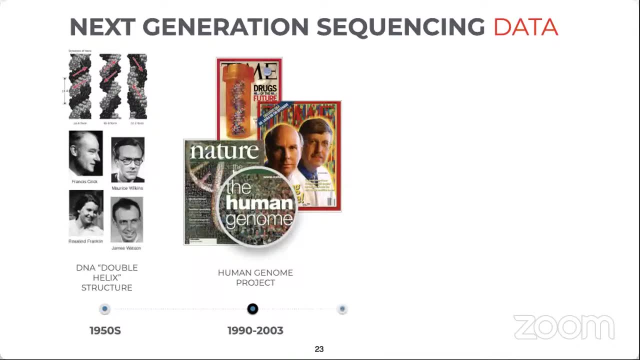 So we recently crossed the 70-year mark since the discovery of structure and function of the DNA molecule, And it took something around 50 years from the time to sequence the first human genome. But soon after that point the technology developed so much that the availability of 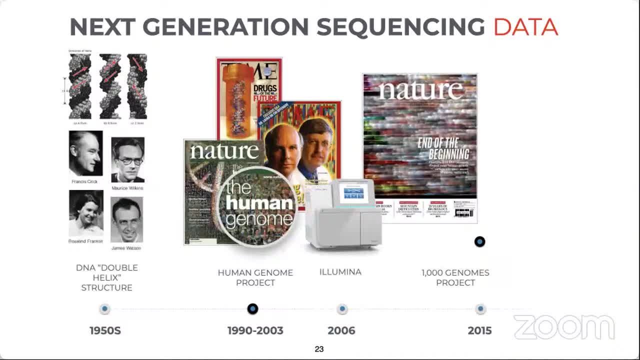 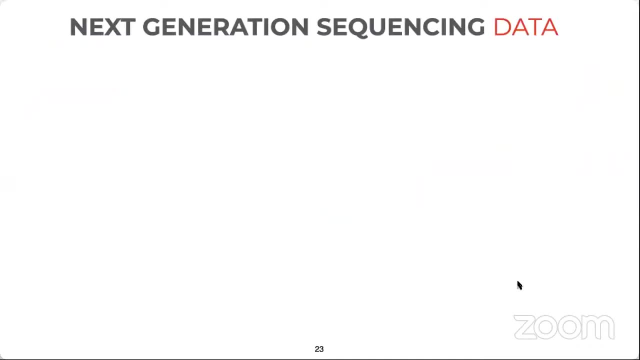 the human genome just exploded rapidly, So by around 2015,. 1000 Genome Project was launched and it brought actually significant number of whole genome sequences into the research community. And again it went too fast. Yeah, Let me discuss this. 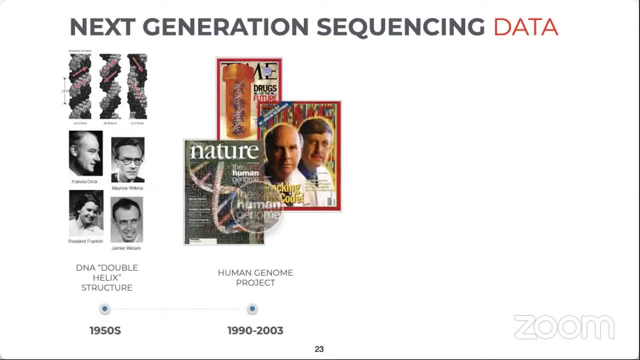 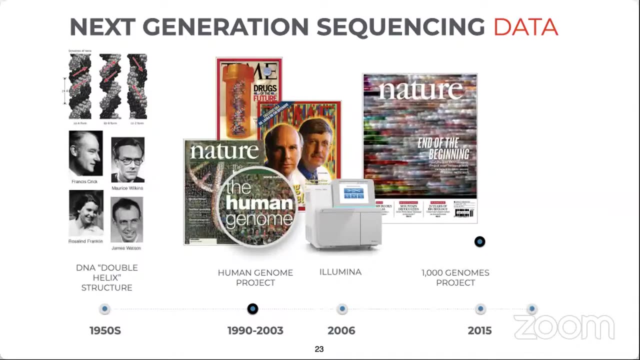 So non-coding RNAs are also part of the part of the gene or genome, not actually genome. So they serve specific function in regulating which part of, or which gene are actually translated by how much. So now several important functions of the long and short-term genome. 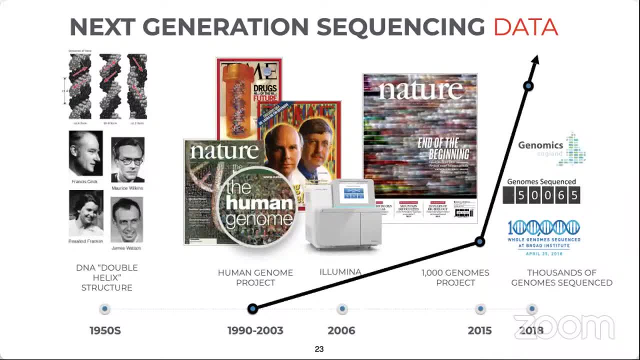 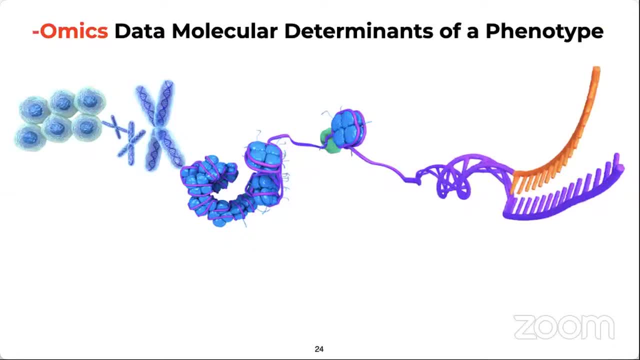 We have found that the functions of the long and short non-coding RNAs are actually actively be identified and actually being discussed, and their participation and their role in regulating these genes could actually serve as a purpose to understand several disease state of the cell or several altered state of the cell. 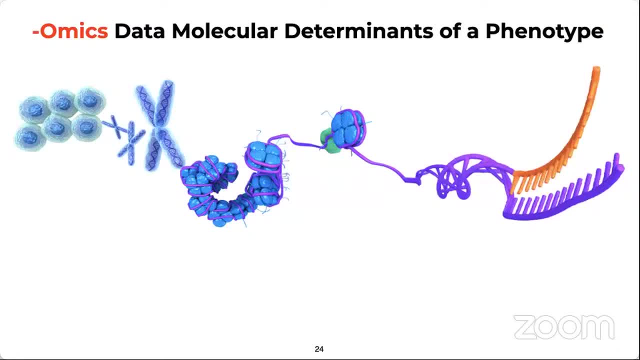 So collectively. the omics aims at characterization and quantification of the different biological molecules. Yes, we can use several available samples. Yeah, public genomics database like NCBI and etc. are part of that. So to know more about how to use. 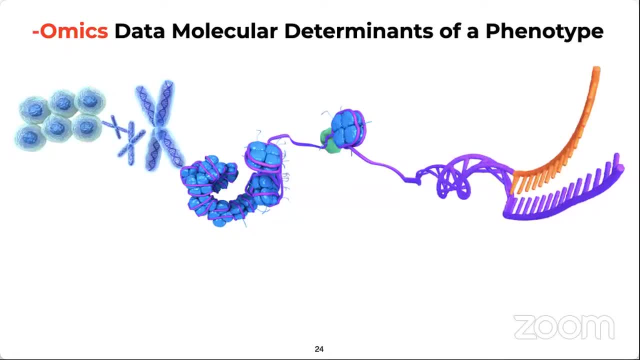 these databases for what kind of data and what kind of analysis. the program actually discusses a lot about that and how we can leverage the publicly available resources for our own research, So let's continue with that. We were discussing about the omics data in particular. So the omics- 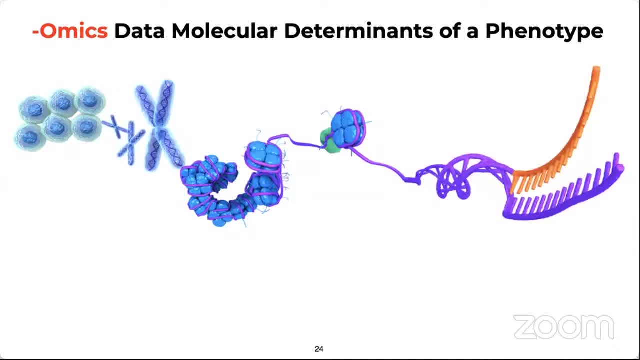 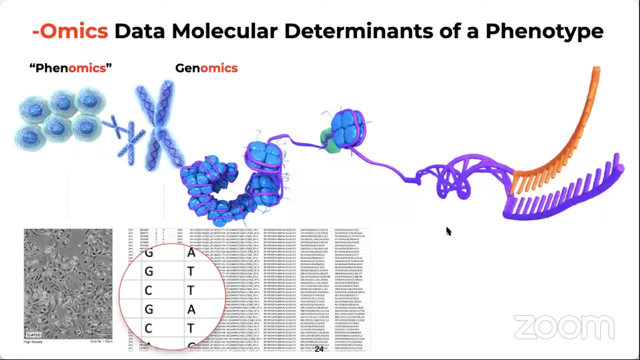 data aims at collective characterization and quantification of the biological molecules that translate into structure, function and dynamics of an organism. The omics technologies are used to explore the roles, relationships, actions of various types of molecules that make up the cell of an organism. Many type of these omics data can be generated using next generation sequencing. 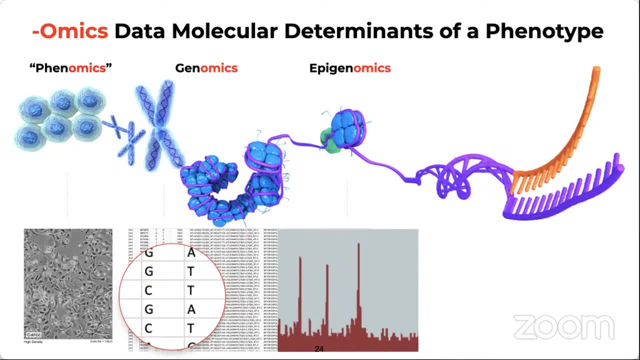 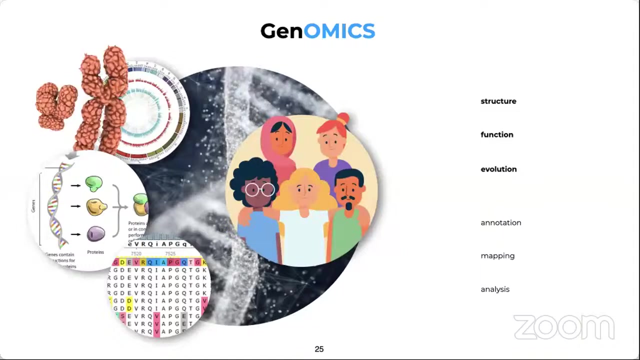 technology, which is also known as high throughput sequencing technology. The data can show details of the omics data and the omics data can show details of the omics data and the information about genomic variants, about epigenetic variants and about transcriptomics, expression pattern of genes and isoform level also. So the suffix om actually defines or refers. 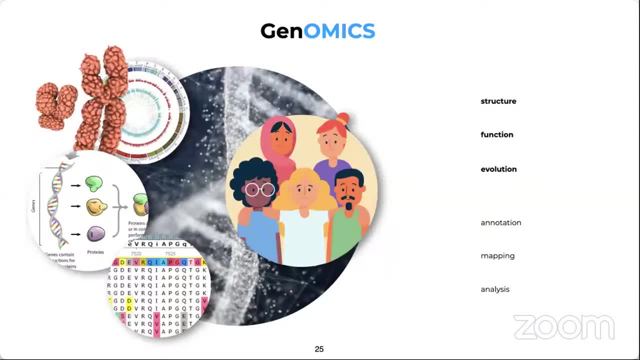 to the various or referred to various field of omics in molecular biology and bioinformatics. refers to a totality of all analysis of all of these different omics. For example, the word genome was actually first coined in Germany in the beginning of around 20th century. The word genomics refers to the totality of the genome or the studies of. 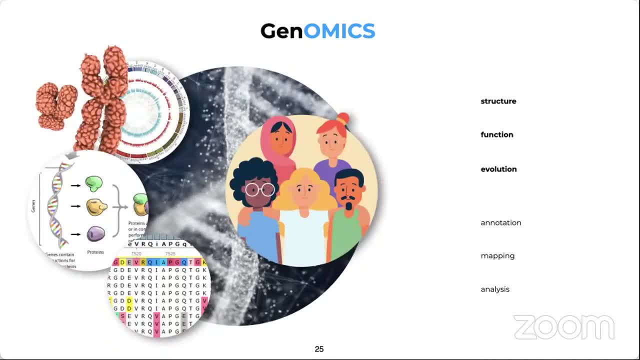 genomes. Genomics actually itself is an interdisciplinary field of biology focusing on the structure, function, evolution, mapping and editing of genomes. The genome of an organism is a complete set of DNA, as we discussed, and this includes all of its genes, in contrast to very well-known branch of biology, genetics, which refers to. 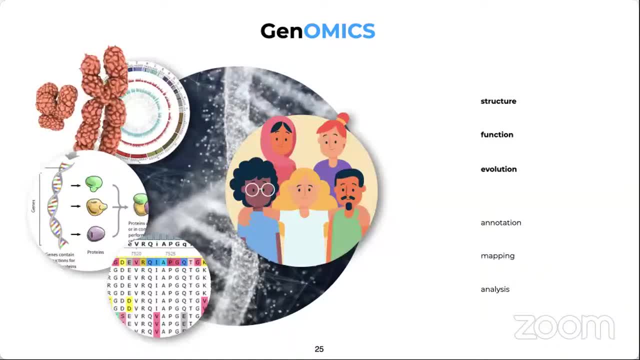 the study of individual genes and their roles in inheritance. Genomics aims at the collective characterization and quantification of an organism's genes and their relationships and influence on the organisms. What happens to the introns after protein synthesis? So sometimes they are actually discarded right. 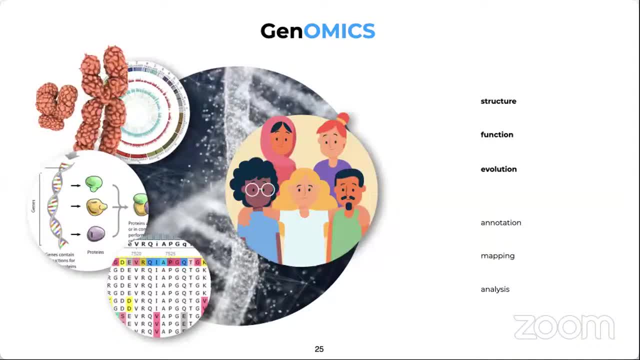 Only exons, which are which form part of the mRNA sequences, are actually exported to the, exported to the cytosol where protein synthesis takes place. Introns do not cross the or several known introns right. 99 percent of the introns do not cross the boundary or nucleus nuclear. 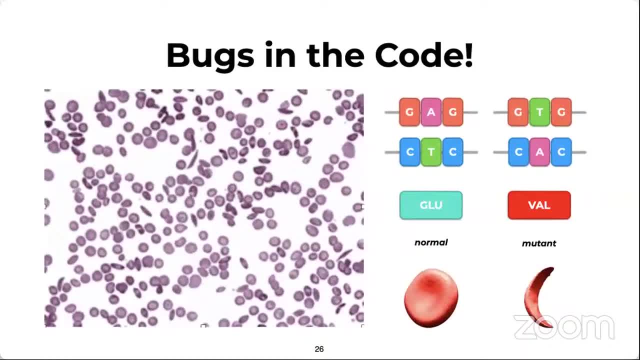 membrane as such. So what do we do by? what do we mean by study? studying genomics, right, As a result of a lot of genomics efforts, we can now detect differences which can be harmless, or we can detect differences which can lead to serious issues. 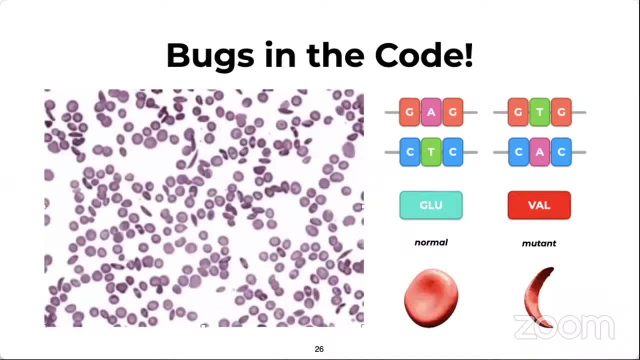 when a gene is produced, The whole study of genomics is centered or focused on identifying specific differences, what we term as variants, or mutation or polymorphism, which we will discuss in further slides. in the available DNA sequence right, These can actually occur as a result of: 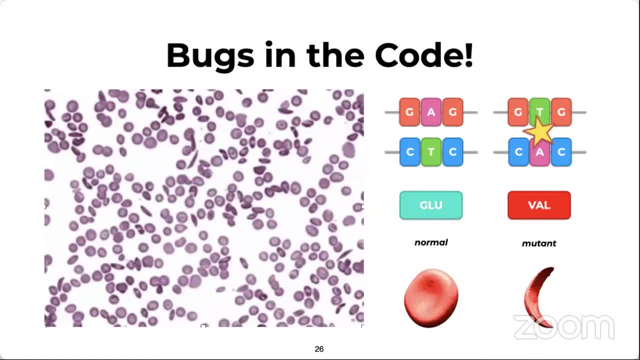 copying the DNA source too many times or as a result of various stresses that can interfere with the regulatory mechanisms, or it can happen in several different random ways, also right. And once such variation or such mistakes or mutation occurs, the end result can be: 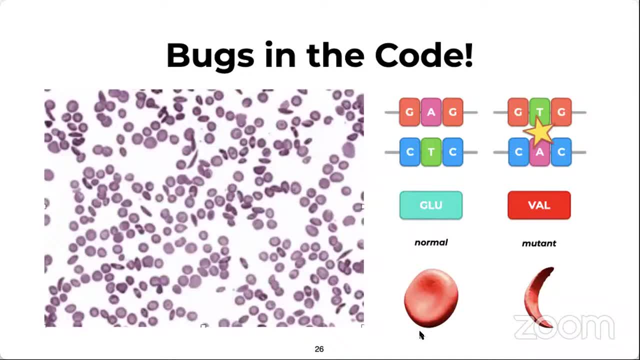 devastating. This is something for the organism or the cell in particular. For example, here one single nucleotide change results in an amino acid change that completely changes the shape of this red blood cells, which leads to a very popularly characterized condition called 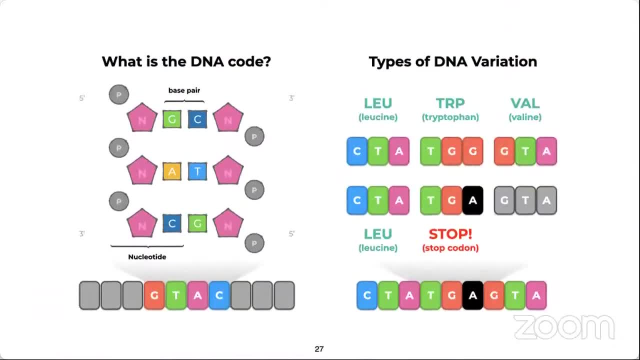 sickle cell aminia. So to understand how genomics is used, first we have to understand the analysis approaches to DNA codes, specifically what we can understand, we can identify, how we can identify these changes and how we can characterize them. and 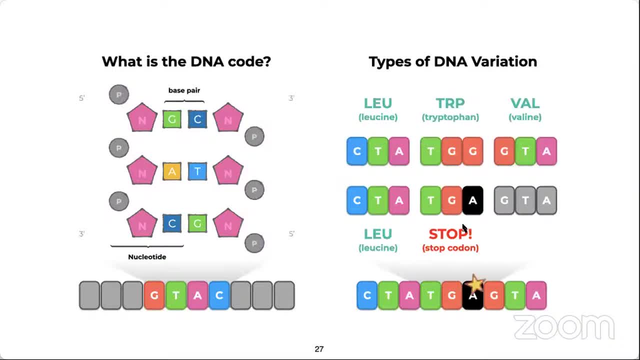 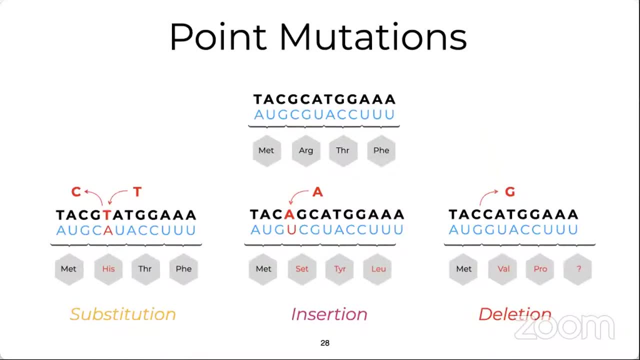 how we can interpret their significance. This we spoke about. So there are several mutations, as we spoke about, several changes to the DNA code, and what are these changes and how can they be characterized and categorized? We can refer to some of the mutations or changes as substitution mutation. 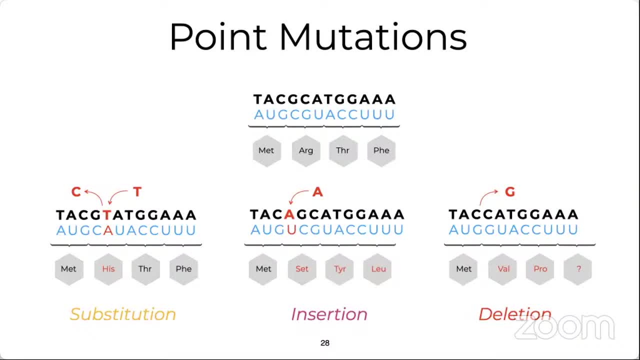 A substitution mutation can cause several consequences to the DNA code, but it implies a minimal change that only leads to a single nucleotide change. Whenever a change in the nucleotide or change in the copied DNA sequence results in a change in one nucleotide level- change at one nucleotide level- that is termed as substitution mutation. 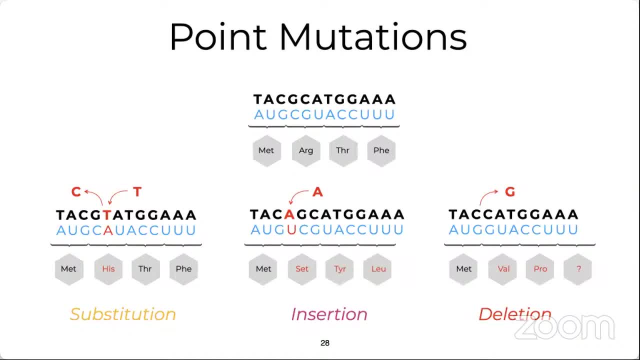 And while an insertion mutation can be defined as an insertion of a new nucleotide to the copied DNA sequence, compared to the template DNA sequence, This insertion changes the number of DNA bases in the gene by adding one or more pieces of DNA. As a result, the protein made by the gene may not function properly because it now encodes. 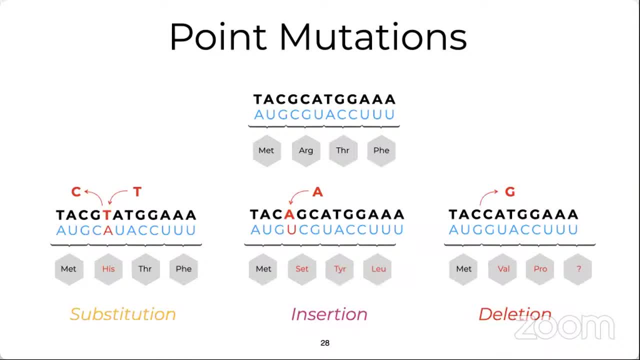 completely new set of amino acid sequences. Okay, Okay, So deletion mutation actually refers to removal of one or more number of nucleotide base in the copied DNA sequence compared to the template DNA sequence, And this deletion actually changes number of DNA bases by removing a piece of DNA. 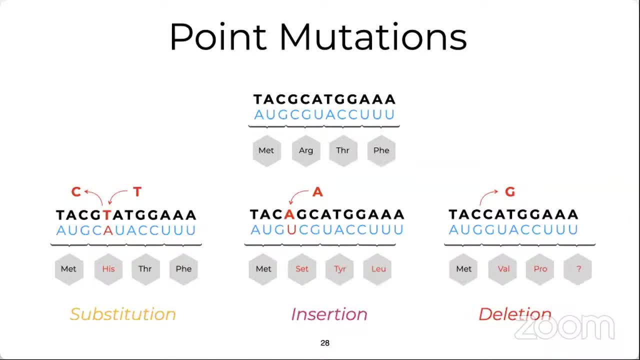 Small deletions may remove one, or large deletions may remove an entire gene or several neighboring genes. This will definitely alter the function of the resulting protein, as we discussed with the insertion also, And as the deletion mutation may result in the complete change of the encoded protein. 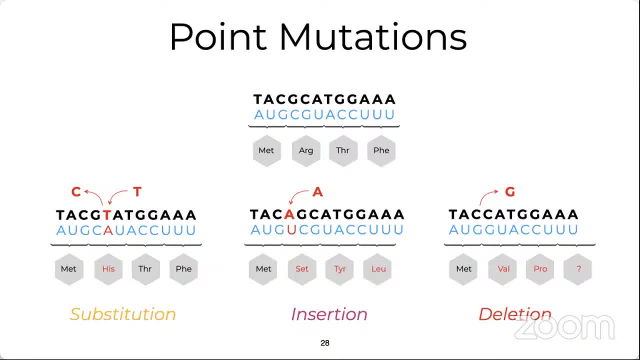 sequence, which will now change at the structural level and also at the functional level. So, and while there are also other variations that are possible, like gene duplication or duplication of regions that are abnormally copied one or more times, The type of mutation, Yeah. 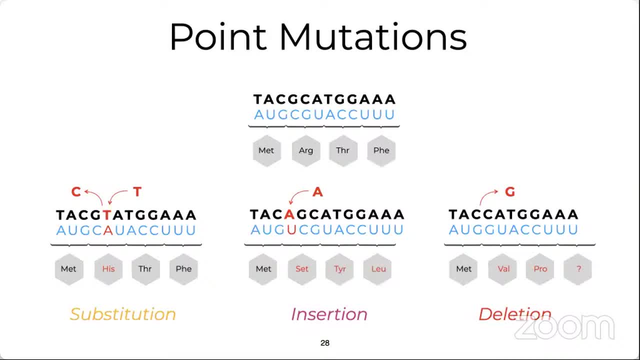 This type of mutation. This type of mutation may also alter the function of the resulting protein. Every type of mutation that we are actually dealing with has to end up- or interesting only when it ends up- at the level of functional implications to the protein that it enters. 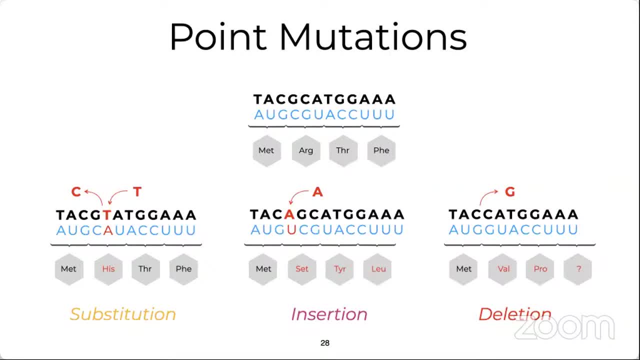 And point mutations are nothing, but when all these variances or changes occurs at one nucleotide level, When the substitution is always point mutation And when the insertion occurs at one nucleotide level. And when the insertion occurs at one nucleotide level And when the insertion occurs at one nucleotide level. 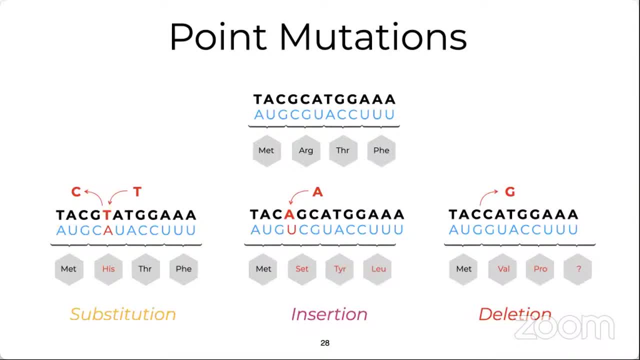 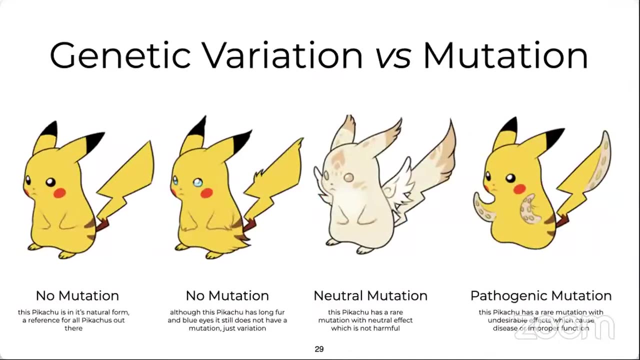 And when the insertion occurs at one single mutation level, a single nucleotide level, and deletion occurs at single nucleotide level, and those are all termed as point mutations, as the change occurs in single point of the genomic position. So there are two basic terminologies that we need to be very clear about. 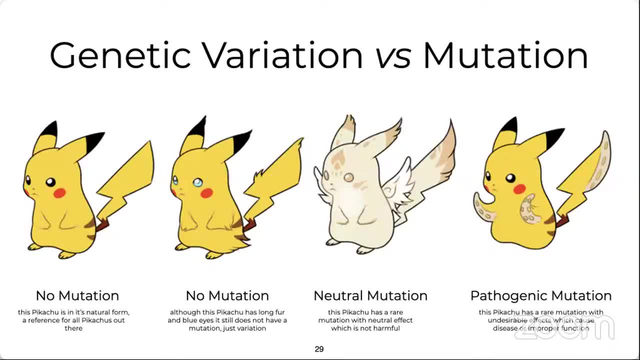 We term some some of the changes as genetic variation And certain other changes as genetic variation. So there are two basic terminologies that we need to be very clear about. We term some some of the changes as genetic variation. So there are two basic terminologies that we need to be very clear about. 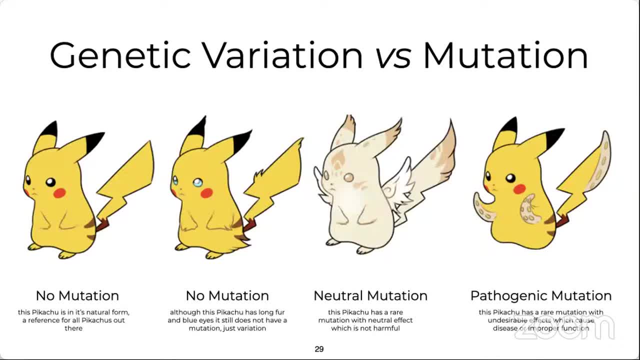 We term some some of the changes as genetic variation And certain other changes as genetic mutation. A specific type of variation that leads to harmful results, For example a change in function that is harmful, are termed as mutation. For example, if you see this graphic, we have the wild type icon or pikachu here and while 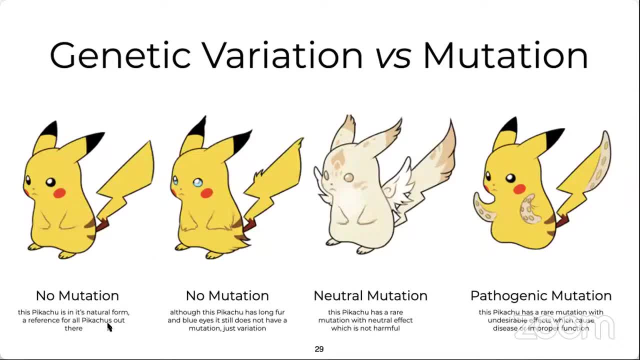 there could be several variations for the genomes that compared to the wild type variant of this pikachu, And these variation will produce noticeable change in the phenotype or morphology of the organism, like blue eyes or hair, but like a lack of the fur or lack of pigmentation. 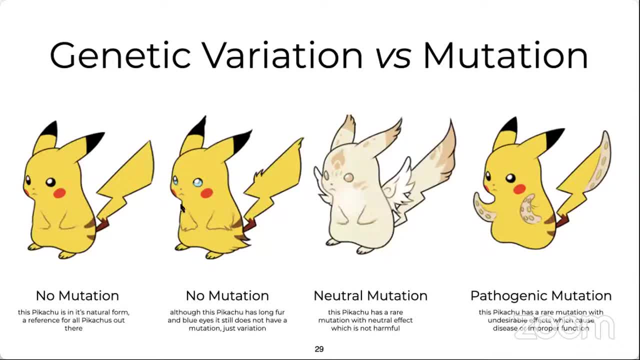 But these and also addition of new features, but these are not supposedly dangerous or supposedly harmful to the organism itself. When the variation that we are studying are not generally harmful to the organism themselves, then they are. these changes are termed as genetic variation. 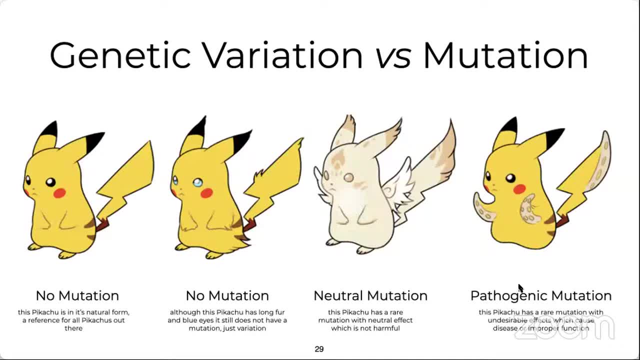 But while when this variation results in harmful changes or results in loss of function or complete alteration of function that leads to abnormalities in the organism themselves, then they are termed as pathogenic mutation. So we refer to mutations, and, And they are always annotated or they are always associated with harmful end result and variation. 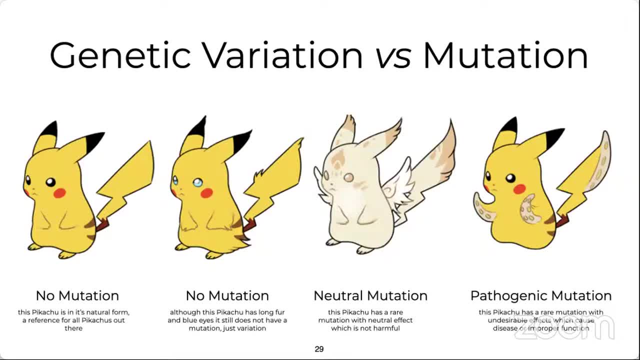 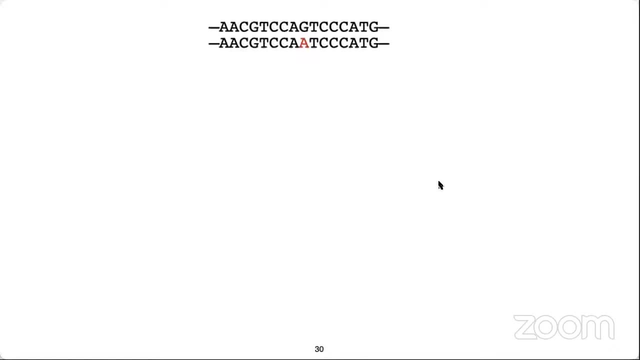 They are always associated with unknown consequences or consequences that are generally accepted to be less harmful, or no known harmful effects identified for those genetic variations. So when these genomic variants are often discussed, we use both mutation and variant, And also sometimes polymorphism is also used several times. 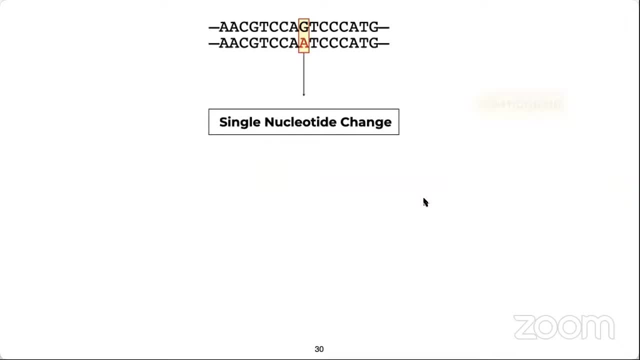 By convention, human genetic research, any genomic variant with the population frequency of less than 1% is called as mutation, And whereas the variant with the population frequency of more than 1% is called as polymorphism. For example, if I am studying a sample of more than 1% of the population, 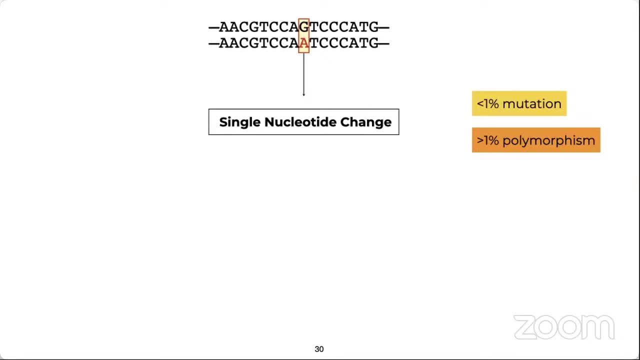 The people or ethnicity that I want to study about and all the variants that I am observing in more than 1% of those sample sizes, right of those population sizes. I have to name them or I have to turn them as polymorphism and less than 1% of variants at the population level, not at the sample level. 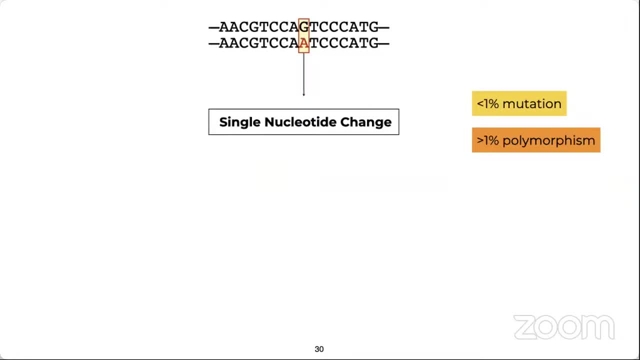 At the population level should be termed only as variants or mutation, depending upon their, Depending upon Their pathogenicity, right, Let's name it that right? This distinction actually is based on population frequency rather than the sample frequency, as we actually discussed, right? 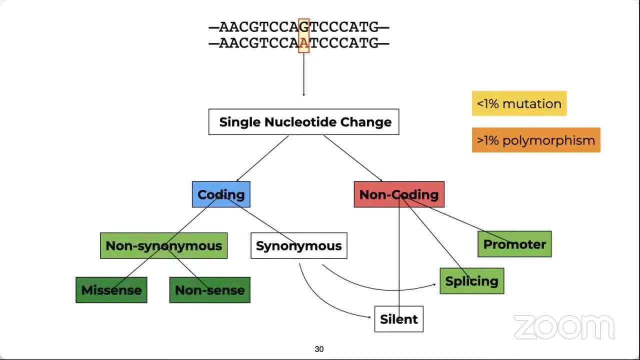 However, as a rule, a rare mutation tend to have functional impact that deviates from wild type, while, in contrast, polymorphisms generally connote to less functionally deviant genomic variants. right Generally, when we refer to something as single nucleotide polymorphism, we refer to only those changes, or mainly to those changes, that are less harmful or that are known to harbor the changes at the phenotypic level that are not harmful to the races. 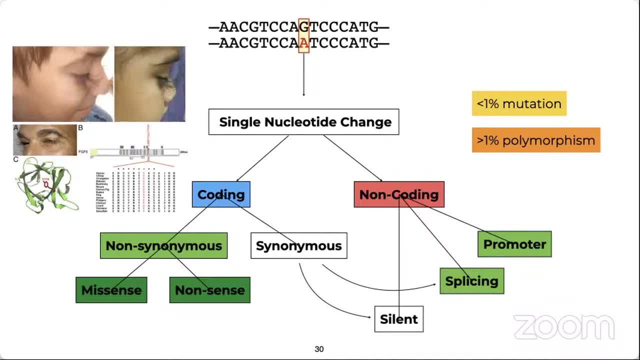 For example, to discuss an example, the very well-known blue eyes of Caucasians in Europe, and also some of them in America, is a result of set of single nucleotide polymorphisms in the gene. Okay, Okay, Okay, That corresponds to pigmentation in our eye level, right? 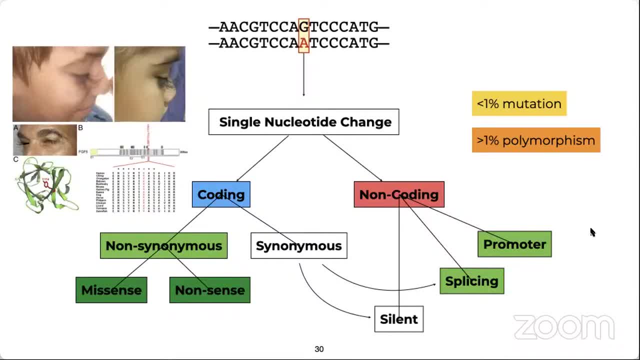 At the eyes, for the eyes, And while mutations, however rare they could be, they can result in some serious effects. A good example of such mutation that causes serious changes at the phenotypical level is at the FGFS gene that causes extremely long hair to grow at eyebrows and eyelashes. 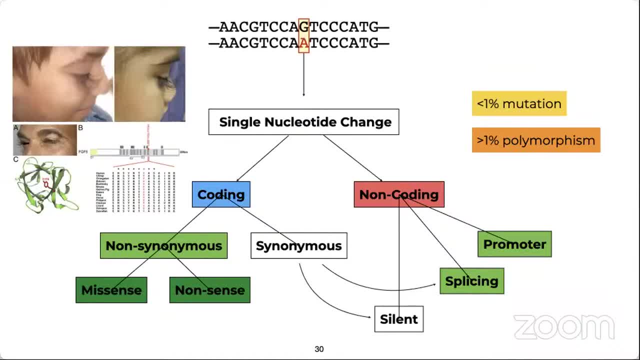 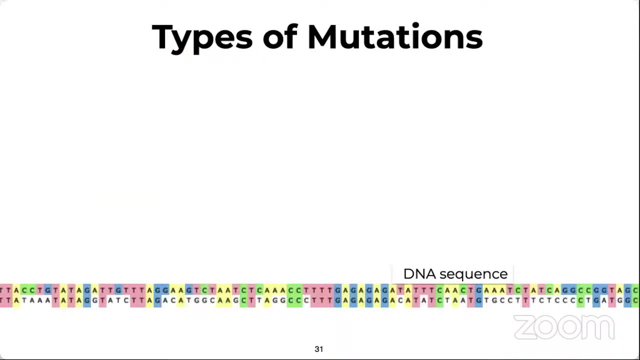 All the changes to a certain level that it affects the quality of life of the person or people involved. So we spoke about different types of variants and mutations at the level of nucleotide. right Now we can actually characterize the same variants- and sorry variants and mutations at the level of amino acid. 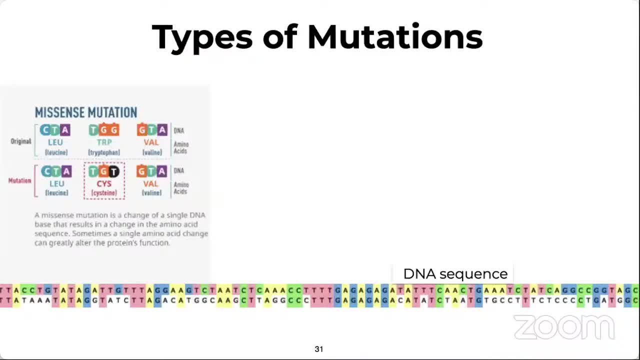 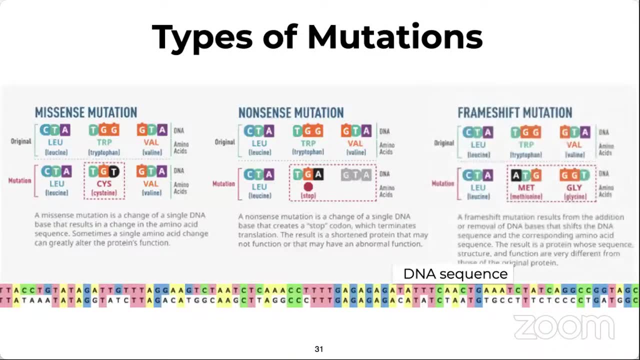 amino acid residue that the trinucleotide codon actually encodes. For example, we can have missense mutation, which refers to change in one DNA base pair that results in substitution of one amino acid for another in the protein made by this specific gene, For example in: 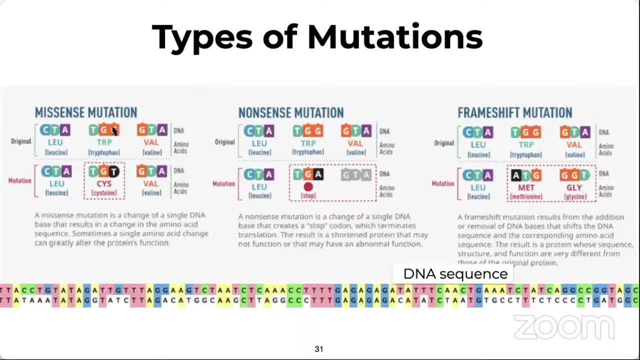 this case, one change in the nucleotide at the nucleotide level changes this one specific amino acid from tryptophan to cysteine. This is a missense mutation And some are actually termed as nonsense mutation where change in one nucleotide level prematurely stops the. 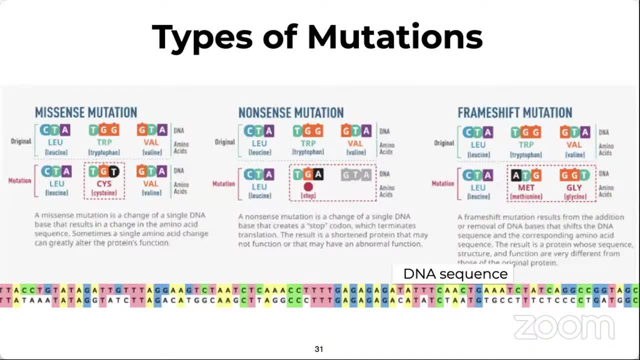 building up of protein, and this results in a shortened protein that may not function properly at all. right, There is also other kind of mutation Changes, like frame shift mutation, where insertion or deletion of DNA bases changes the entire reading frame of the codon themselves, So resulting in a protein that is completely 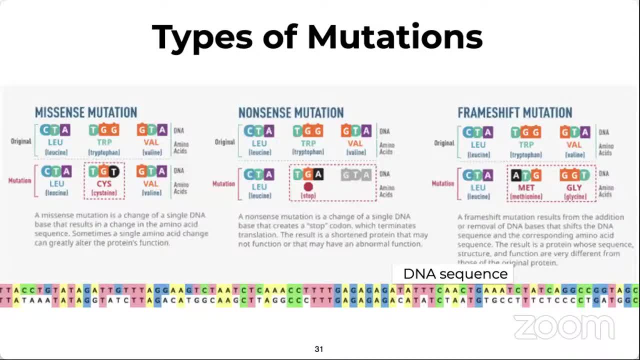 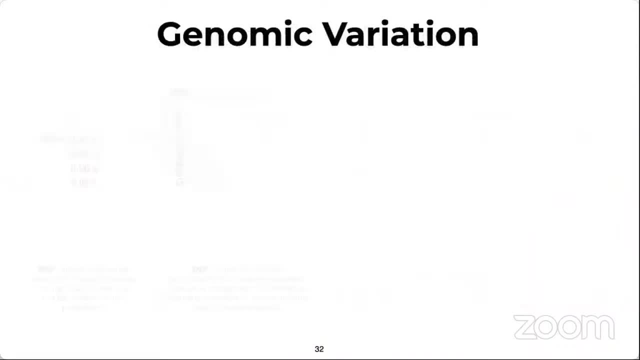 different from what it is supposed to be produced at the wild type level And most often these proteins are usually non functional. So, to summarize, we can summarize this as genomic variation can be of several different types In genomic data. we are looking to find and characterize the changes in the DNA code and 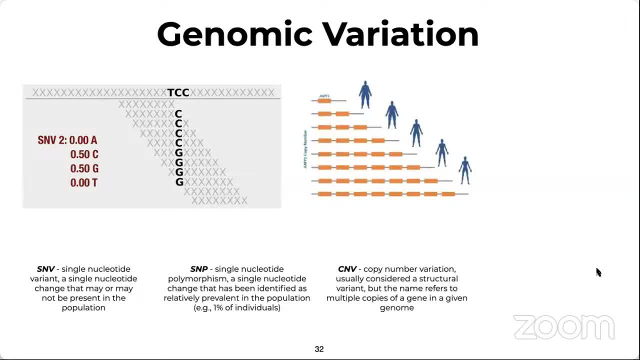 associate them with the phenotype of the organism. So some of the acronyms that we actually discussed and we should actually remember are SNPs and SNVs. right, And to reiterate, SNV are single nucleotide variant, a single nucleotide change that may or may not be present in the whole. 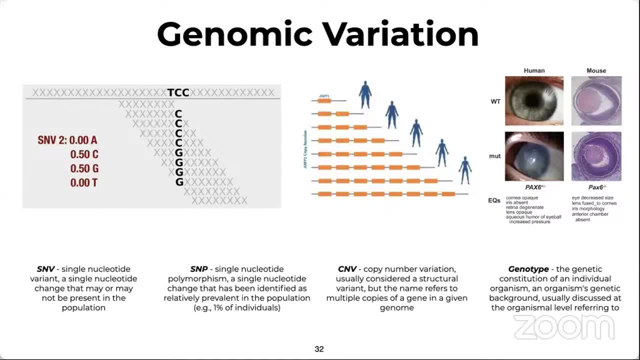 of the population. Basically this means any change from the reference genome found in the given DNA sequence above the level of technical error right. All the changes that we find in our sample data that differs from the reference sequence are termed or are categorized as single nucleotide variant, And single nucleotide polymorphism is when a nucleotide that is known. 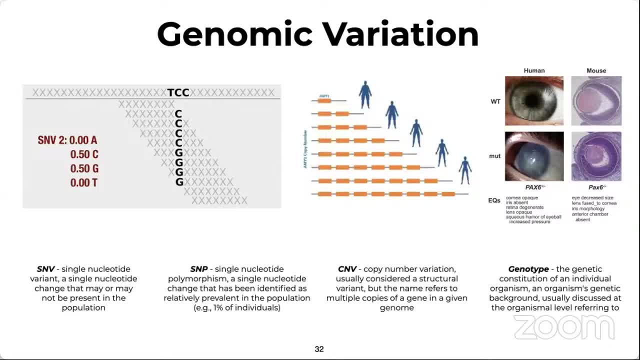 to be altered in a proportion of population. Typically, the proportion considered is approximately at the one percentage level of the population, And there are also other other terminologies like copy number variation when a gene is encoded. multiple copies encoded in multiple. 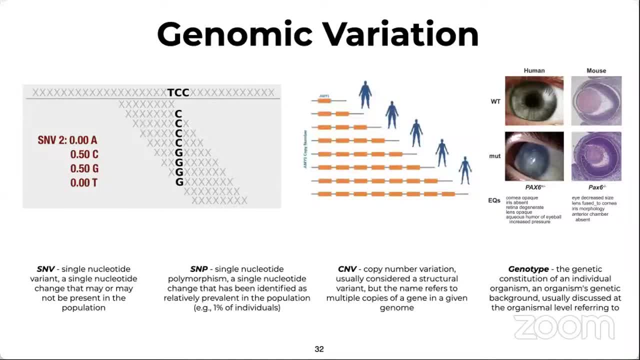 copies, and the number of copies varies between the reference genome and in the sample that we are analyzing. So these changes, as well as the characteristics of these variants that we are actually analyzing and identifying, are commonly referred to as the genotype of that specific organism. So, before moving on further, if you have any queries, please share. 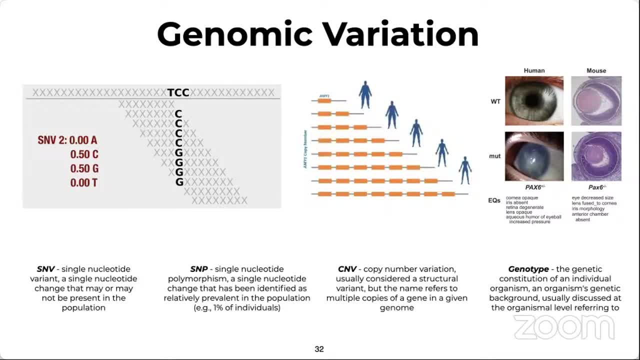 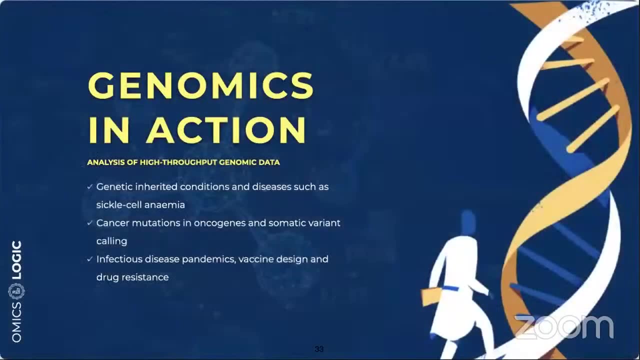 it with me. Okay, there is a general query about like to do about projects, about projects we will actually get to know at the end of the session And, yeah, about the genomic databases we actually discussed. So let's move ahead and see how is genomics or how supposedly are these variants. 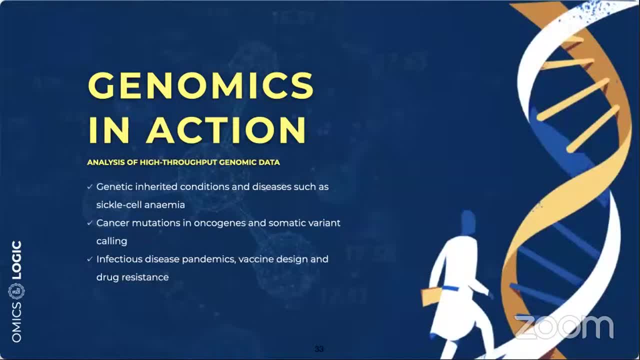 and understanding of these variants are used in real life To help us understand the impact of the genomic data. let's take a look at some of the genetically inherited conditions and diseases, such as cancer, mutations in oncogenes, oncogenes and sometimes like infectious. 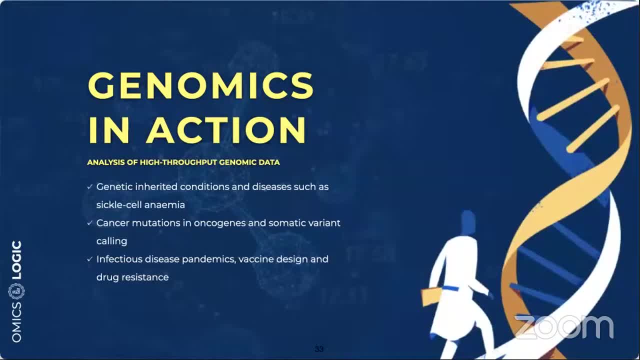 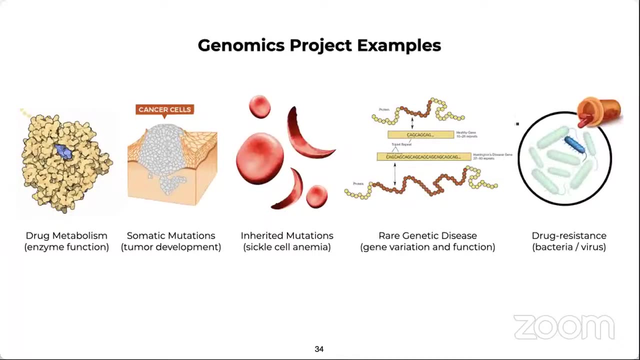 diseases and for which drug resistance is involved, and sometimes like genetic, genetically inherited conditions, like sickle cell anemia and other cases. So most of the data that we are discussing here, or information that we're discussing here and several other examples of how genomics data analysis are used. So let's take a look at some of the genomic data. 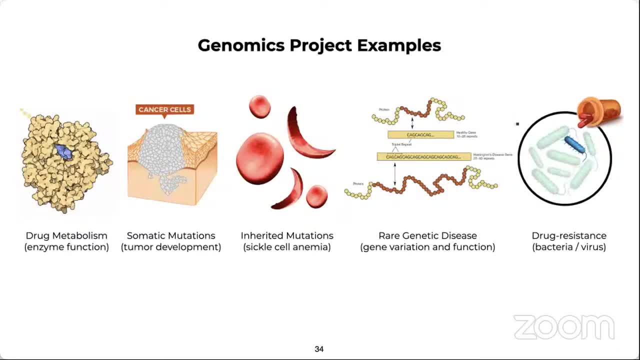 limitations. So let's reach into the genetic outbreak response based on Ner scent or disease possession and we have some studies that obviously show that bağ Ras and continue to happen. And again, just to give a general look at these and say any type of pathogen that we'll be analyzing. you'll see that these have particle metabolism, which is the debuted levels. that stack is an medal level and they all have the Afterwardskennt exposed to the mass pH values. So if you can go back to that dataorer that we talked about earlier, if 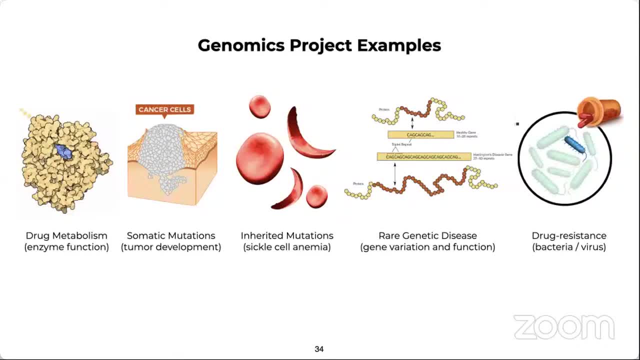 or sometimes understanding the rare single-nutrient variants that are involved in changes in the structure and function level of some critically involved protein, and also some of the variants that are known to develop drug resistance in the pathogen at the pathogen level, not at the host interaction level. 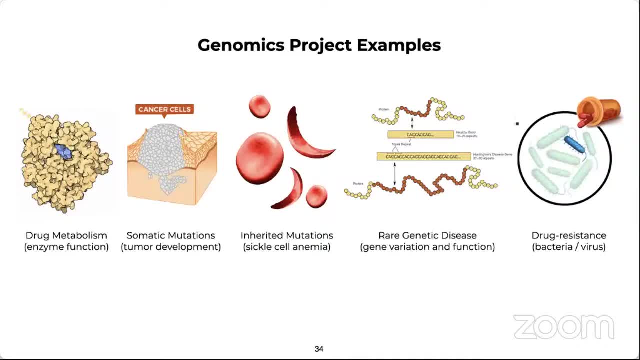 Some of the known pathogens, like Mycobacterium tuberculosis and even sometimes some Sars variants, are known to develop drug resistance to very well known antibiotics and anti-antiviral drugs that we are actually using. So these are all some of the project examples that we will be dealing with the progression of the program. 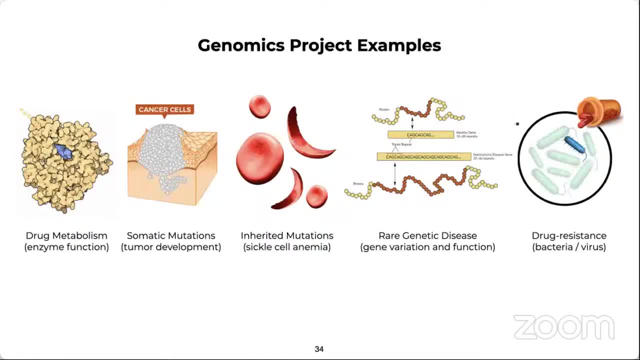 And you will learn a lot about how the data, or what kind of what type of data, is analyzed and what kind of data is used to do the work that we are doing. So these are all some of the project examples that we will be dealing with the progression of the program. 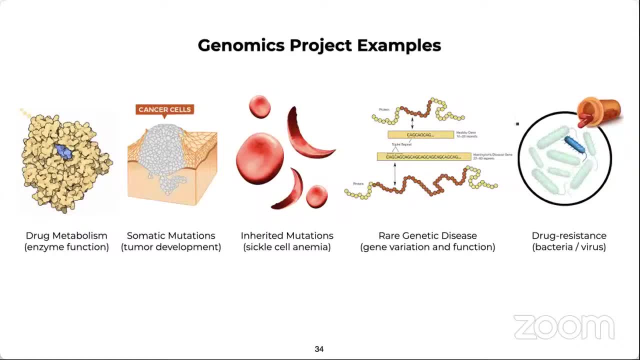 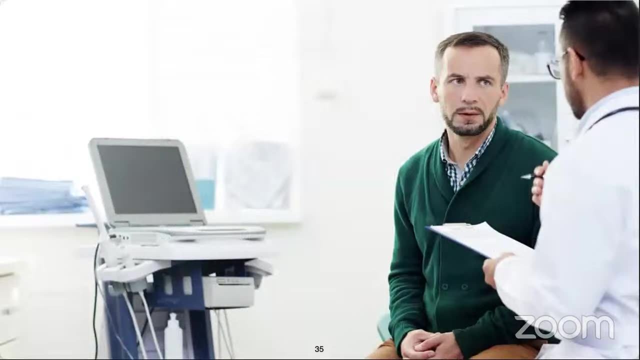 What is the analysis process and how are we actually using curated data set to understand this level of genetic variance and its association with the disease type? So, for example, to give you an example upon, a patient may be requested to go for DNA sequencing to help with the prognosis and diagnosis of the disease. 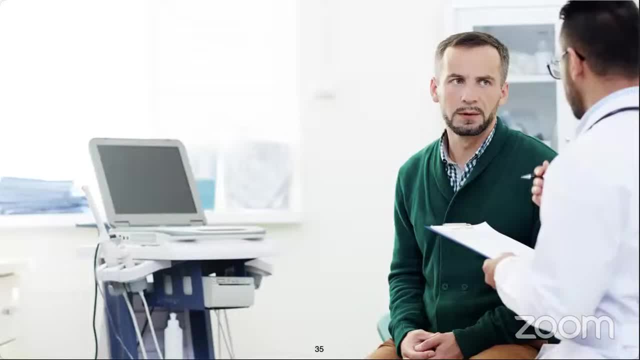 So, upon receiving this sequencing results for any sick patient, the first question we usually ask- or the first question is that is usually addressed- is what are the genes that are affected? So this is not a very simple question to ask, while genomics is already used for currently. 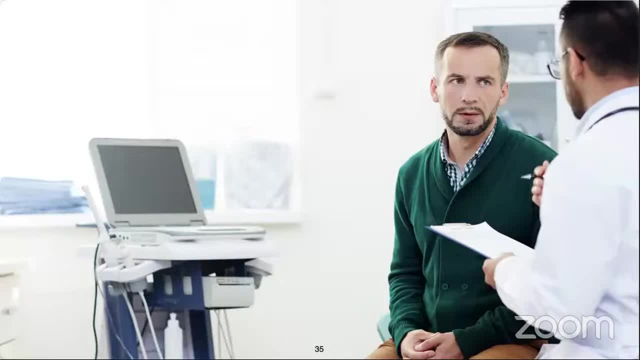 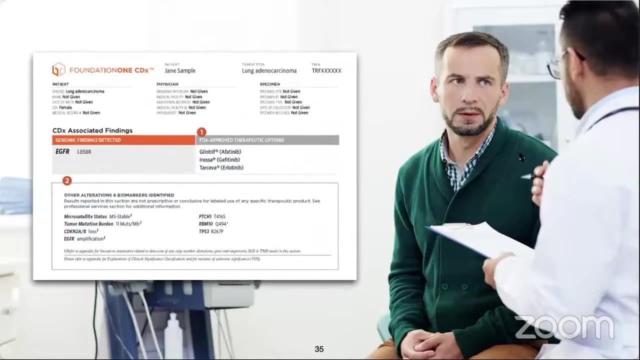 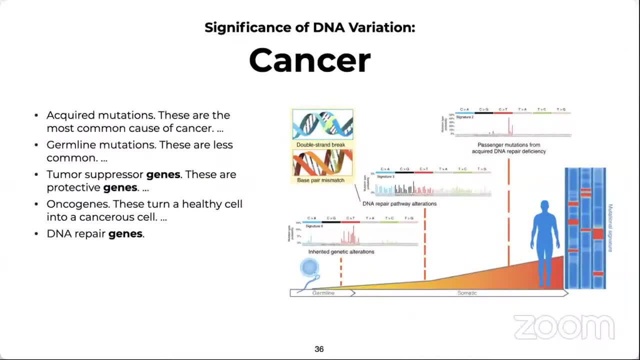 all over the world. So, for example, in the association of cancer, the DNA variation can help determine the genetic risk associated with oncogenes. right, But most often oncologists look for somatic mutation in tumor suppressor genes. So in oncogenes- sorry, in oncogenes or DNA repair genes, which are all very well known. 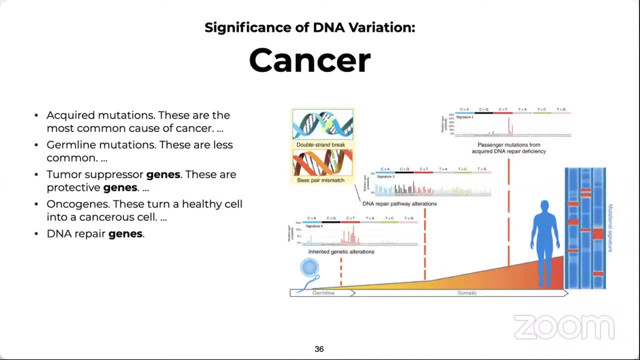 to be associated with the tumor progression. So, since cancer often, since cancer most often occurs with age, many researchers see or often notice this accumulation of somatic mutation in key genomic regions as a combination of driver mutation which can be associated to the progression of tumor, and passenger mutation. 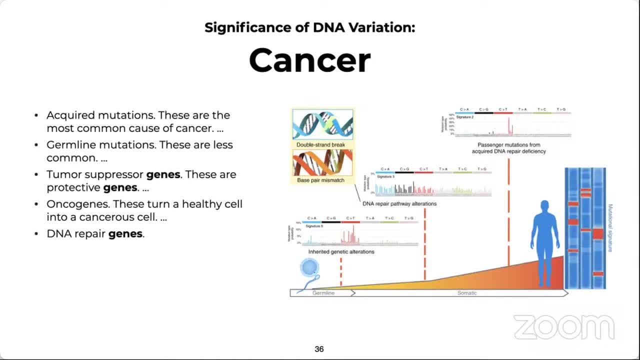 which can be associated to the result of this tumor progression at the genomic level. This can actually help us diagnose the cancer early on. It can actually help us evaluate the risk of the cancer severity. It can actually help us look for appropriate treatment to slow down this cancer progression. 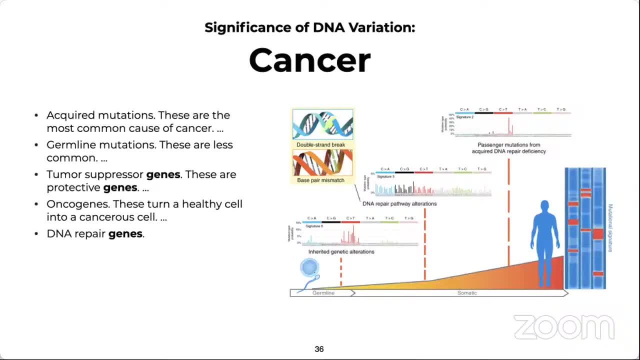 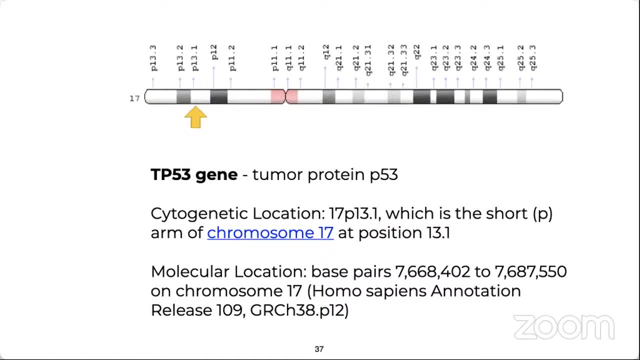 and help us deal with this incurable metastatic cancer. So one particular gene of interest is the tumor protein T53 or TP53.. This encodes for a protein that is responsible for tumor suppression. Generally, it is present in all the cells. 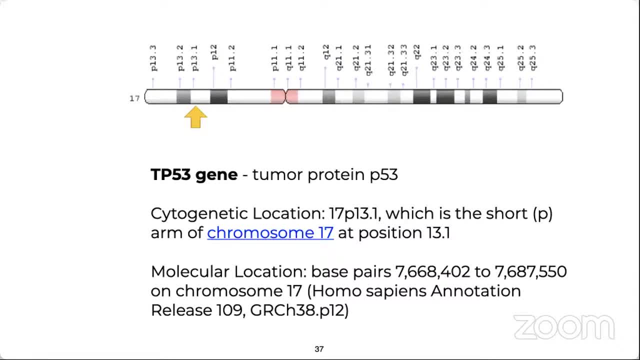 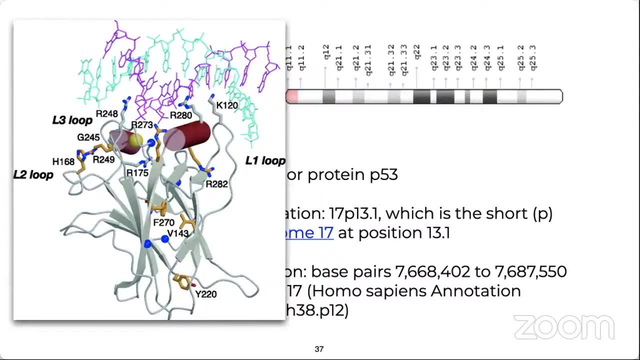 It is implicated in many cancer and it helps prevent tumor growth through the process called apoptosis. Some or several mutation in these genes can lead to loss of function and ultimately promoting tumorigenesis by not controlling tumor growth, Controlling the replication of the cells that harbors abnormal growth with damaged 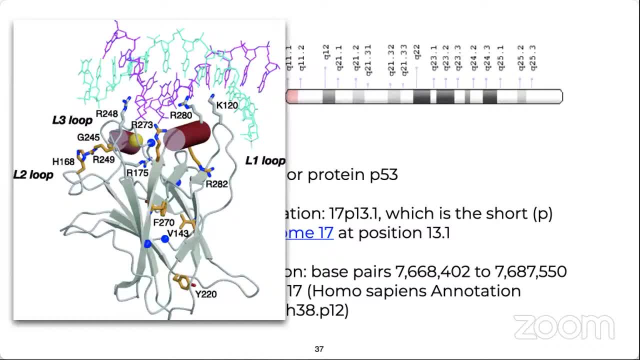 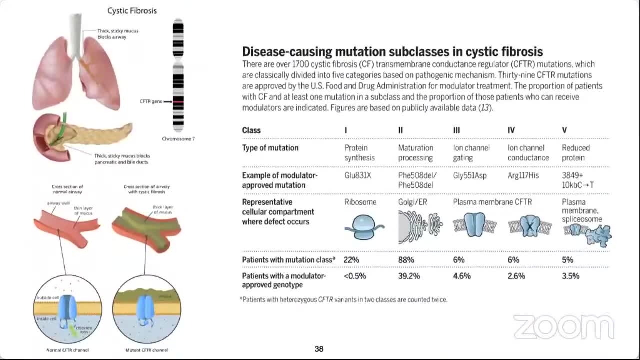 DNA. So this is one of the very well-known gene that is associated with the tumor progression and that we will also discuss in a short time. Other diseases, like cystic fibrosis can also be linked to individual genes, like CFTR gene, which can affect the function of the channel that is responsible for clearing mucus from. 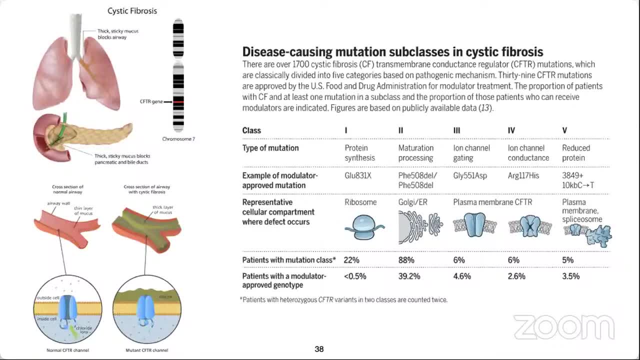 ARBs. This is an example. This is an example of diseases that is caused by genetically inherited mutation. These mutations are inherited genetically and identifying such variants and such mutations can actually help in dealing with some really deadly diseases like cystic fibrosis in this. 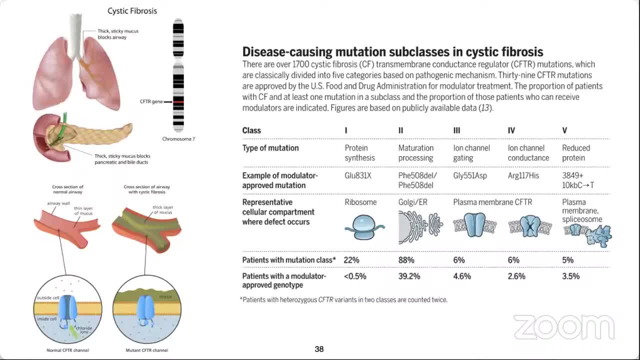 level, For example, people or person that is harboring Having this specific variant or mutation to CFTR gene, can be suggested to some suggested to treatment options that targets this specific channel to open up for clearing the mucus level at the for the patients who are suffering from cystic fibrosis. 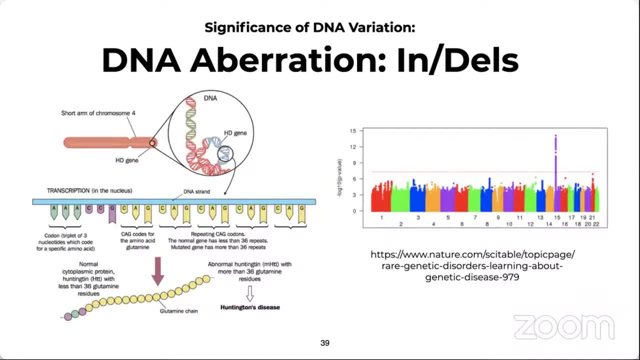 So and in generally also Some more Significant DNA variation, where the variation is now focused on, not on not the single nucleotide variant level or collection of mutation level. It is now focused on abnormal number of copies that is present in one specific present for 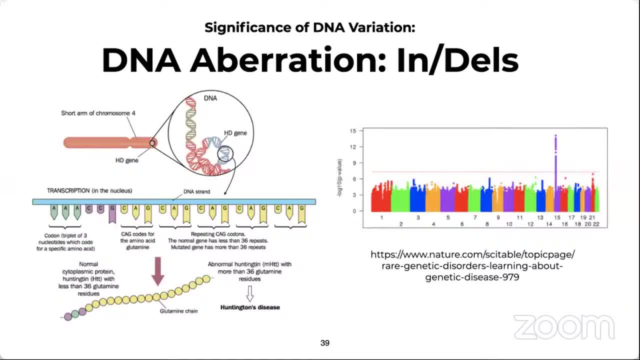 one specific gene in specific chromosome for. So in this case We are actually dealing with Huntington. This is where the HTTG, which is associated with the Huntington's disease, encodes a large number large protein- Huntington protein- and- and the aberration that is caused is the multiple. 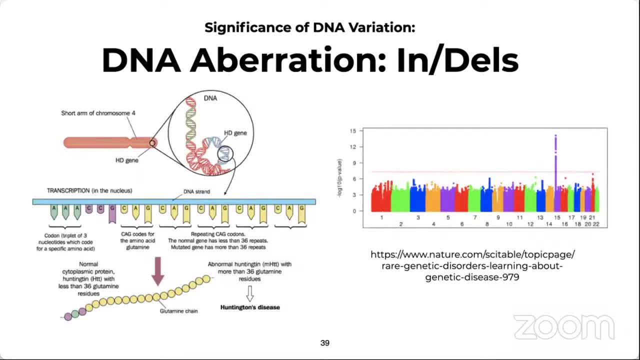 insertion and deletions, of multiple insertion and deletions at the at this specific nucleotide level, which results in abnormally long Huntington's disease, And Huntington protein, and hence the Huntington disease, actually results in this. several of this information is actually available to us due to the efforts of researchers and 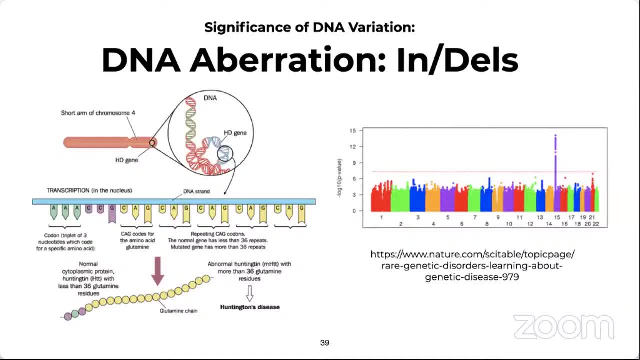 the private and publicly funded consortium which publishes studies on several individuals with these diseases and in this specific case, the Huntington's consortium actually published a study of over 1000 individuals with early and late. This is a study of over 1000 individuals. 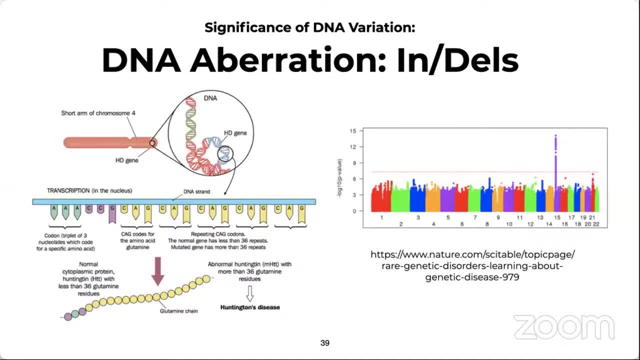 So we can actually estimate the onset of this disease and By by actually applying targeted sequencing and as well as whole genome sequencing and this treasure trove of data is actually used by multiple were used at multiple levels, to understand that this is and in generally understand the level of DNA aberration and 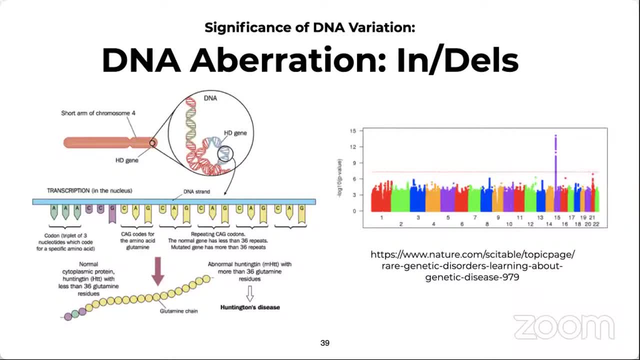 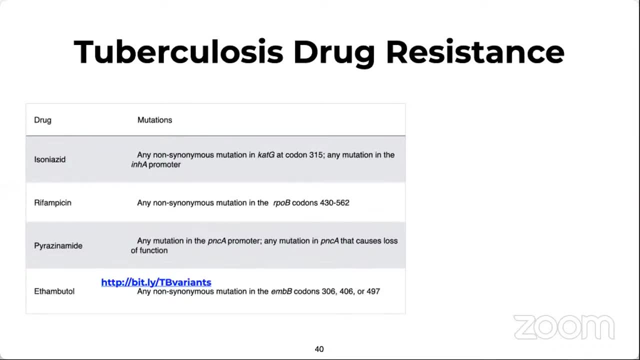 their involvement in The pathogenic effects of these DNA Right. So, as I mentioned, these Changes, changes in the DNA or changes in the genomics level and their characterization, should not stop at the human level, where we are mostly dealing with responses to these response. sometimes we 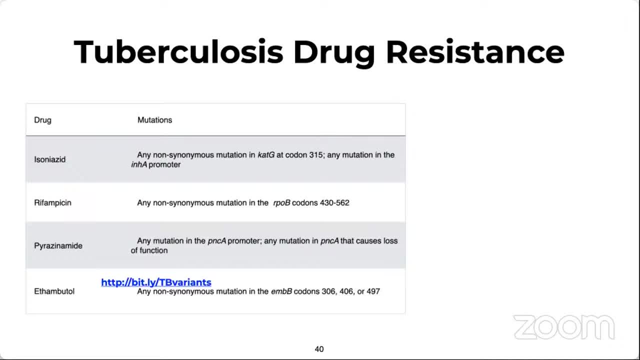 could be dealing with responses to externally activated stress factors, like infection in that, or causes due to external factors, like stimulus due to pollution and other criteria, or abnormal indigestion and several other situations. So in this specific case, for infectious diseases, we can actually use the same approach of studying variants, but not in the 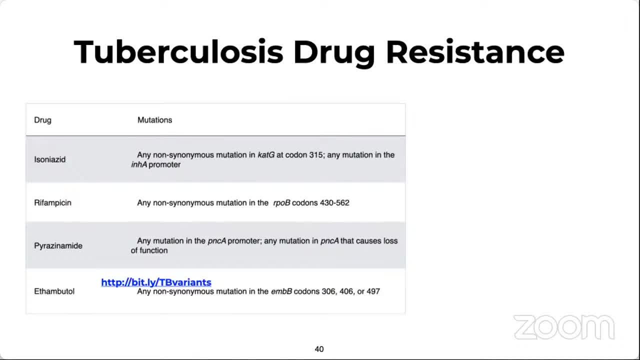 organism, not at the human level, where microbacterium tuberculosis accidentally occurs- actually causes severe diseases. right, We can study the genomic sequence of the pathogen and understand what these variations in the pathogens genome actually refers to in terms of understanding the characteristics of the pathogen for increased virulence. 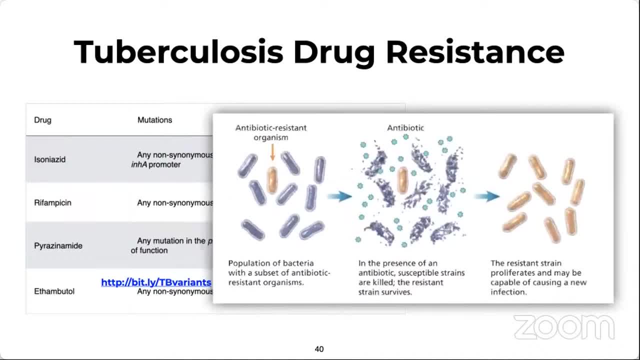 or increased resistance to specific drugs. right, So to give you some sort of a relation and understanding. right, In 20th century alone, tuberculosis was the leading cause of death in the United States. only right. And today most of the cases are cured with specific. 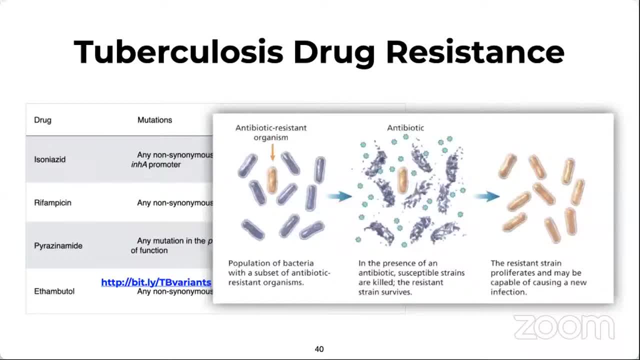 or special regimen of antibiotic treatment that can stretch over several months. However, recently we have come to know that this bacteria has become more and more resistant to several or single type of antibiotics. So it turns out that the bacteria turns out that the resistance, or this resistance, 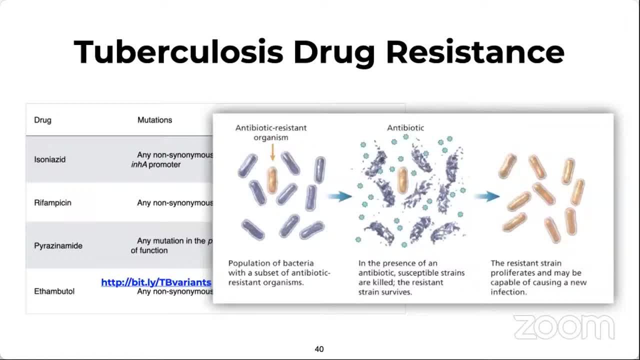 is the result of one or multiple mutations in specific genes are sometimes in the promoter that are preceding these genes. right Understanding which gene and at what position these variants actually are characterized and categorized to different drug resistance level will actually help us design a very efficient ways. 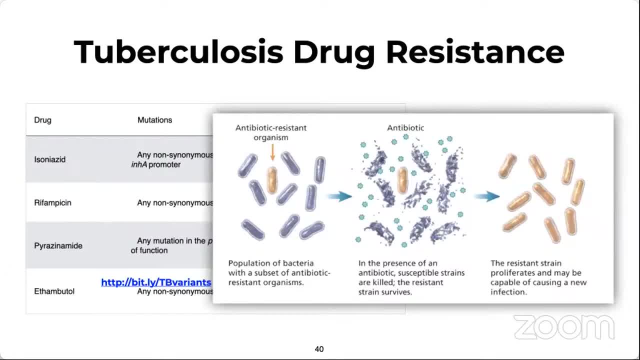 and efficient antibiotics And develop new drugs to address the surge of multi-drug resistant tuberculosis infection. And there is also another level of this drug resistance, which is called as extensively drug resistant tuberculosis, which simply is drug resistant to any type of antibiotic and any type of preventive measures. 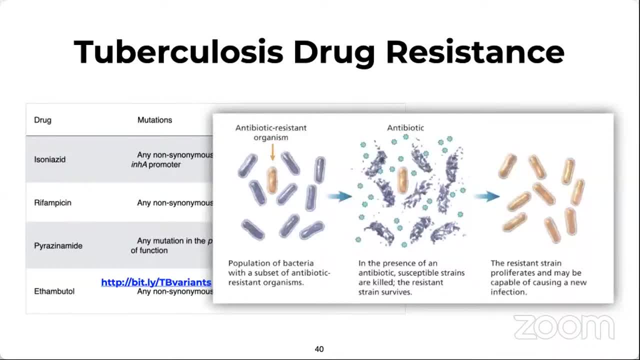 So such resistant levels of pathogen? the resistant pathogens are actually arising from the changes or random changes in the at the DNA level Or at the genomic level which suddenly could be beneficial to the pathogen, And very well known case of this is in the viral genome. 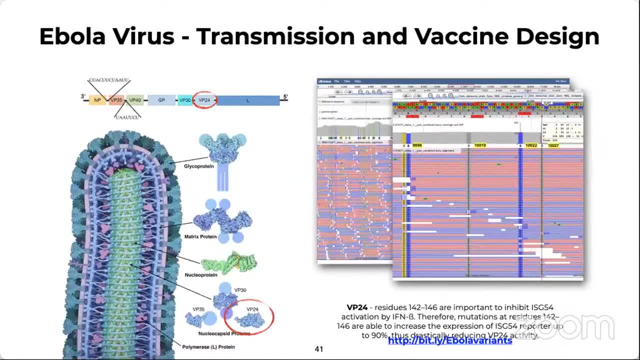 And here we have an example of Ebola virus where changes at one specific protein or one specific glycoprotein increase the transmission and virulence of this Ebola virus. But we are actually witnessing the same level of changes and variants and variants of concern, variants of interest in the SARS COVID pandemic. 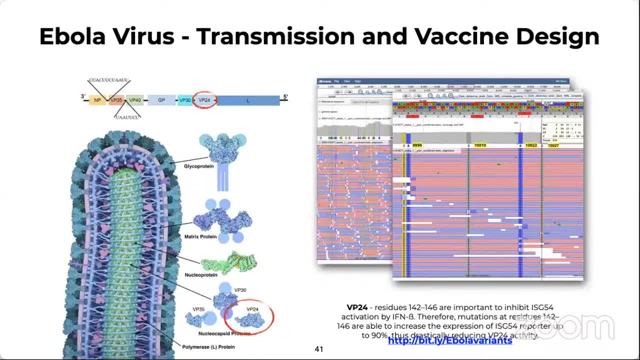 that we are currently facing. right now, All of these changes at the genomic level can actually result in the changed characteristics of transmission or virulence for this viral, for this virus in specific virus specifically, And only some of them could be beneficial to the virus. 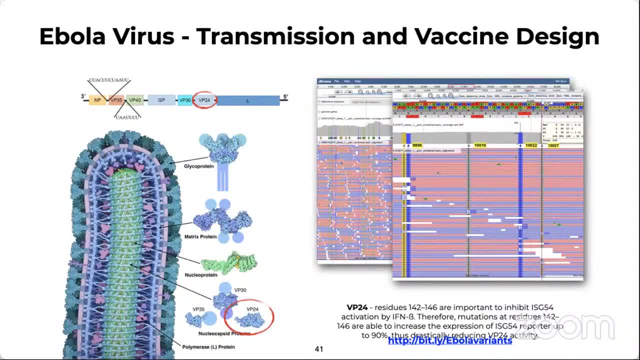 but most of them could be detrimental to the virus, Since virus actually replicates at an accelerated rate, so we have a larger population of these, of these virus, which eventually ends up ends up with the increased transmission rate or increased virulence rate. 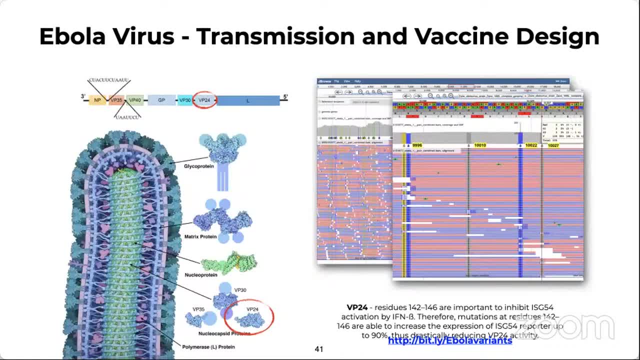 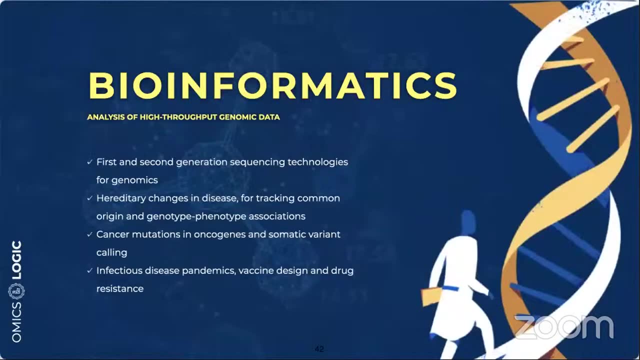 And hence hence the birth of new and novel and and strains and variants of concerns and variants of interest, as we have been witnessing in the last two years. So, before going to how to practically get this information from the sequence of genome or sequence of DNA in the genome, 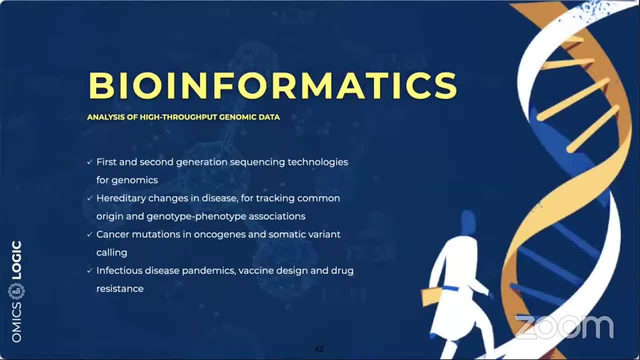 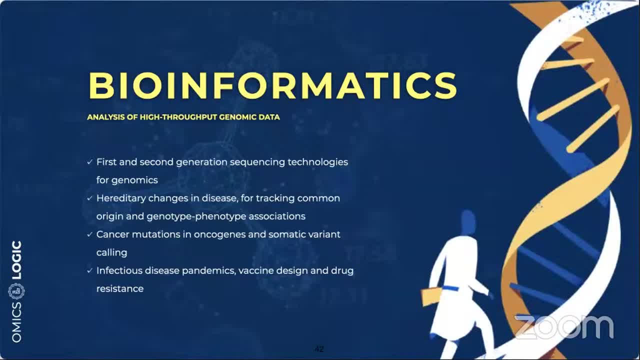 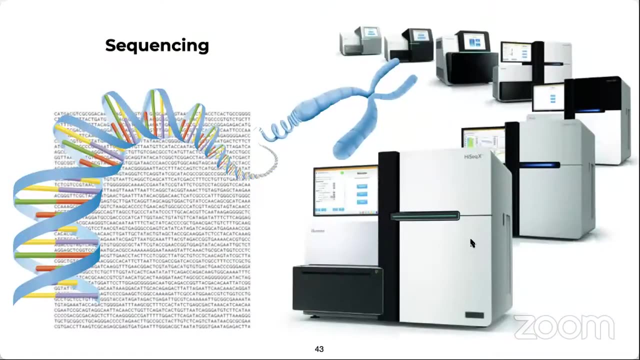 from the biological sample is called next-generation sequencing or high-throughput sequencing, or NGS. This technology, as we know, was first developed during the Human Genome Project and has evolved tremendously since then. So many different sequencing techniques were introduced over the years. 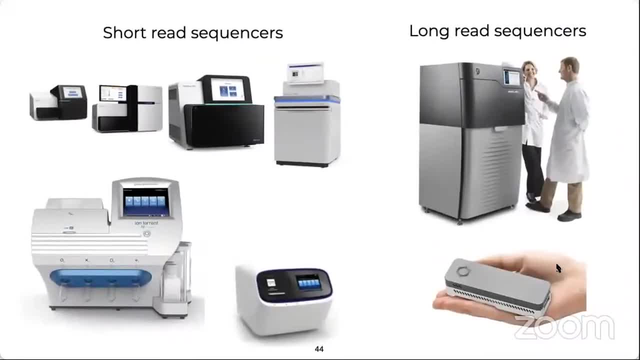 I'm not going to go over them. let's quickly go over them. So, in short, we have short-read sequences and long-read sequences, and each of them- short-read and long-read sequences- have their own place in understanding, understanding, understanding. 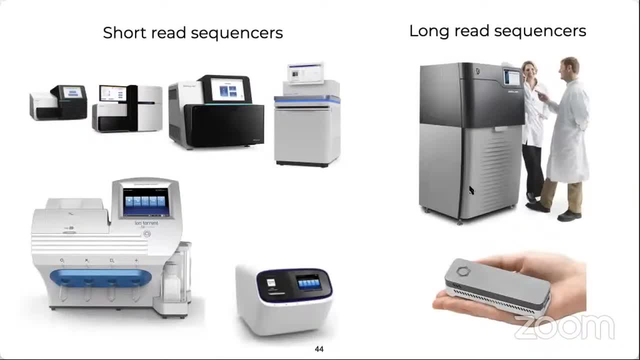 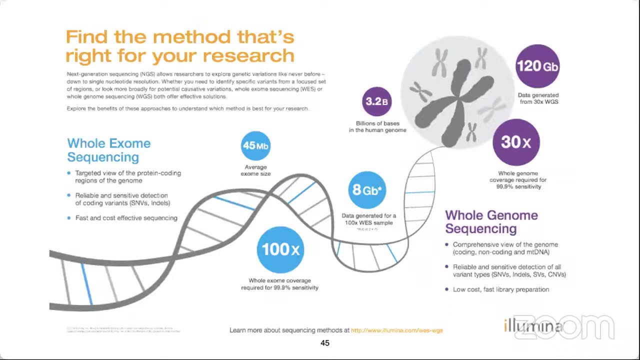 understanding the genomic variants at the DNA sequence level. So these different sequencing techniques actually, why are? why is it coming twice, I don't know? Okay, So actually we'll allow researchers like us to explore genetic variations like never before, down to a single nucleotide resolution. 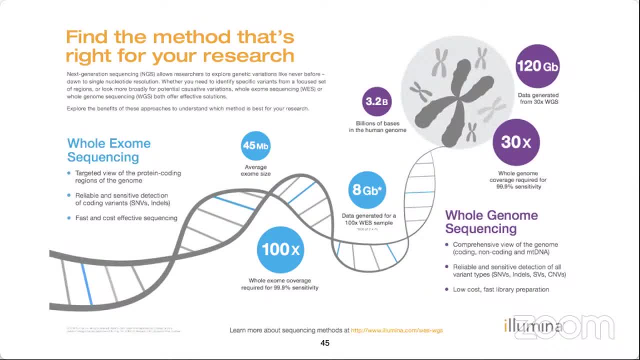 And these different techniques will actually help us explore the genomic variants at different resolutions solution, as we mentioned. So this could be at, for example, whole genome level, where we have- where is it? at whole genome level, where we have to sequence all of the DNA bases? 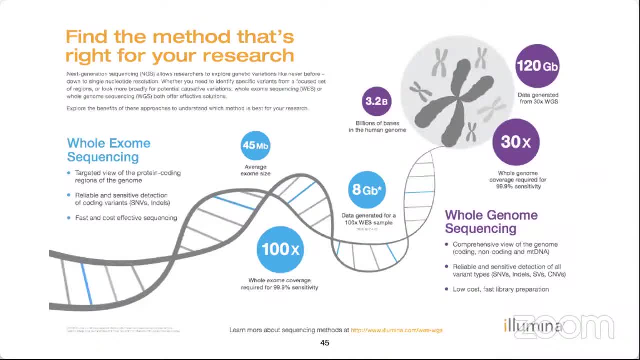 and since the amount of information that is generated is huge and that involves a lot of resources in terms of money, in terms of time, in terms of sample preparation, in terms of library preparation, and hence this is done at an average coverage of 30x, which 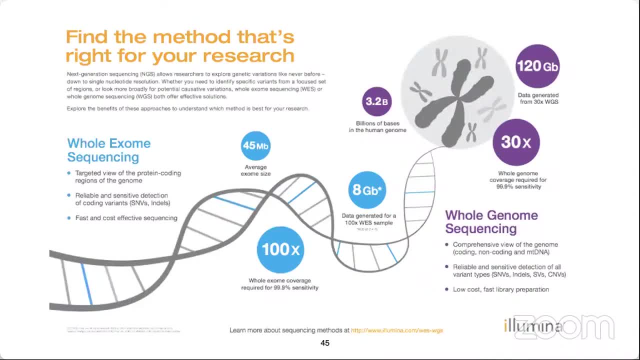 defines the number of times one specific DNA base is being read. So this is an average coverage of 30x. average of 30x to be sufficient enough to build a map of whole genome of the sample that we are interested in and get it compared to the reference genome to understand. 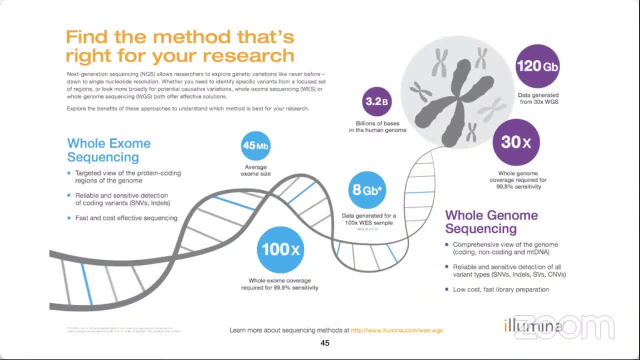 sequence variation of the whole genome level. We can actually not focus on all the genome. If we are interested only on the transcriptome or gene coding or protein coding part of the genome, we can cut down considerably on the amount of DNA sequences that are DNA bases. 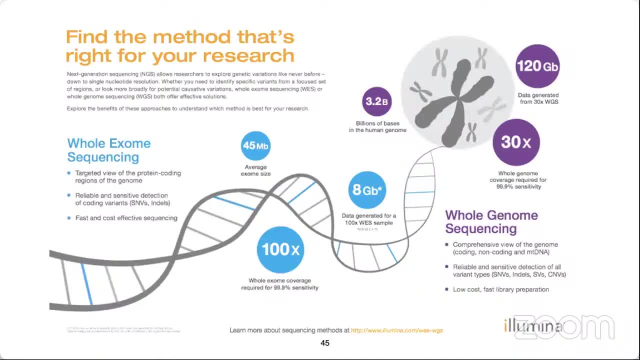 that are sequenced and hence those and hence the resources that are used to used to prepare libraries and sequence the DNA bases at the whole genome sequences can be used to focus, exome sequencing or only the protein coding regions of the genome, and such a level of 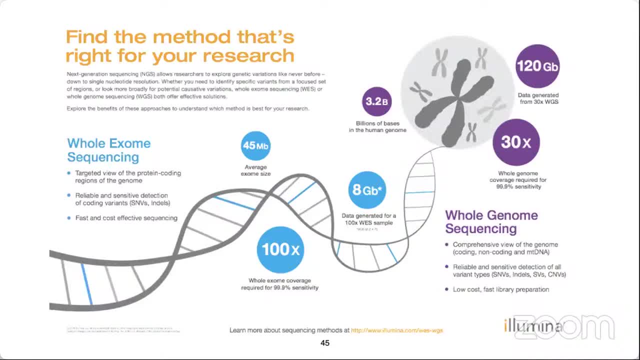 sequencing can be performed, or usually is performed, at a 100x coverage level, because our aim is to identify some of the rare variants that are present in the protein coding regions of the genome and which will help us associate this variants and mutations to disease type. 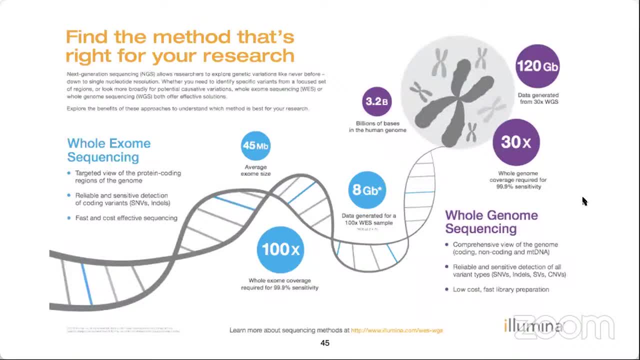 And we can also actually focus on targeted sequencing which will target specific regions of the gene, and that will again reduce the number of or amount of resources that we need to understand the genomic sequences. but there we have to have some sort of prior physiological or biological understanding about the regions that we are going to target. 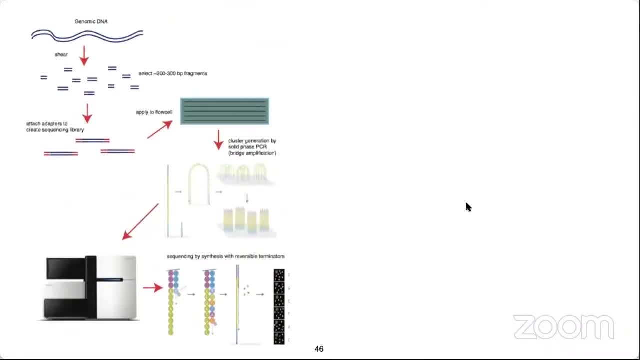 So how is this actually done? to give you a preview, or to give you a short introduction, right? The NGS technology captures the DNA sequences and generates the digital data using several steps. First, the RNA, or the genomic DNA in this case, is extracted from the cells and is then sheared. 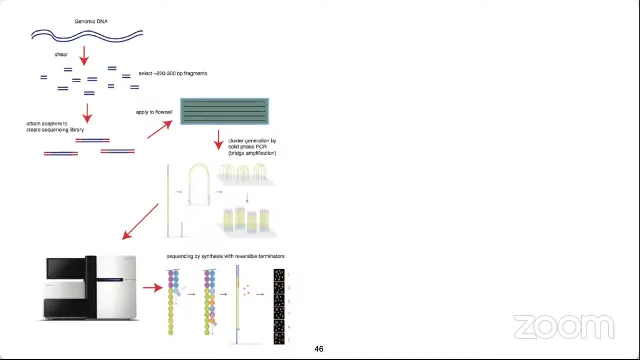 and is placed in the flow cell. and inside the flow cell, these fragments of sheared DNA are amplified using PCR amplification or bridge PCR amplification method. Then these amplified cDNA copies or fragments are then inserted into the sequencer and the machine uses a form of 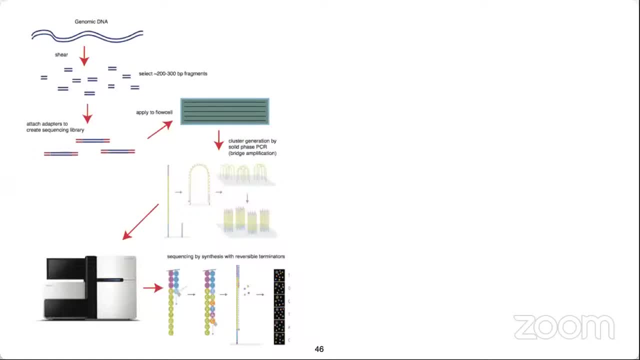 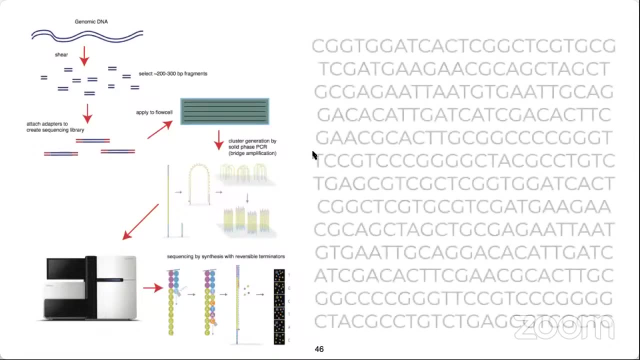 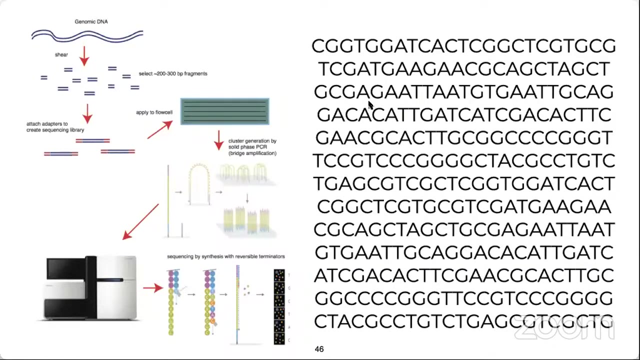 Image analysis to capture each and every letter in the flow cell fragments by analyzing visual patterns and converting them into the sequence of letters. So typically next generation sequencing reads are between 30 base pairs to 300 base pairs and they contain series of these DNA bases that are A, T, G and C. 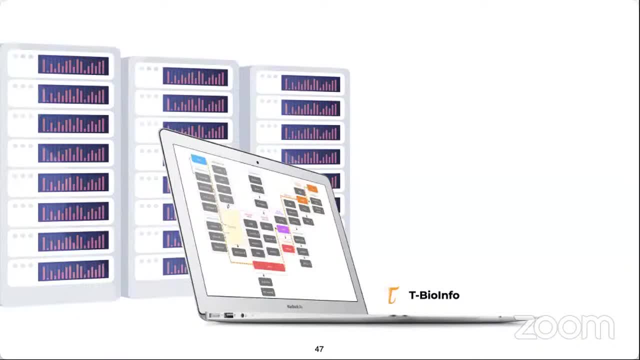 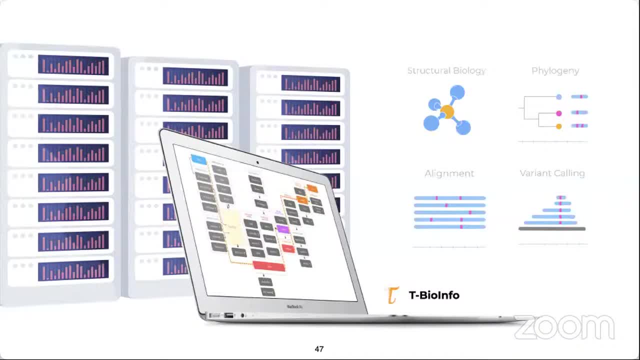 And there is a lot of work to be done, And there is a lot of work to be done. They include alignment of reads, and these include alignment of reads and analysis of relationships between the sequences and their evolutionary divergence, and the measurements of gene expressions and relationships between sequences and structures and identification. 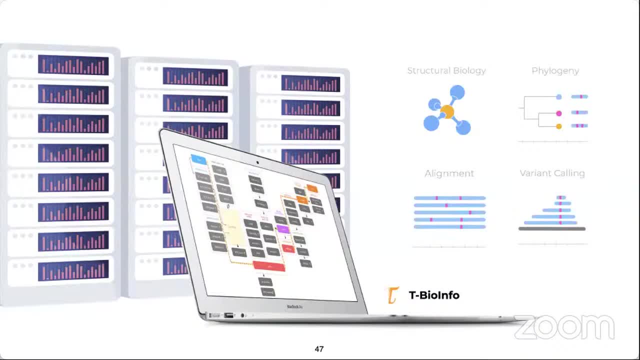 of somatic and germline variants And there are. these are different methods with which we can analyze this raw data, And the T-BioInfo server is an example. And the T-BioInfo server is an example of a platform or a big data platform that can 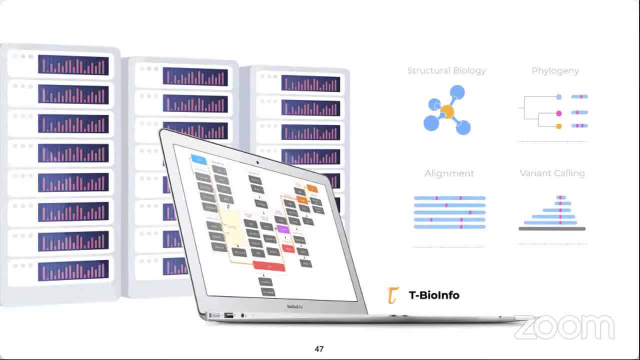 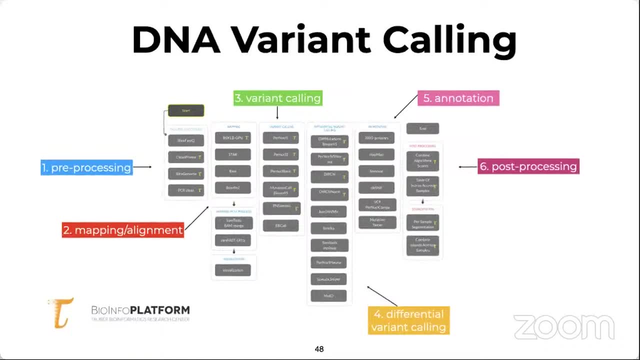 be used expertly to perform all types of these analysis and many others using an intuitive, user-friendly interface. Some of this we are going to have a look right now. So when this genomics data analysis is performed, it is usually performed with the FASTQ files. 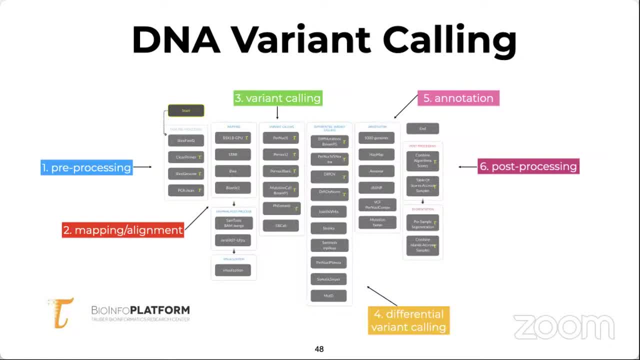 which are the output of the next generation sequence of machines. There are several important steps to be considered, such as pre-processing, mapping, mapping, variant calling, annotation of variances and post-processing of these variances to understand their impact by relating that to the phenotypical and biological state of this. 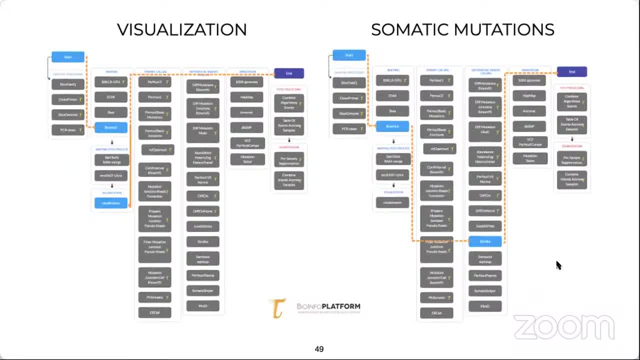 sample For each task. you can connect the analysis jobs into a pipeline and each one will have various inputs and outputs. Sometimes it is just enough to visualize the FASTQ file alignment to a reference genome to quickly get an understanding of major variants that are present in our data. 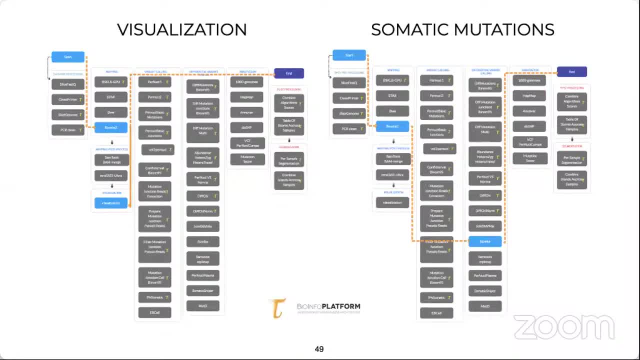 But for most of the time we might want to extend this to identification of these variants by statistically viable methods, so that we can perform downstream analysis with a lot of confidence and identify very well annotated mutations, like mutations that are associated with the disease state, like mutations that are associated with some altered phenotypical. 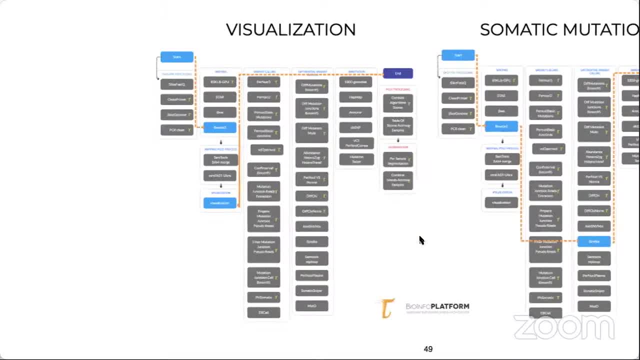 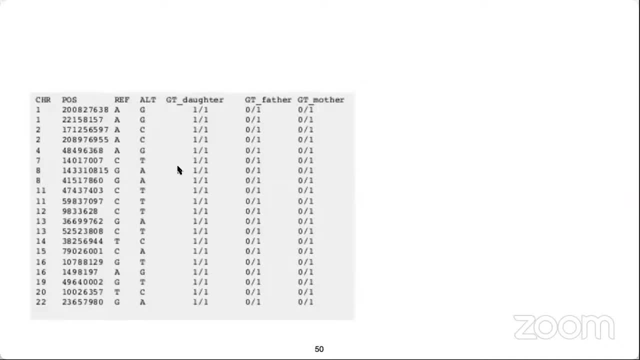 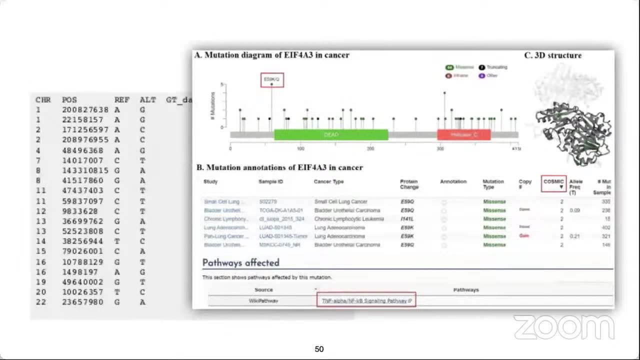 conditions of the virus, For example. the downstream analysis will actually find a list of mutations, a list of variants, and these can be represented and this can be displayed in a different, multiple, different ways, visualized in a multiple different ways. One can form at the basic level, we can annotate this as what type of mutation that they are. 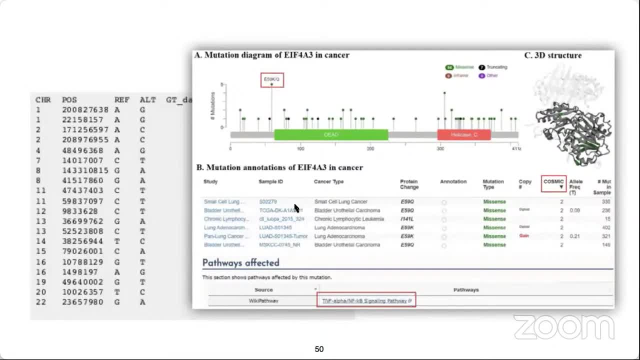 causing at the protein level. Or we can annotate this to what type of diseases that these variants are associated with. They can be tabulated. research can give you a lot of information regarding these individual variants. Or we can visualize these variants at the plot like this, which is called as Lollipop: 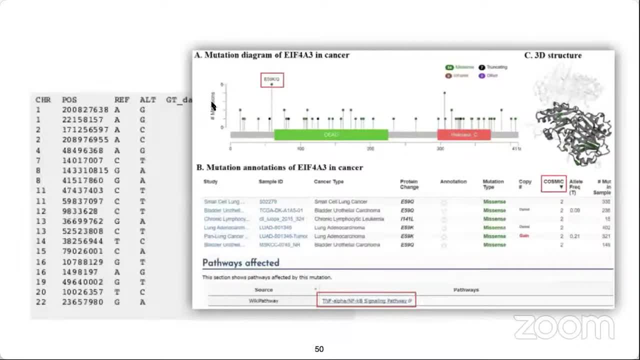 plot, where the length of the plot will directly refer to the number of variants that are present in our data, And we can also visualize their impact at the amino acid level. So this is a very interesting topic, Thank you, But more information is coming out in the in the days to come, very, very soon. 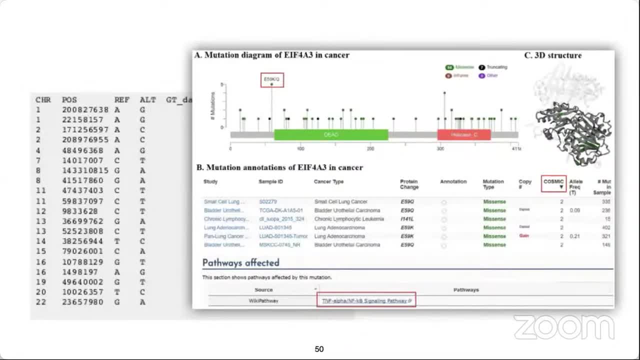 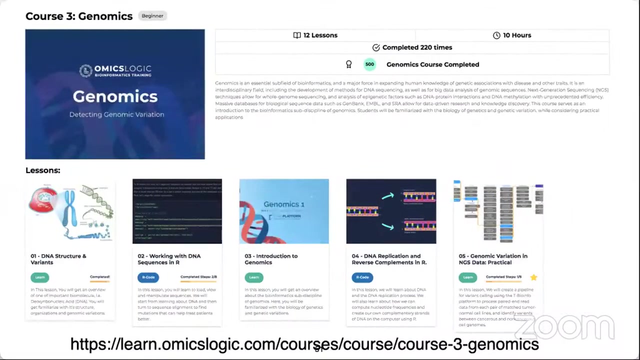 Thank you very much. Thank you Okay, Thank you very much. Okay, I think I don't know that that indicative of anything, Why it gets, by mapping their variants or variation onto the three dimensional structure of the protein, that that this gene actually encodes to an identify, whether the variation that. is observed at the three dimensional structure of the protein is concentrated at the functional part of the protein, or rather it is concentrated at the structural part of the protein. So this and several other related data can be related. information and steps to perform this analysis can be found in the genomics course, which we will list in the presentation. 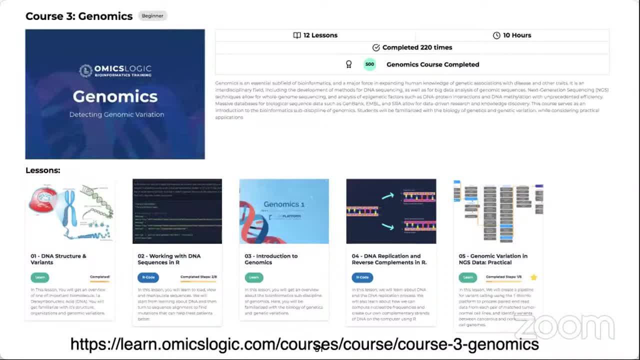 Thank you very much, Thank you very much, Thank you, Thank you, Thank you for your question, Thank you, Thank you very much. course which we will refer to and use extensively in the program and along with the several other publicly several other example project which uses publicly available data to perform. 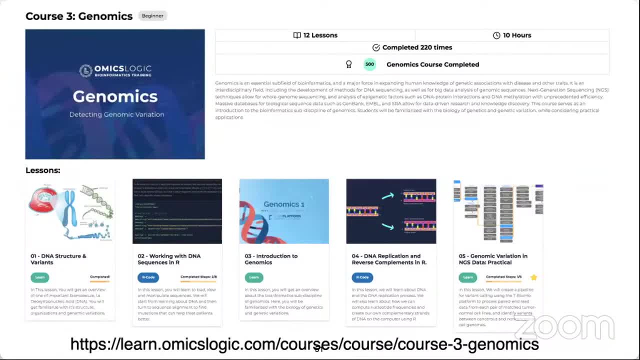 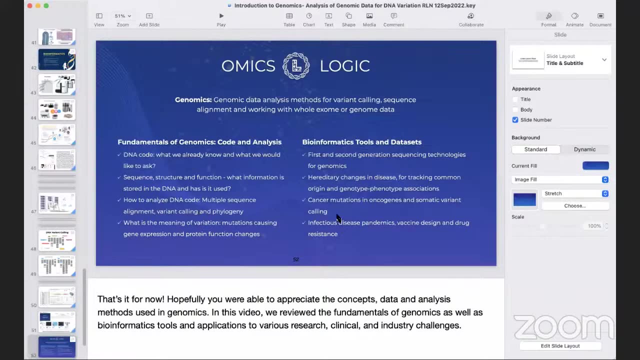 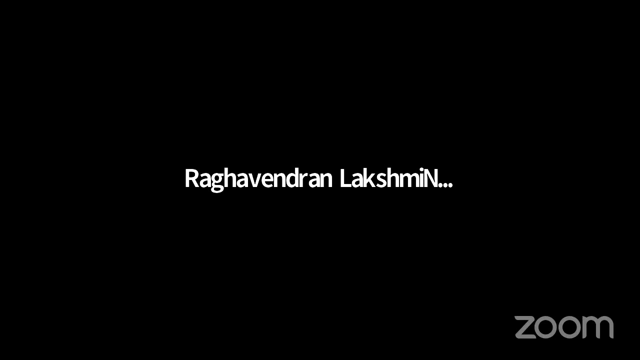 specific analysis types for different data to arrive at a special biologically implicated conclusion that we will discuss. So if you have no questions until now, I want to quickly reshare my screen to show you how these analysis can be performed and what we will be able to learn from these analysis. 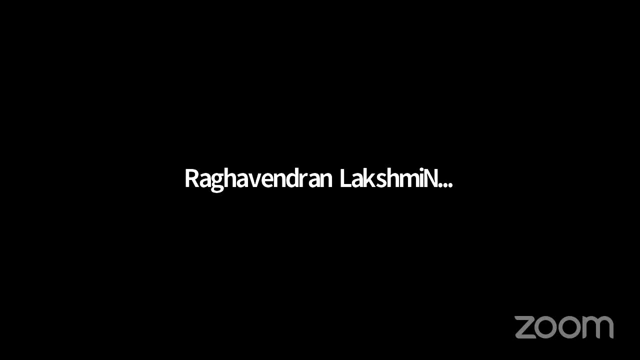 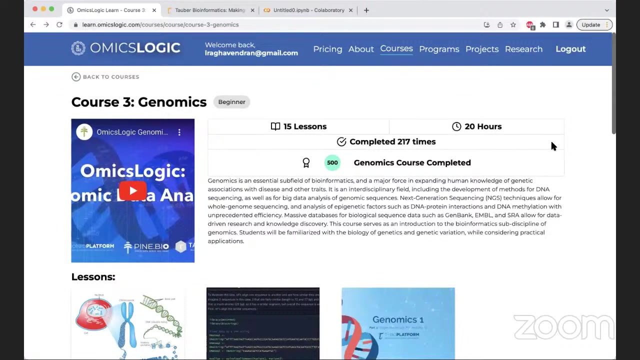 methods and let me find where is mine. is this okay? this is so. please confirm. you can see my screen and I have now opened course 3. The genomics course in the omics logic website. can you see my screen? yes, sir, it's okay. yeah. 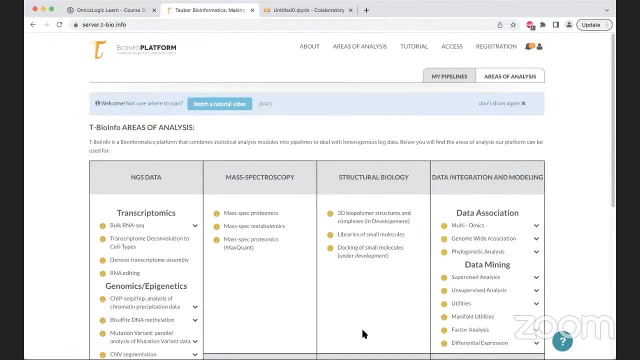 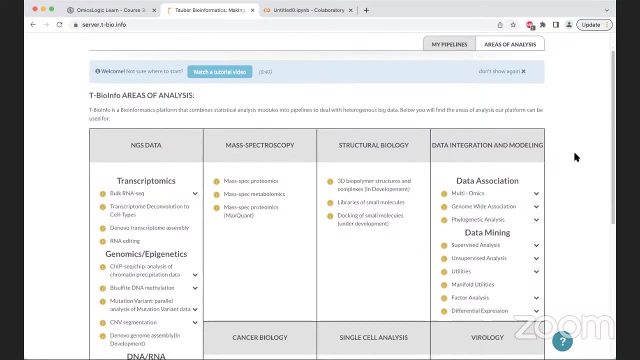 thank you very much. So this is the server- tbio info server- and those who have access to this server can actually follow along with me. or, if you want, if you prefer to watch what I am trying to do and trying to give get a sense of what can be done, you are free to do so. 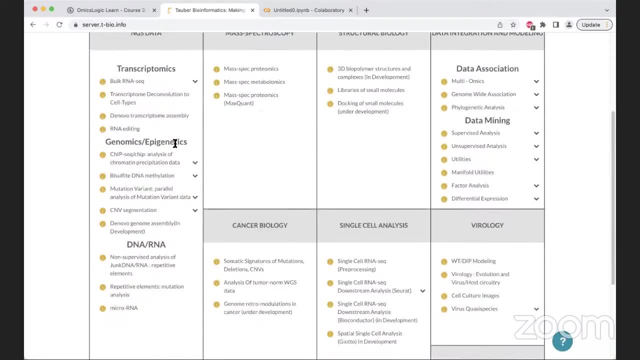 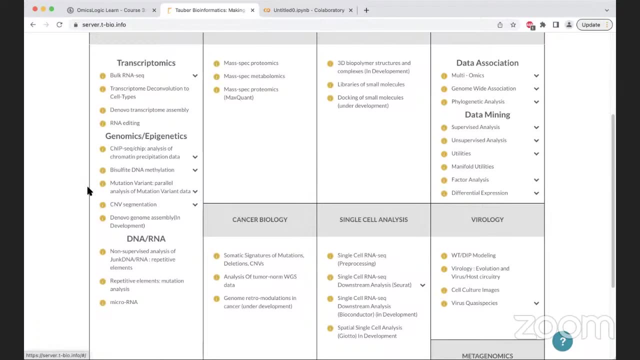 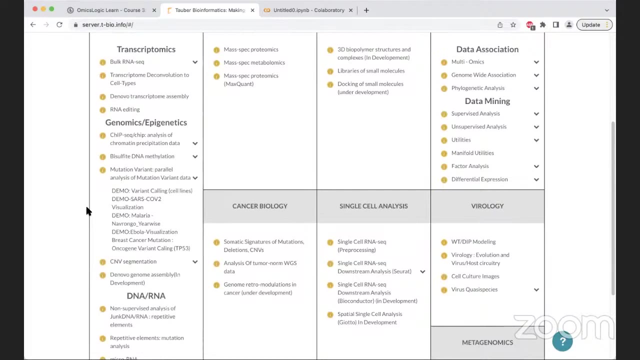 So in the server tbio info platform, under the genomics section, we are right now Discussing extensively about this mutation variant or analysis of mutation variant data. So if you drop down this option and there are several demo projects that are available which will give you the sense of building up of this pipeline with all the necessary 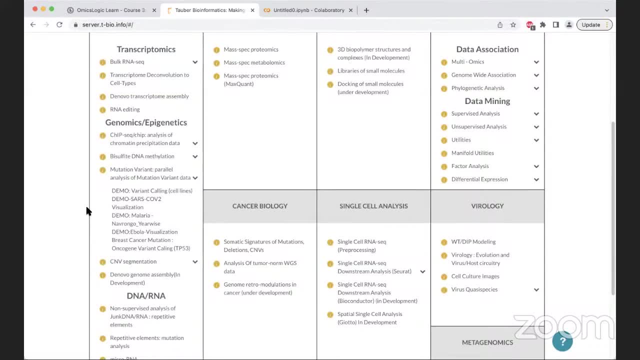 steps involved, or most of the necessary steps involved, and it will help you analyze the output file so that you can say, get a sense of what is being done and what we will get at the end of this analysis. So let's take one specific demo pipeline. 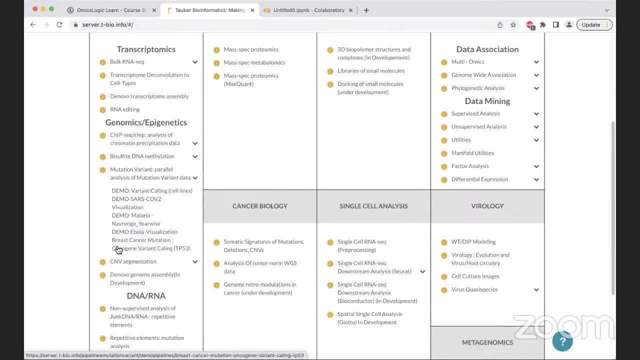 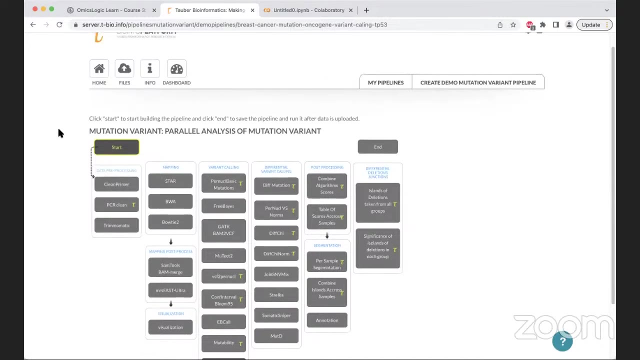 Okay, So this is a demo pipeline where we are trying to understand variants that are specific to the tp53 gene, and this data is a targeted sequencing data, and you will know what do you mean, what I mean by targeted sequencing data. you know why. So anybody who has credentials to access tbio info platform are actually will be, will actually. 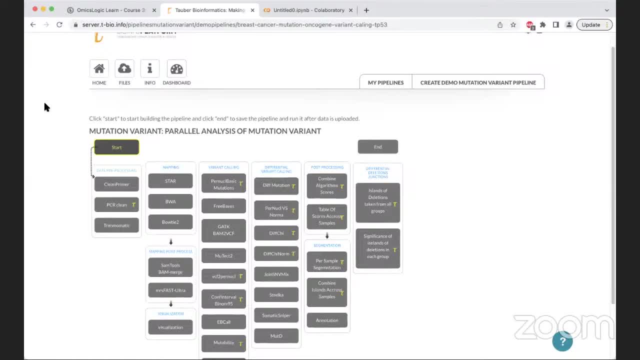 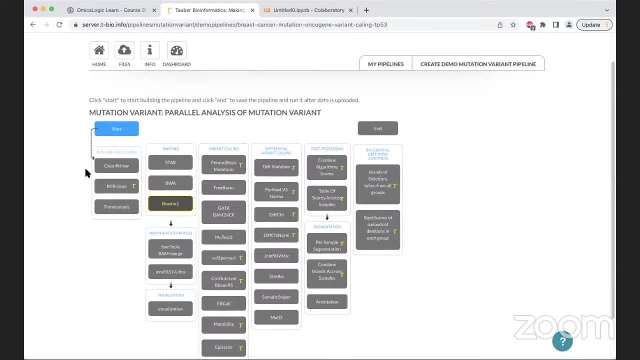 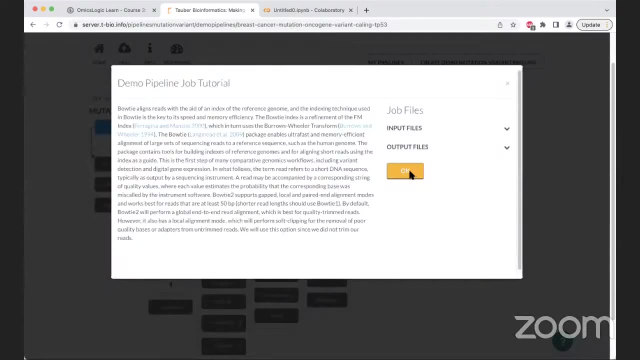 get access to this demo pipeline, irrespective of the subscription level that they are at. You are free to export, so let's start. so, while you are starting, we have actually uploaded the all necessary input files to you, so let's perform the analysis. observe that. the next 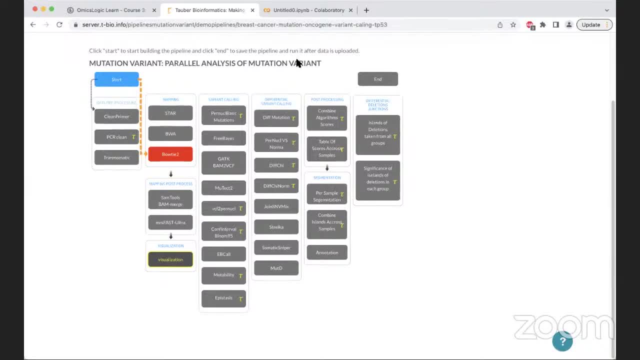 step or next possible steps are actually highlighted in this specific pipeline. we are actually using only these steps, but while in truth, when you are going to build a pipeline, at each and every step, the pipeline is going to give you all possible route that you are, you can take and you have to choose depending upon the type of analysis that you want to. 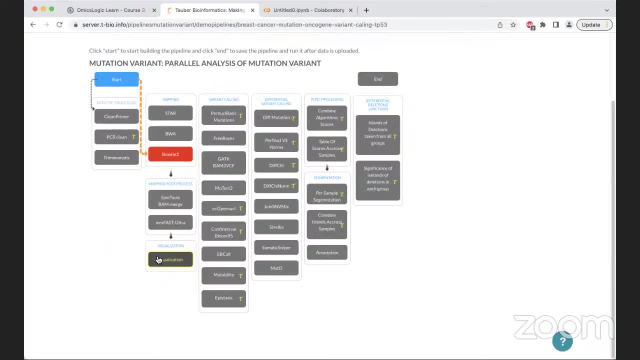 do and the type of question that you are asking in this specific pipeline. I'm just happy visualizing the variant that I have- oh, no, sorry for not I am. in addition to visualizing the mapping of FASTQ files or of the reads onto the reference, you know, I also want to identify the variants. 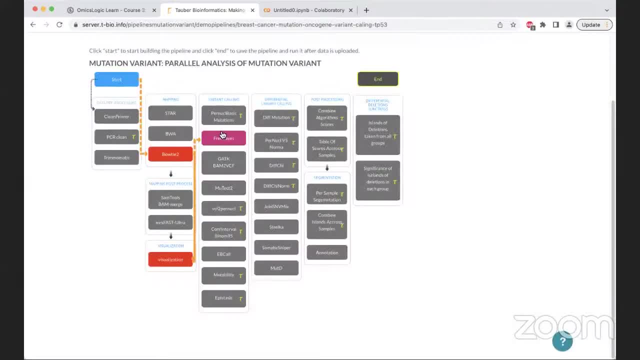 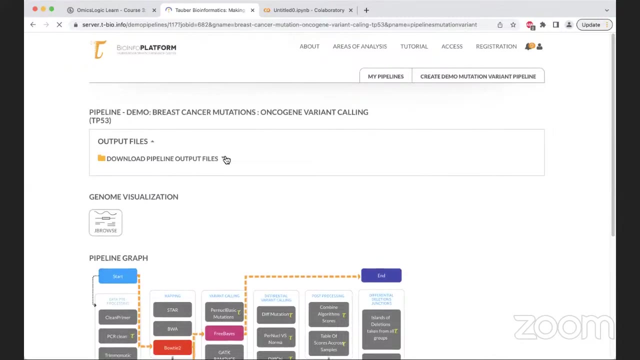 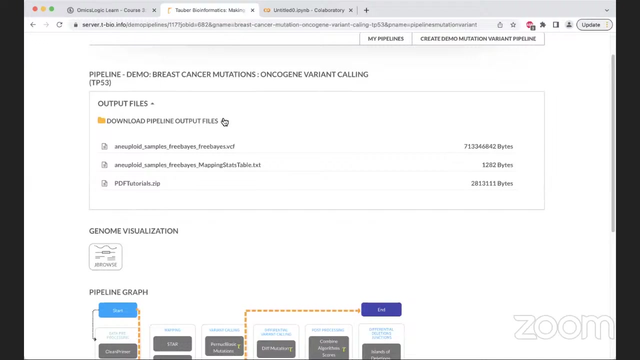 that are present in my data. so I include a variant calling algorithm or pipeline and this step into this pipeline and I am ending the date, ending the analysis pipeline right now. upon pressing n, you get access to all the output files. you are free to download this long or large vcf file and check what this vcf file generally will look like, right? 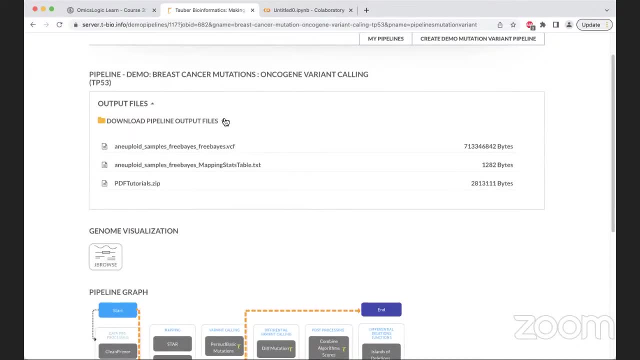 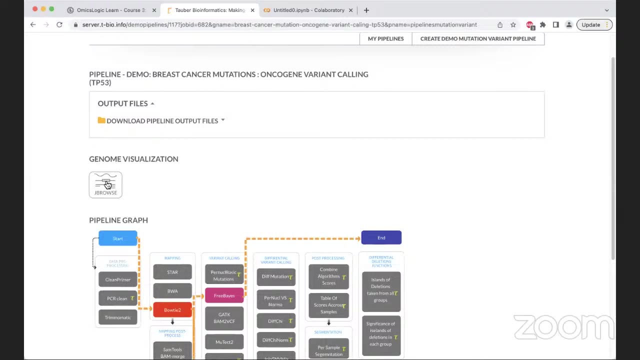 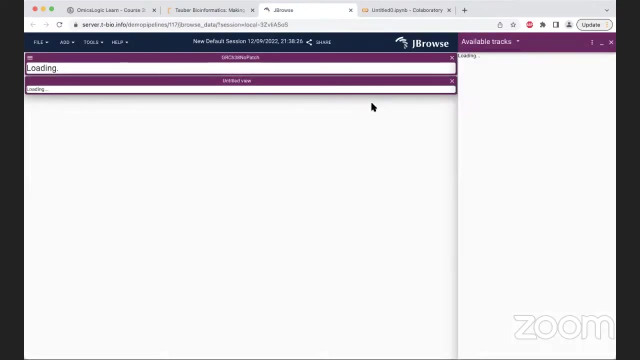 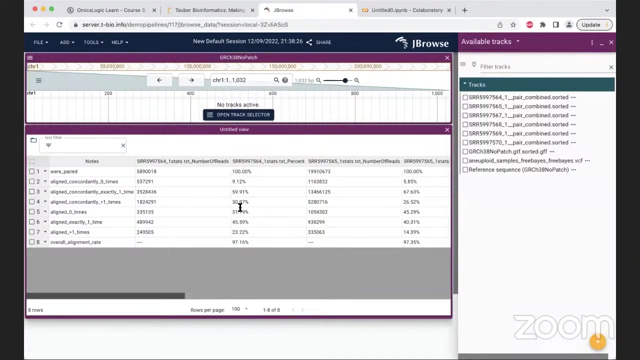 while the mapping stats table will tell you how good your mapping of the samples that you sequence to the reference and all of this. So all of these information are condensed into this genome visualization option, Which you can visualize intuitively. so when you open this, this actually loads up the mapping. 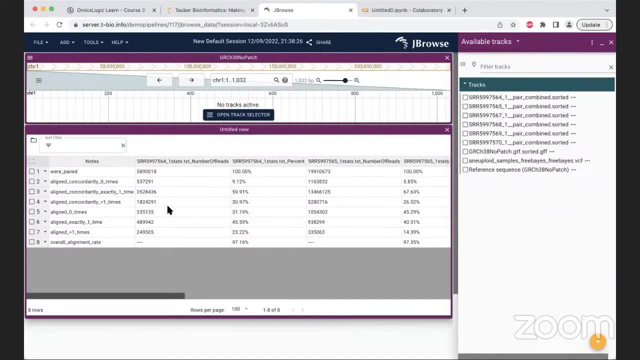 table or mapping stats table, and the first key statistic that you want to confer to or you want to focus on is the overall alignment rate. when you see an overall alignment rate of over 90 percentage, you are generally happy with the status or with the overall alignment. 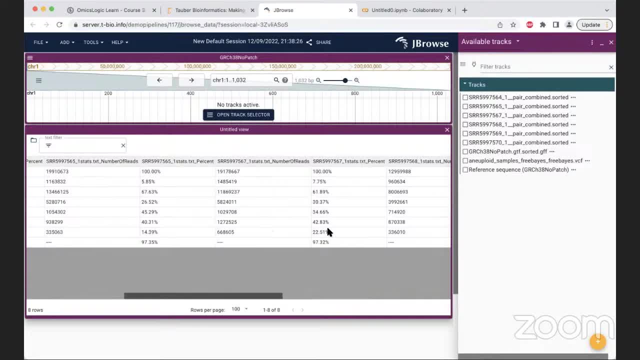 rate. you are generally happy with the status or with the overall alignment rate, and we have this information. that is the general alignment of the mapping table, that is the- with the quality of your sample. So I see that the alignment is excellent for my sample. 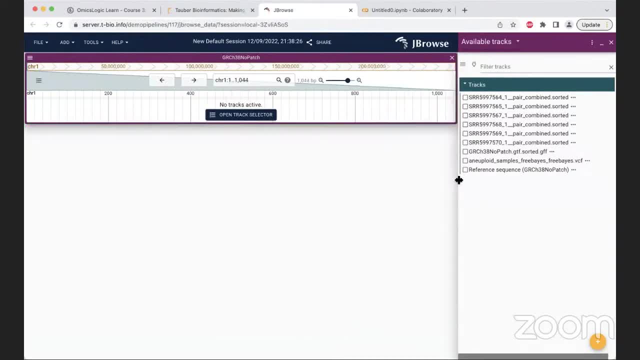 So I no longer need this information. I am going to close this over to available real estate, So I have several of the tracks that is available in this visualization platform. What do I want to visualize? I first want to see the frame of reference. that is reference sequence. 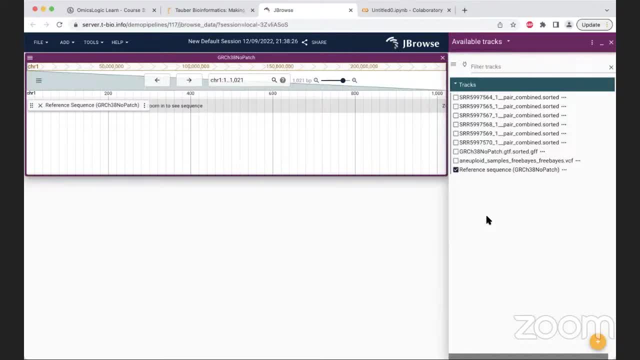 and so I enable that, and I also want to see the annotation of this reference sequence, or all the genes that are that can be named in this reference sequence. So I am going to enable the GTF or GFF file that is associated with the reference. 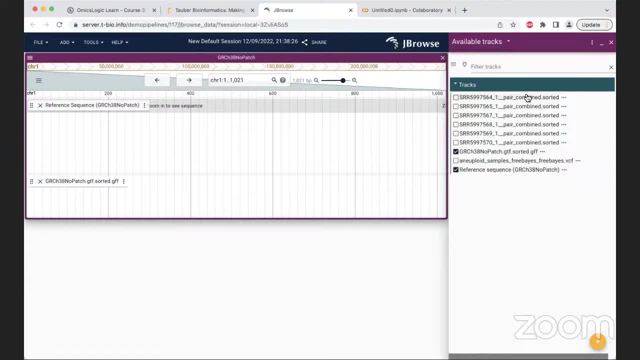 and that is given here, and these are all the reads that I have. You can actually enable them to visualize their alignment here. and but first I want to see the result of my variant calling pipeline by enabling the VCF file out, and I want to see. 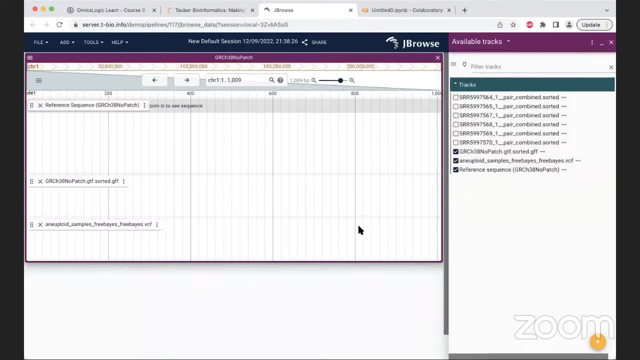 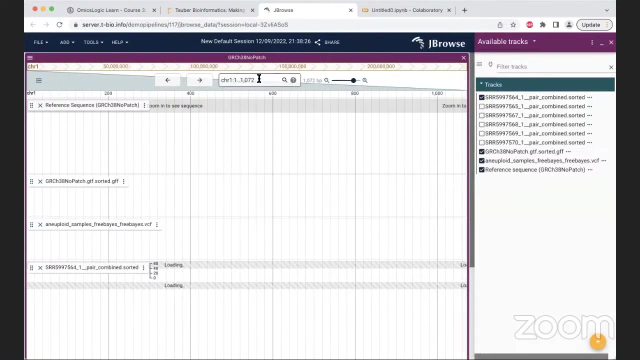 for one of the sample. due to time and due to memory constraints, I will just enable only one sample here so that I can visualize that. all right, when all of this is done and for this specific data, you will not visualize anything because the nature of the data, as I mentioned, the data, the 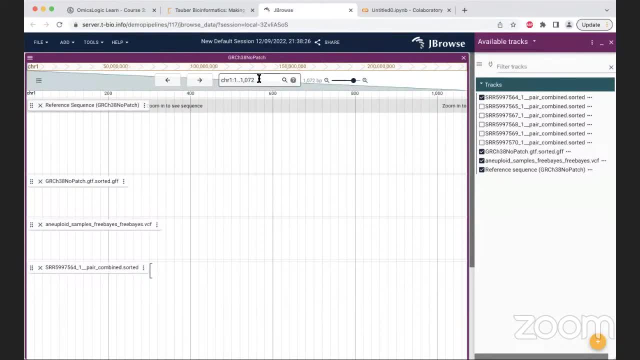 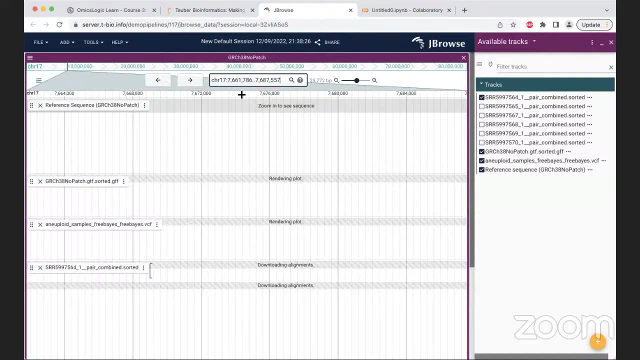 sample we have taken is targeted sequencing effort and that targets only tp53 gene. so when we type tp53 we can go to tp53. once you are in tp53 it's going to load up all the results and all the analysis that we have done so far. so it says: zoom in to see sequences, and these are all. 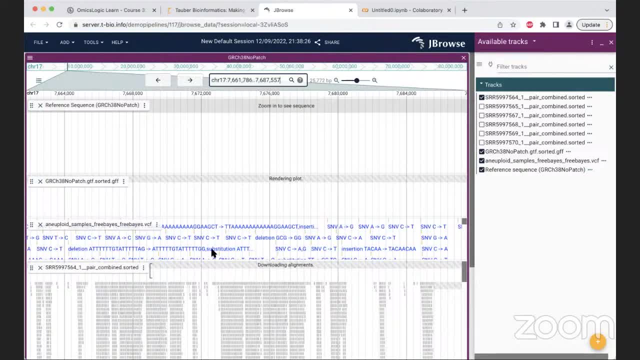 the reads that are mapped onto this specific portion of the sequences, and this is: these are all the variants that we have identified from our sample, compared to the reference sequences here, and the gtf file is still loaded, and this is the organization of the tp53 gene. so let me 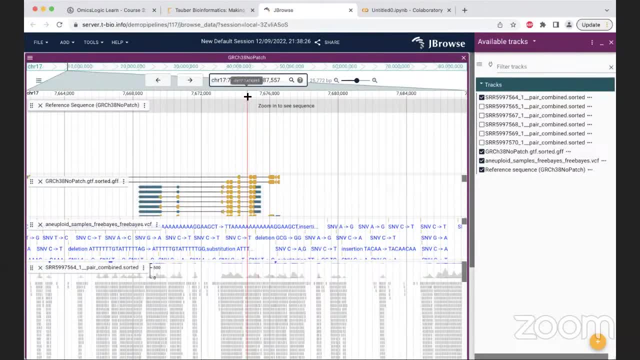 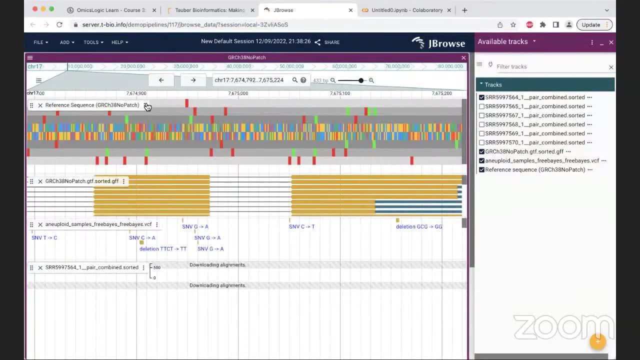 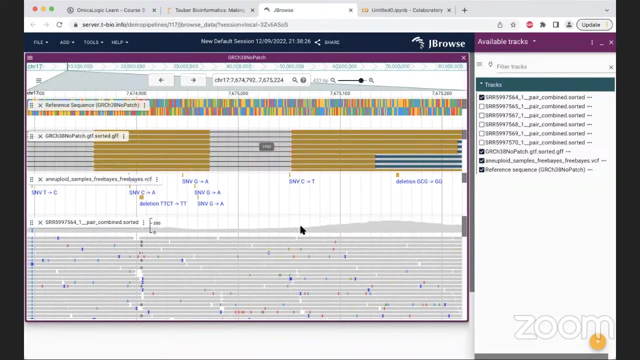 take a look at the gtf file and let me take a look at the gtf file and let me take a look at this specific portion. right, you can select like this, and that's going to zoom into this region, so I can make some rearrangement by not showing translation and pull this up, and I can see that. 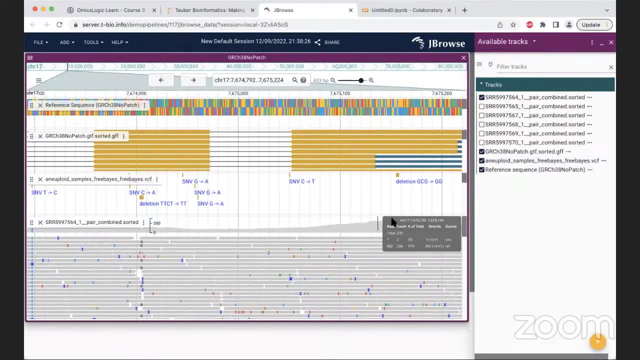 this will correspond to the. the height of this peak will correspond to the alignment of this read onto this specific region. and I can see variants at several places. let's see some. let's see some variants at several places. let's see some variants at several places. let's see some. 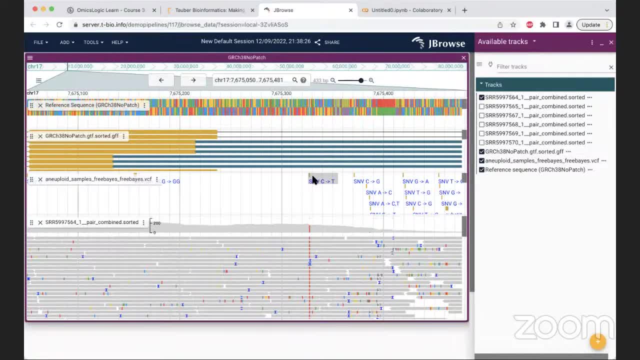 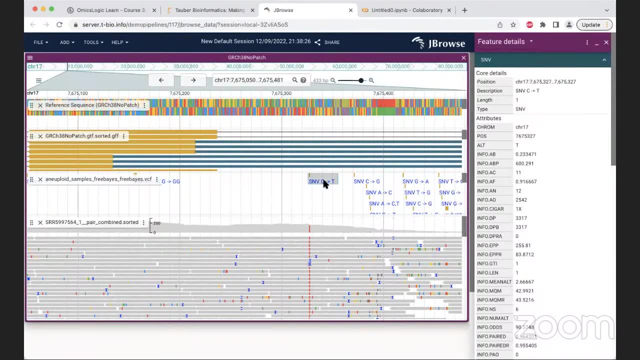 here exactly this point, right? so if you click on this one specific variant, it tells that this is a single nucleotide variant at this level where the c is actually converted or changed to t, and that corresponds to this specific variant, where you can see that and if you can read what's inside that. 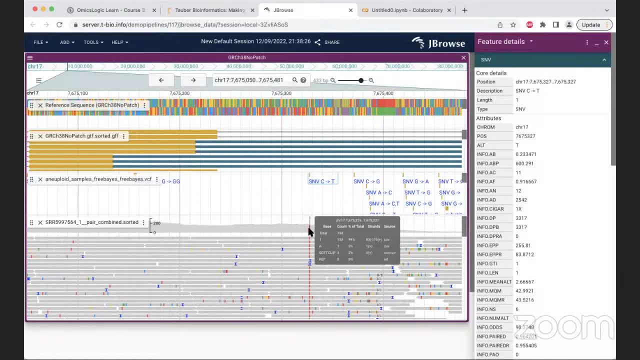 specific box which says and which corresponds to this red line or red bar and the red bars, the height of the bar signifies to the alignment score or confidence of this alignment to this at this specific position- and we have variant characteristics at this specific or this particular position. the position is like 7 million 675 326 and we have a 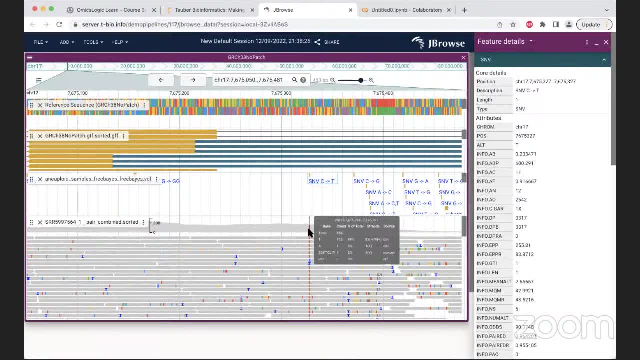 reference. we have an altered sequence here where the reference is altered to t at 99 percentage of the positions. we can see there and and and for. for understanding what is the reference, we can refer to the point mutation or single nucleotide variant at the vcf visualization where the 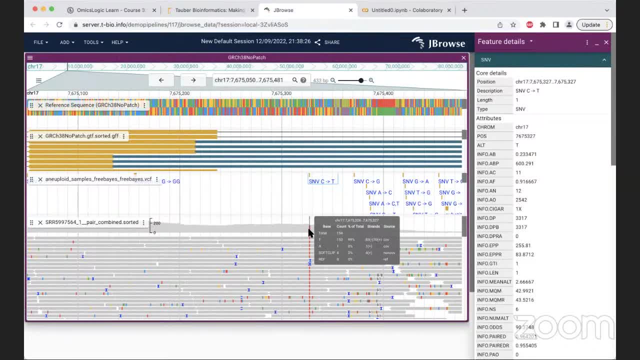 reference sequence is a reference nucleotide basis, cytosine- and now it is actually mutated or converted into timing. so additional information about this variant is actually found on the right side panel of this specific visualization. so this is just one example of how to visualize your variant and their alignment strength. this is again just only one specific for example. you 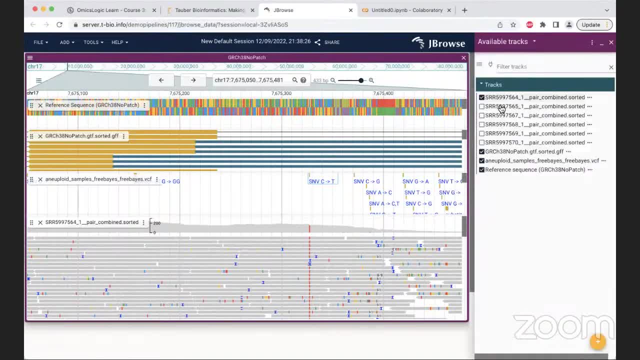 can take this feature details one specific track. if you enable all of the track, then you will be able to understand, or you will be able to relate to, how many of my sample harbor this specific variant and whether that is valid or not. for example, if you go. 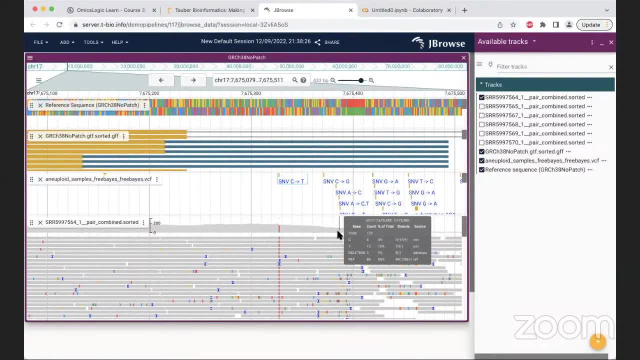 little bit on to the left or right you will find not so strong bar. right this has a very a tall bar and not so strong bar. that means, for example, this specific variant- that means the reference sequence- has 86 percentage of the reference nucleotide present in our sample. 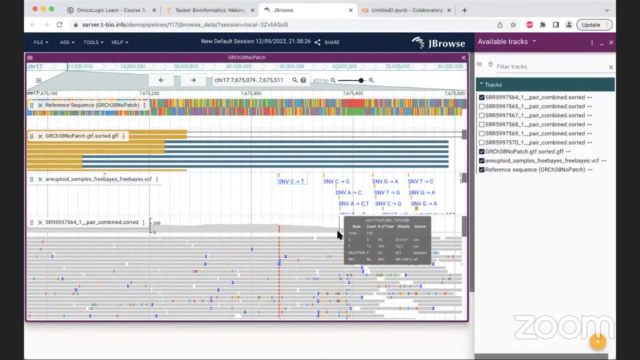 and only remaining um 13 or 14 percentage is actually distributed to several different other variants that we generally see. so this is how you can visualize the um, visualize your pipeline results, and i also wanted to show you uh available resources to perform some analysis in r to 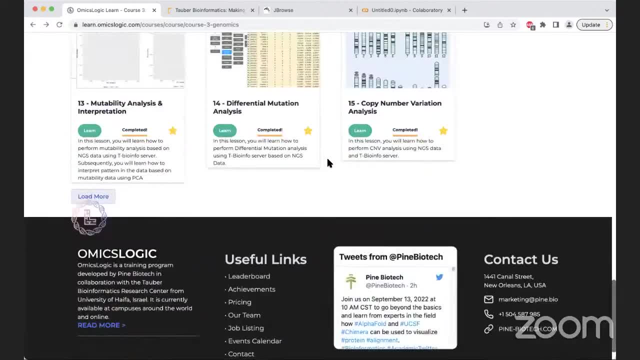 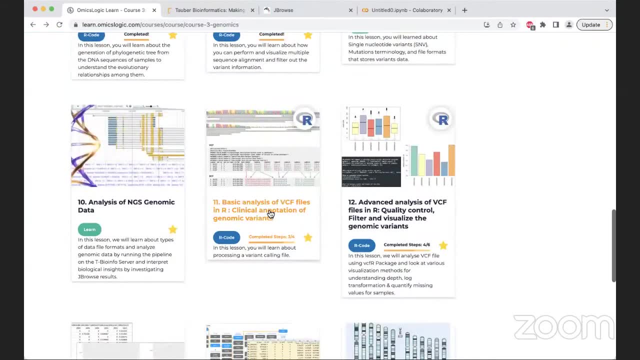 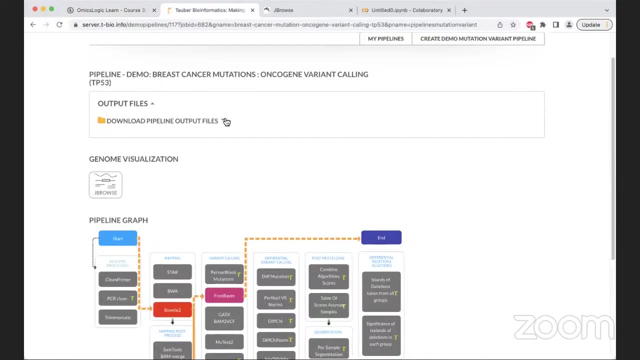 clinically annotate your results. i'm not going to go over them or i'm not going to demonstrate to them because of of not much time, so it's available here. um, so what you can do is you can take this vcf file, that is the output that that this pipeline gives you an output. right, this, this vcf. 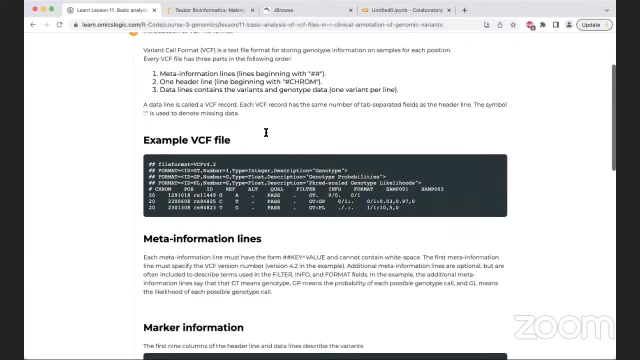 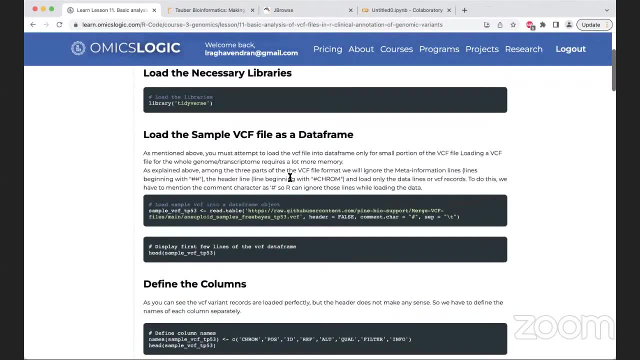 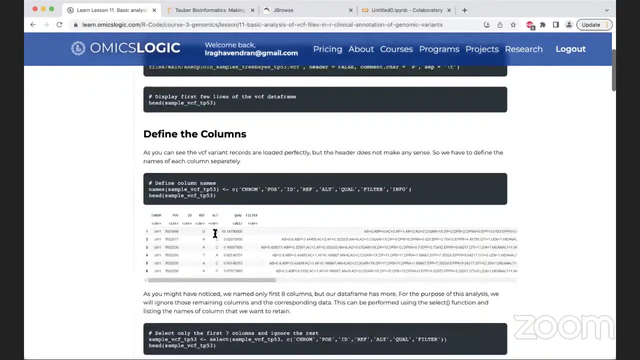 file. you can take this and load in an environment like r, where you can read each and every one of these variants and process them and store them separately. and it clinically available variants that are characterized in the clinvar database, and this database not only lists all the variants. 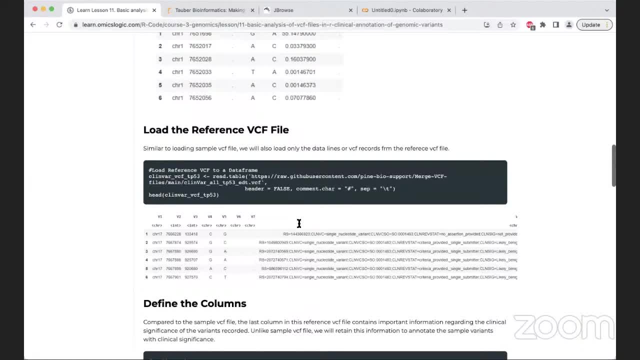 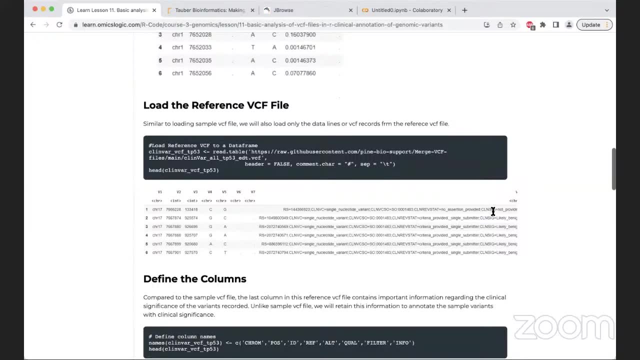 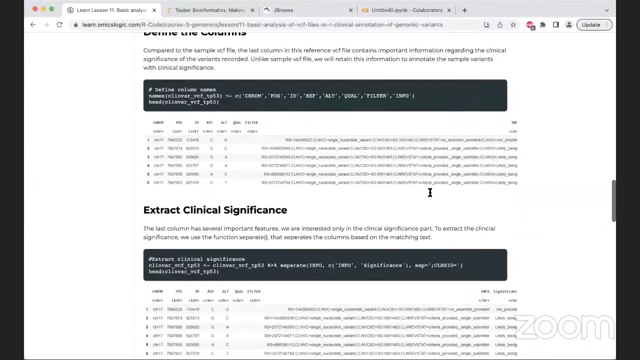 that are available for that specific gene or specific. you mean, in fact, for all of the genome and it actually it also annotates them as at the clinical significance level, like this being benign, or this variant being unannotated, or this variant being likely pathogenic, or this variant being clinically 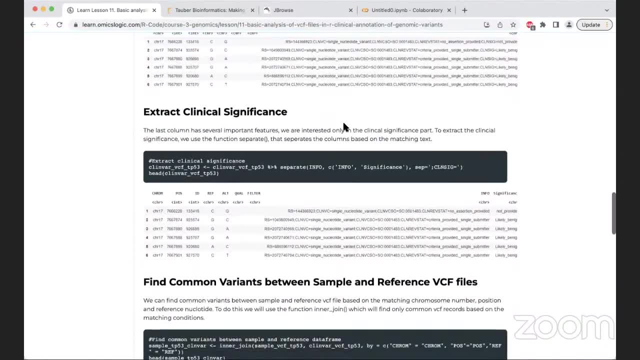 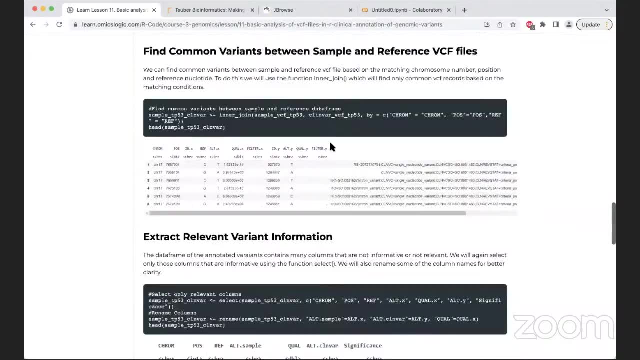 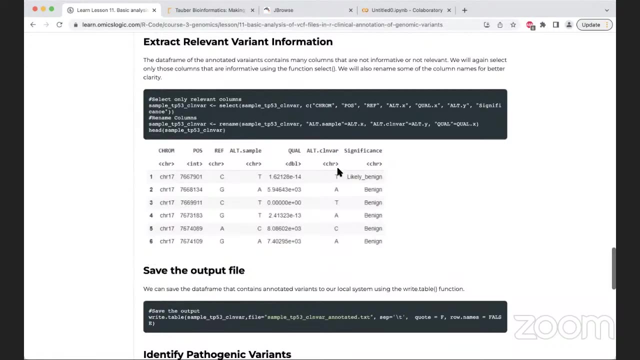 pathogenic. so we can go through several steps of selecting only clinically pathogenic variants and comparing that with the variants that we have identified for our sample and in this specific case we can actually identify six, six specific variant, and one of them being that we discussed so far and where the c is changed to t. i. 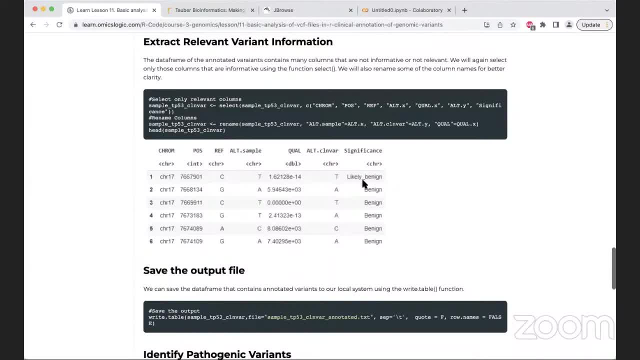 think that is. this is the, this is the same variant, and this variant is actually characterized as likely benign in the clean bar database, and we have several other variants that are also characterized as benign. and when you do this analysis- for, for example, this is a curated data and hence the only. 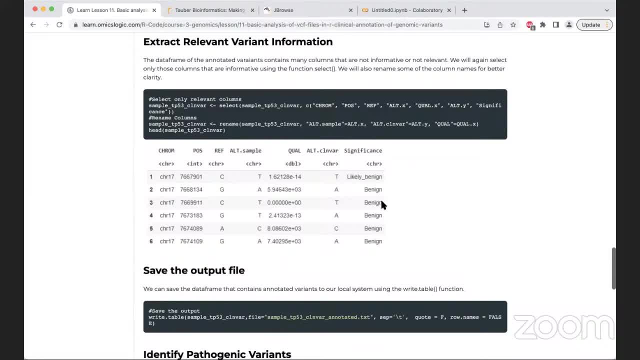 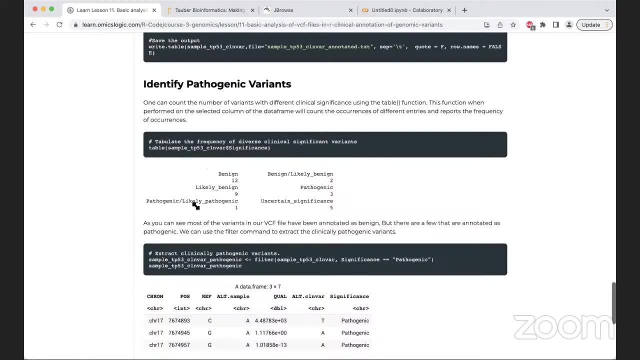 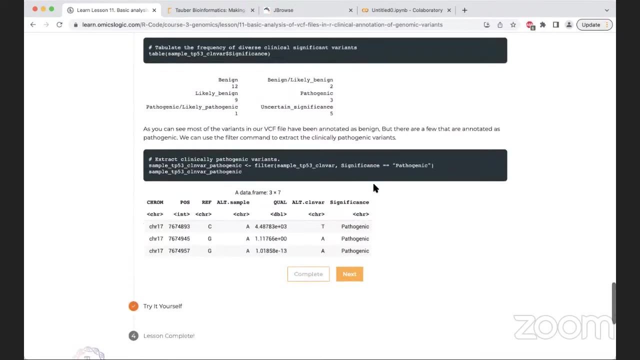 variants or only significance that we could identify is likely benign or benign. and when you do this analysis to uh for for all the uncurated data set, then you are likely to find some pathogenic variants. like we have four pathogenic and likely pathogenic variants and they can be: 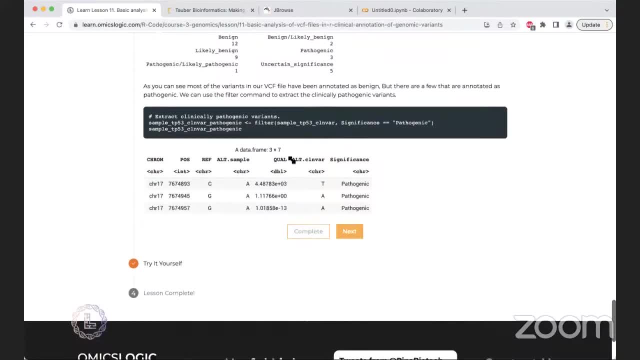 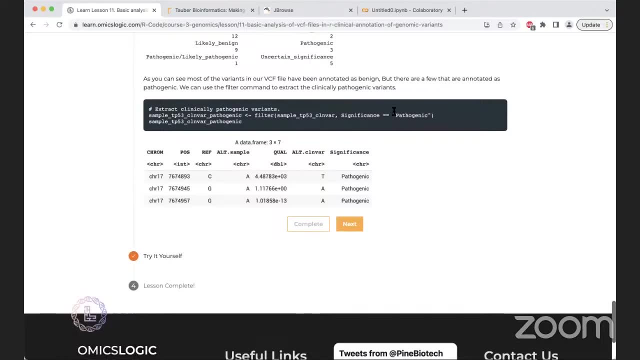 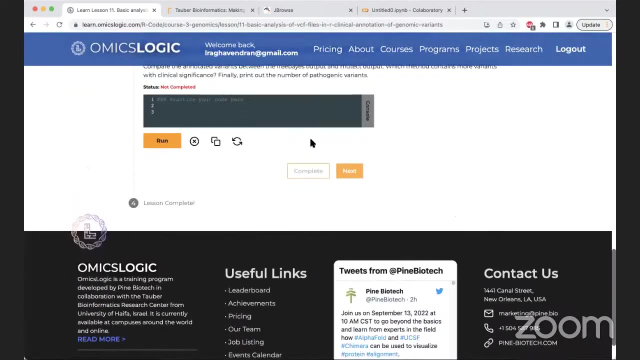 listed as here. so this is completely uh, yeah, this, this, uh, this. this type of analysis is uh that can be performed in in an environment like r, using all the codes that we have provided here, and, in addition to providing this code, we also give you a section where you can try out these codes in the r console that is loaded in. 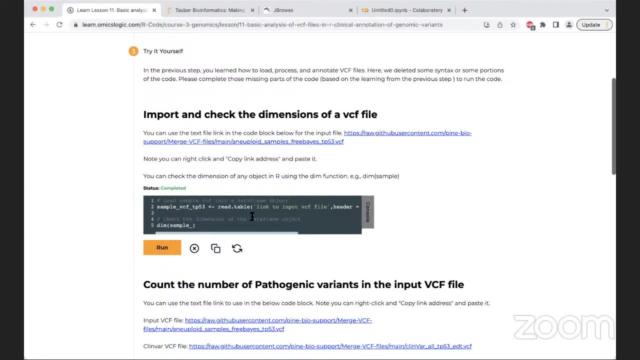 the back end itself, for example here, just by reading what it's supposed to be doing, for example, um, by taking the link, copying the link for the input file and pasting at the specific position uh, in the r function and this console. this challenge of this technical challenge, here is given for you to test your. 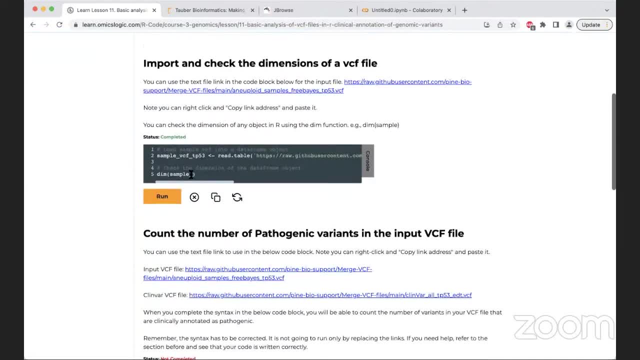 understanding of the code that we have given in this specific section. so here you can type: complete the syntaxes. we have left out some of the portions of the syntaxes so that you can get a sense of understanding can be performed. So when you complete all the necessary incomplete syntaxes and you 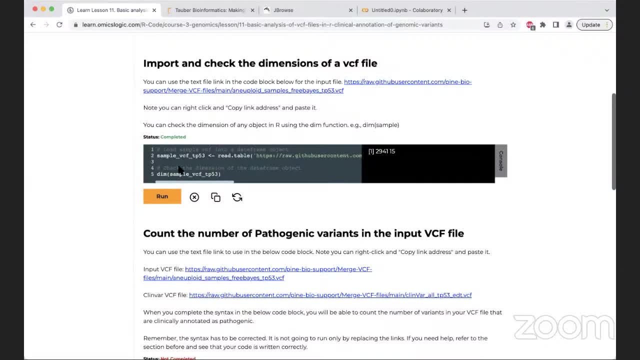 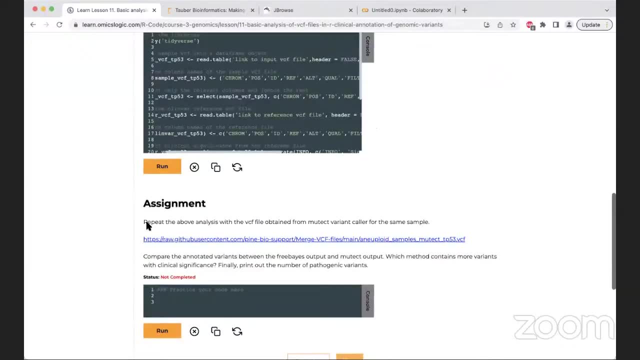 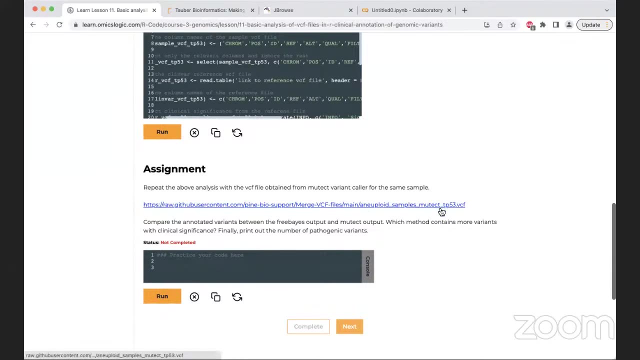 get success in running the code and understanding the code in general. So this is just one small example. We have several other examples of these using these methods and we have specific assignment where we have given you a console to try this assignment for a different type. 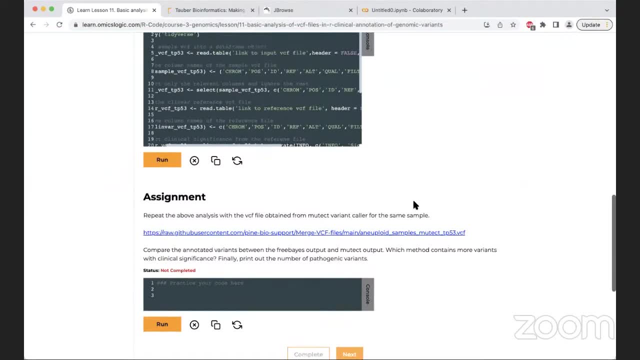 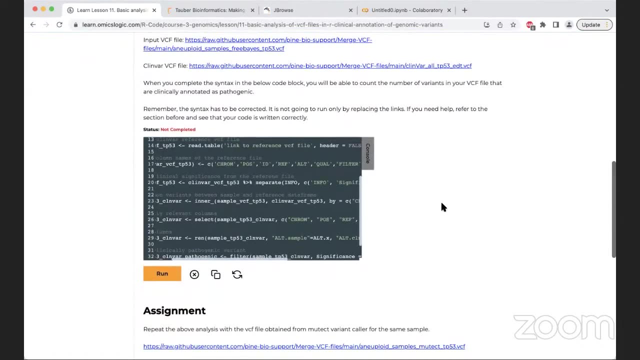 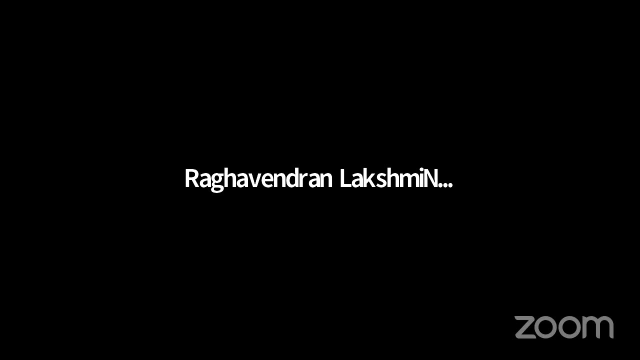 of data, or data that is slightly different to the type of data that we have been discussing in this specific lessons of that. So that will with that. that will conclude my lecture. So all of this and extensive discussion and step by step processing a step. 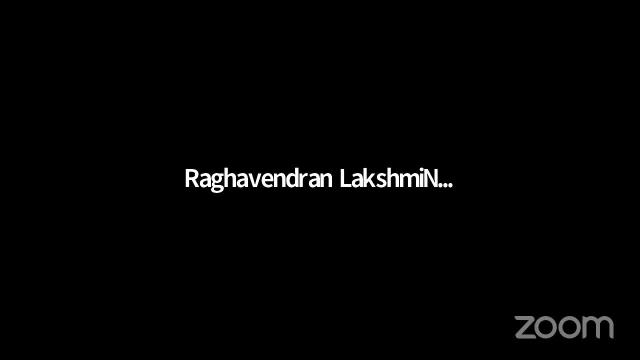 by step analysis, building types and everything is discussed in the next lecture. So in a live or asynchronous course type in the genomics program- and I hope to see many of you in the program- and we will discuss this and also several other impact code publications. 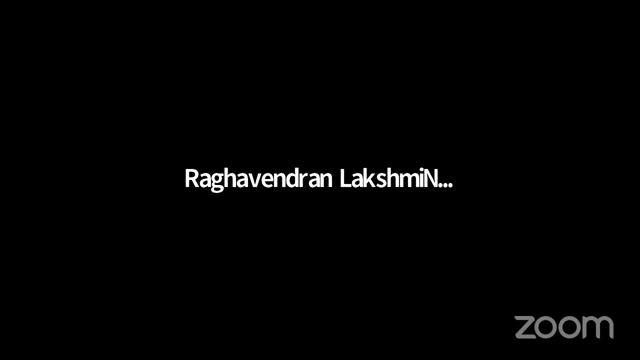 and example projects with which we can understand how to perform this analysis on genomics data, to understand the variance and their relationship to disease, to different pathological state of the genomic data. So thank you very much. So thank you very much for your time and I hope to see many of you in the next lecture. 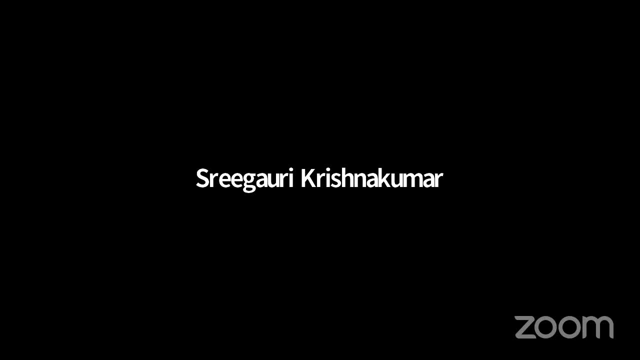 Thank you very much to Ms Parsh Thar to discuss about the fee structure and the associated resources that you get as a part of the program. So over to you, Parsh. Thank you so much, Sree Bhori. So let me share my screen. Sree Bhori, could you please? 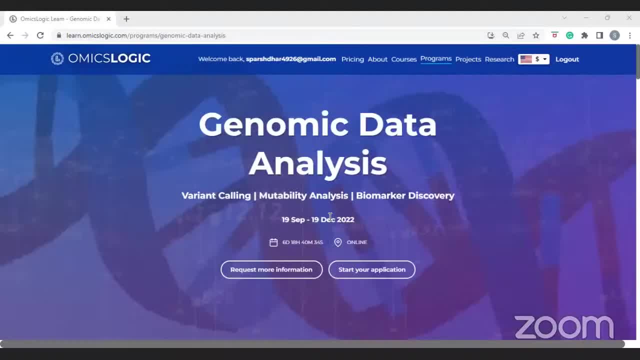 confirm that I am audible and if my screen is visible. Yes, the audio is a little bit. Can you hear me? Yes, we can hear you. Yes, we can hear you. Yes, we can hear you. Yes, faded, but otherwise, now is it. yes, it's all. 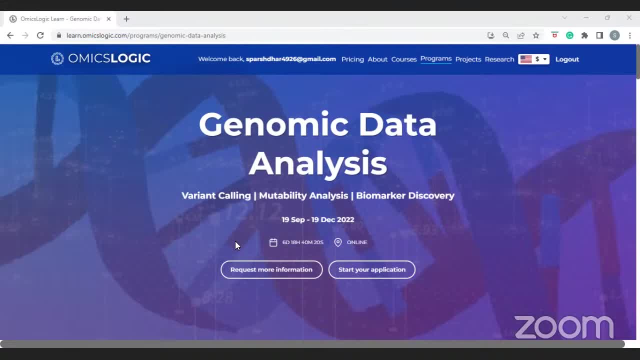 now the audio is fine. shri gauri, yes, it is, thank you, perfect, perfect, um so, um good evening, good afternoon or a good morning from whichever part or from you all participants are. so i am spurs her and i'm the marketing manager here at fine biotech, so i'll quickly 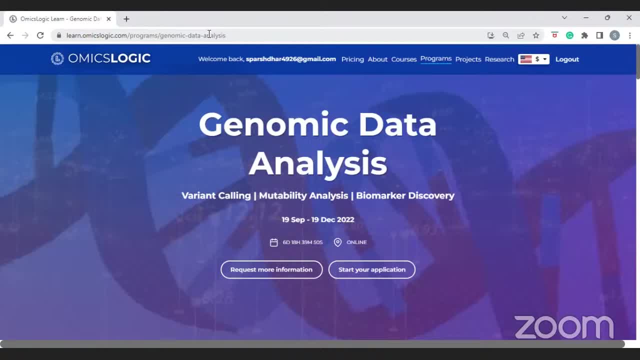 guide you through the fee structure of the genomic data analysis mentor guided program and also the resources which you will have access to if you enroll in this program. so this is the program page and here's the link the program page in the chat box you can go through. 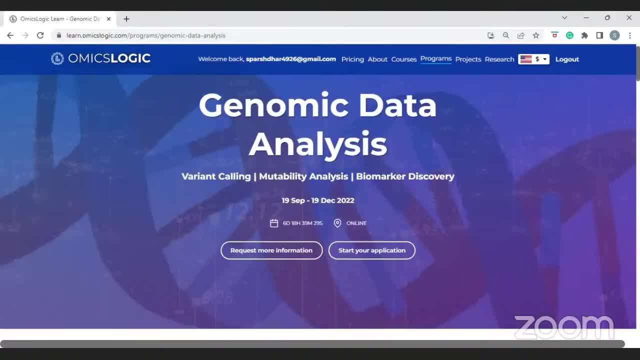 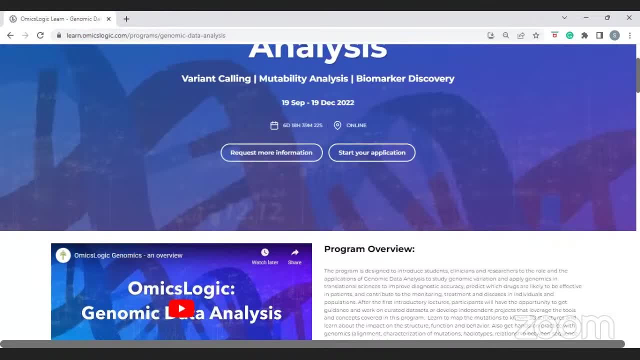 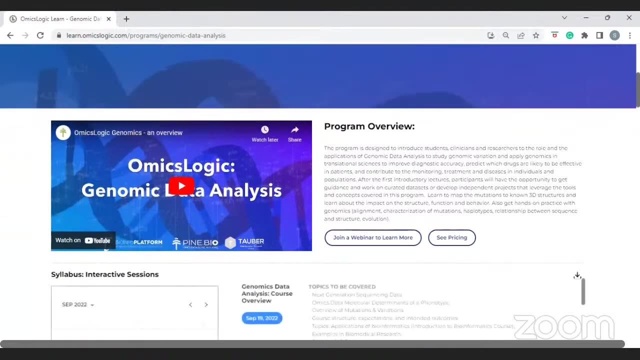 after the webinar ends. so the program is commencing on 19 september, next week, from monday onward. so those who are interested to be a part of this program, they can enroll themselves in this coming week. so when you scroll down you will see the program overview. what exactly? 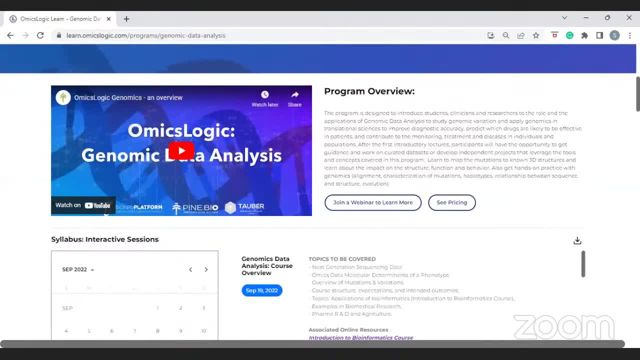 we will be covering the program, why this program is designed, for whom it is designed and what all applications or role in genome data analysis. the program will be covered by the manager, so i will just start talking about what is the genomic data analysis program. so it is. 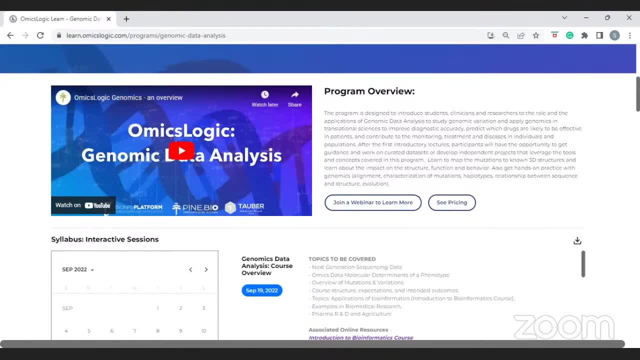 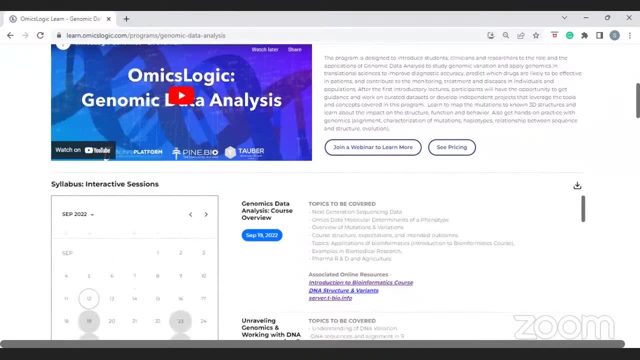 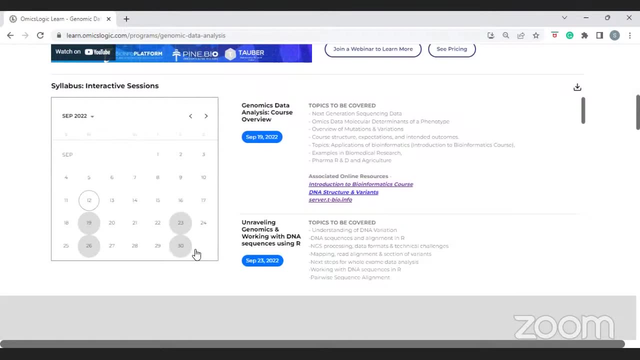 data analysis, you will be studying to discover the genomic variation or apply genomics in translational sciences, etc. So when you will move further, you will see an interactive session calendar where there are few dates highlighted. So on every Monday and every Friday there will be a session that will be conducted for this particular program, and it can be either: 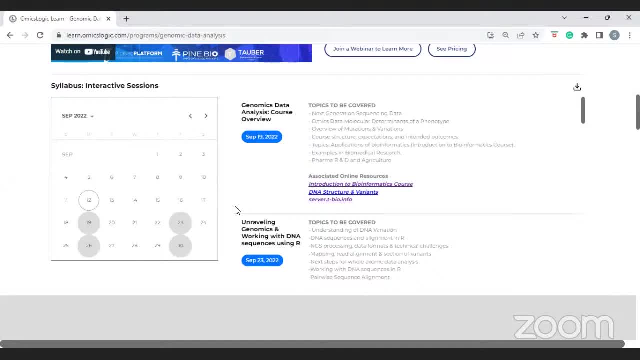 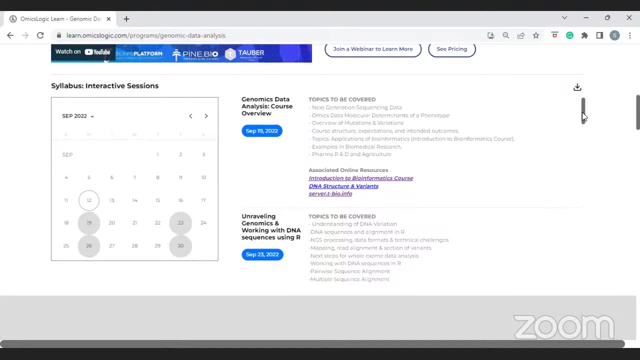 asynchronous session or it can be either live sessions. We will send you a calendar invitation accordingly. So, as you can see, here on the right hand side, there are different sessions which we will be conducting on genomics. So the first session that is on 19th of September. it is. 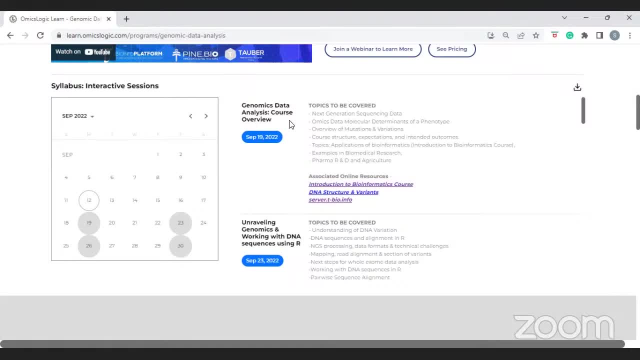 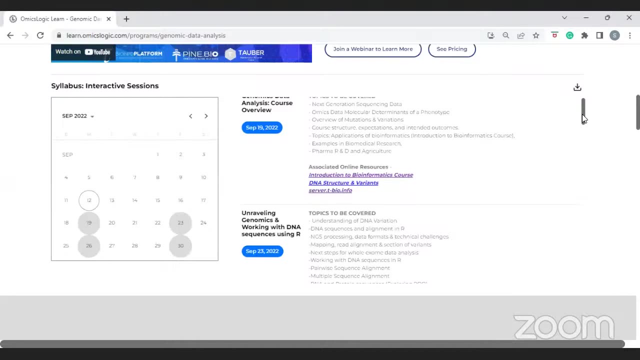 on genomic data analysis, where we will be covering the overview of the course, where there are different topics Related to next generation sequencing data, omics data, molecular determinants of phenotype. Then we'll be covering about applications of bioinformatics, introducing you about the 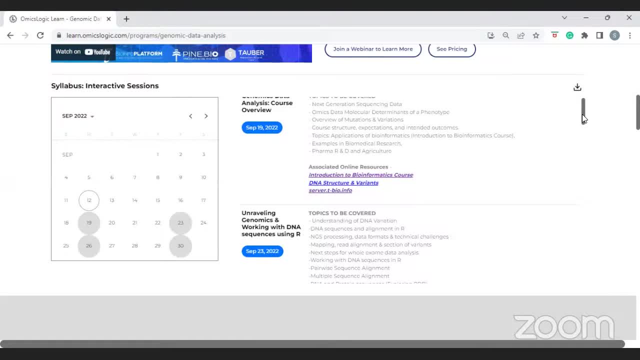 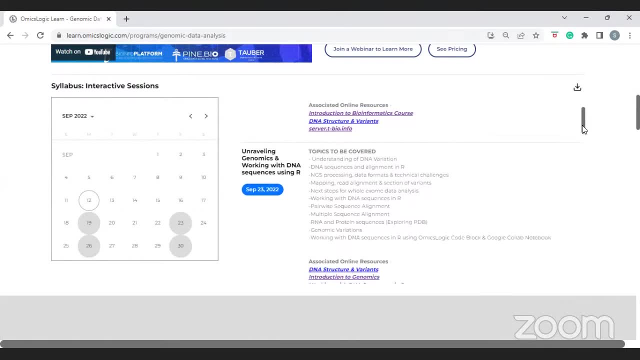 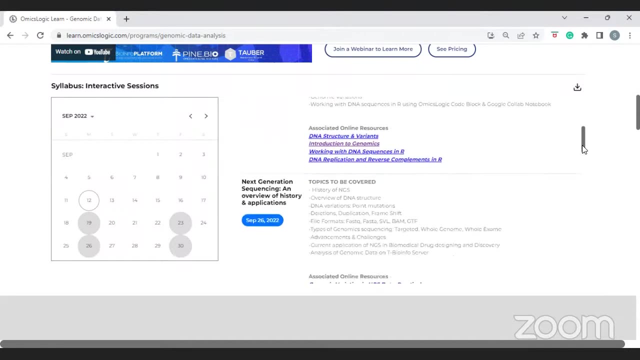 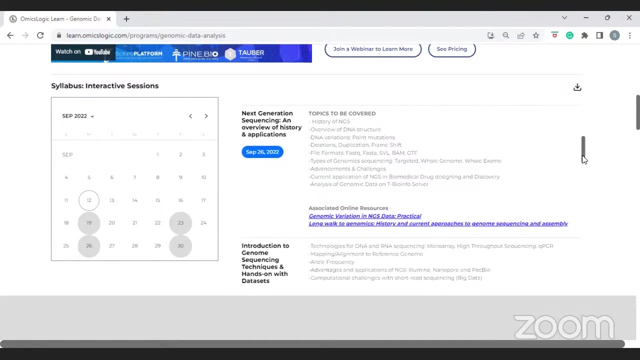 introduction to bioinformatics course, which we have different terminologies as healthcare, applications of pharma, R&D and agriculture, etc. Then, moving on to the second, we will be unraveling genomics and working with DNA sequences using R. Then the third is regarding the NGS, next generation, sequencing its overview, history and application. So, as you will see and 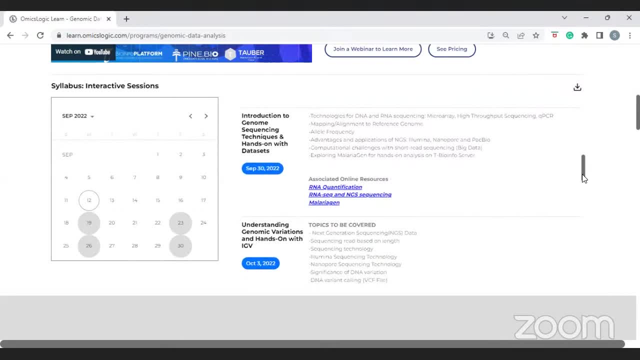 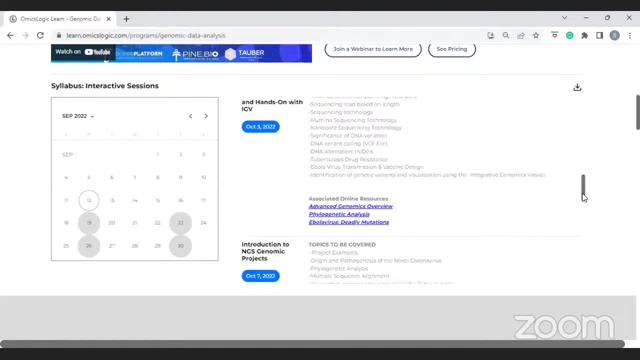 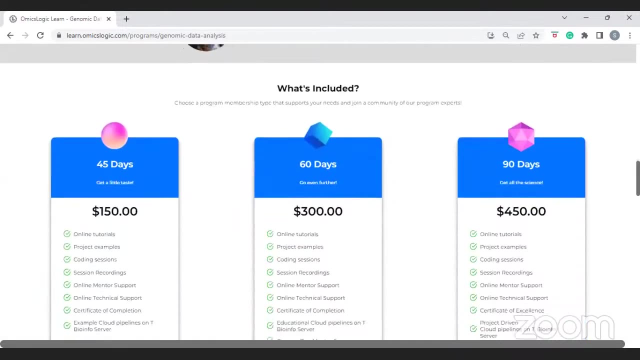 you'll scroll further, you will see the title of the sessions, the topics which we'll be covering and also the online associated resources which we'll provide you once you will enroll for the program. So now, moving further, if you'll scroll down, you will see three different tenures for 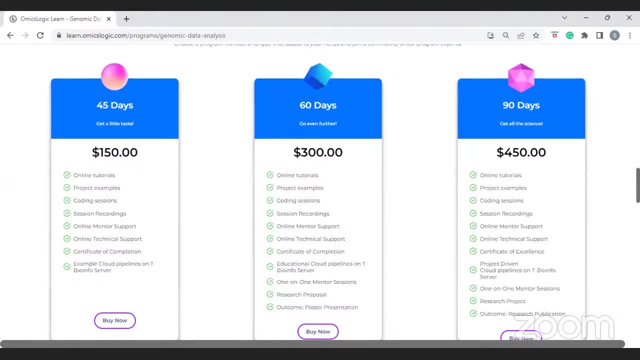 which you can enroll in this or register for this particular program. So, as you will see, the program one is 45 days, another is 60 days and then is 90 days. So what is the difference between the three tenures? In 45 days tenure, you will be going through with an extensive mentor-guided training. 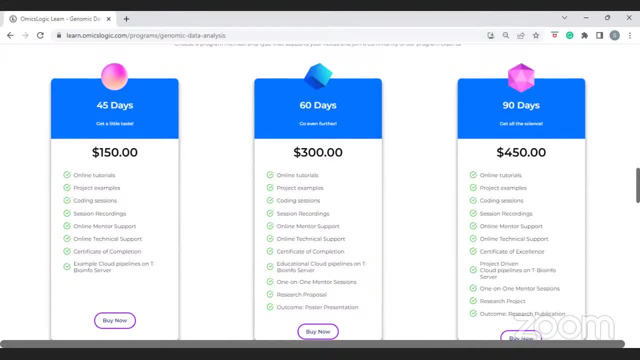 related to genomics, data analysis and the resources which we include. the common resources which we include in all these three tenure are online tutorials, project examples, coding sessions, session recordings, online mentor support via our Skype group or Telegram groups, online technical support and. 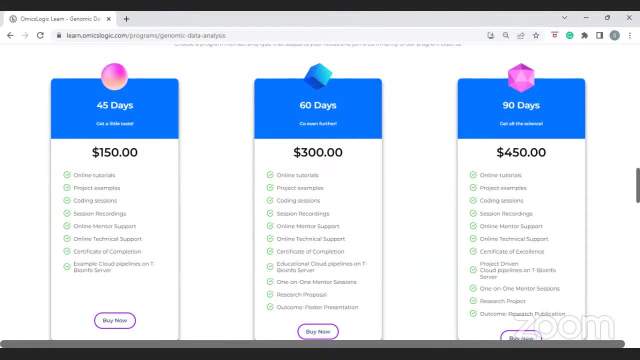 certificate of completion and example cloud pipelines on tbio info server. So in 45 days tenure, as I said earlier, you will be going through with an extensive mentor-guided training program In 60 days. other than other than the extensive training, you have two opportunities. one is 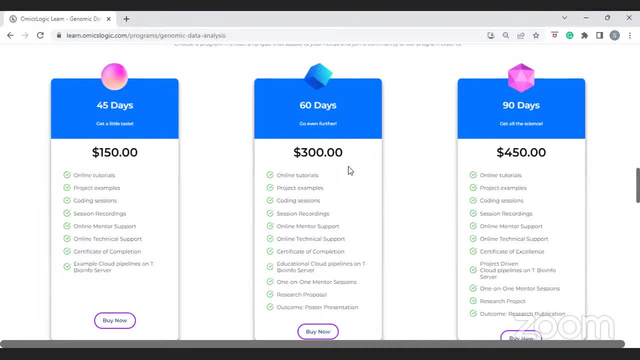 one-on-one mentor guidance, like you can go through with a one-on-one mentor guidance and then you can can, if you have any further query while going through the training part, so you can fix a one-on-one meet with the mentor- maybe your 15 to 20 minutes- and get clarify your doubts. secondly, you have an 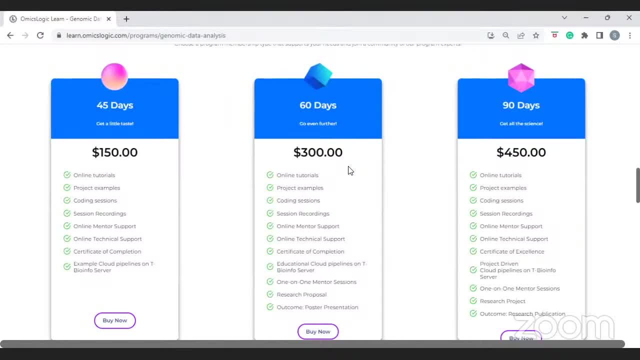 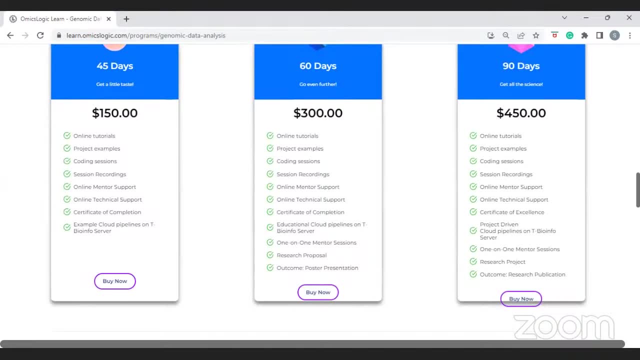 opportunity to draft a research proposal and present it to mentor for further evaluation and get expert feedback. and now, moving to the last tenure, that is, 90 days, you will be having the opportunity to draft a research project. you will be having an opportunity to draft a research project. 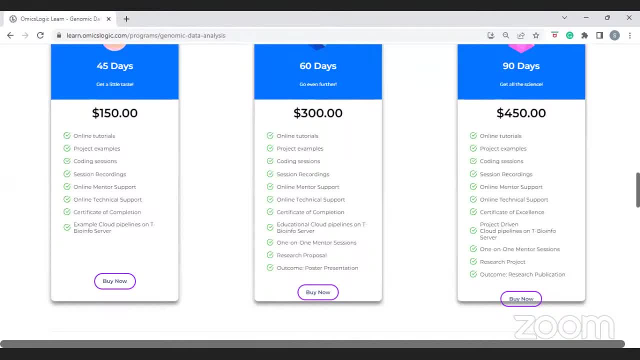 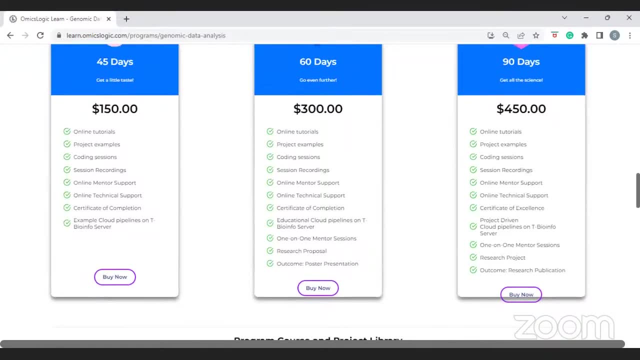 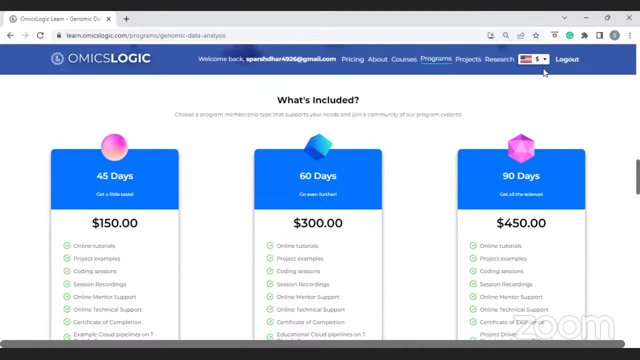 and get it published in a good peer-reviewed journal. so these were the resources which you'll avail in these tenures as mentioned, and the difference between these tenures. now, if you will see, here on the right hand side, top corner, there is a drop down menu. so those people they 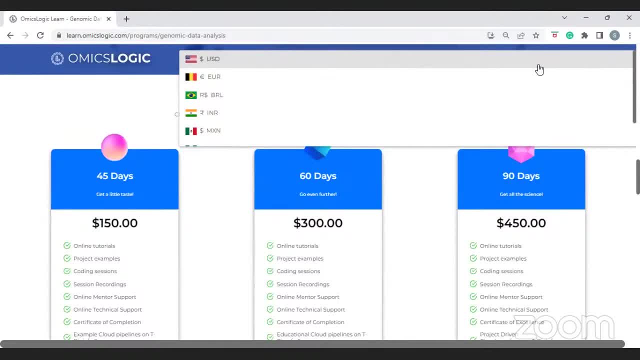 can can change according to their locations the currency of the program. right now it is in usd. if someone is in nigeria, they can go it for naira. if someone is brazil, they can go for vrl, for euros, for in inr, and so on. so please, accordingly, accordingly change according to your locations. so this was. 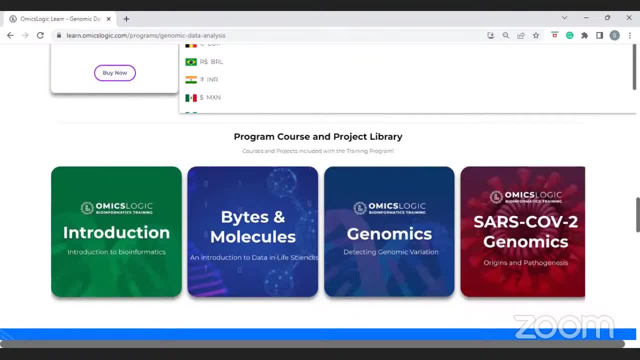 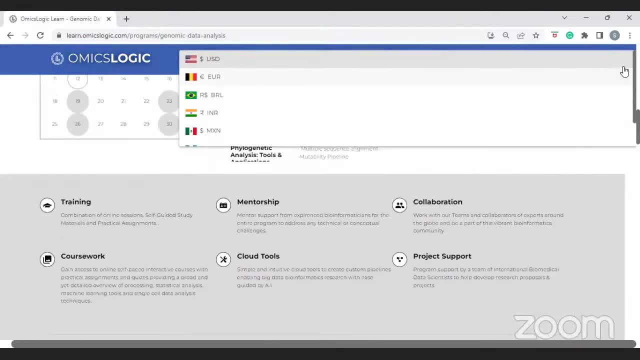 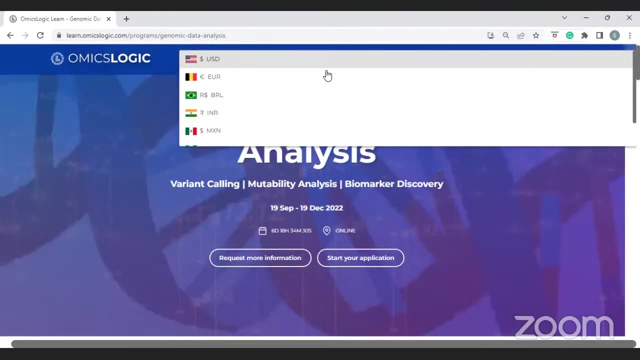 all about the resources, the fee structure of the program and also, yes, we have scholarships. so those who want scholarship to get themselves enrolled for uh, for this particular program, they can mail us at marketing at the rate, omics, logiccom and uh. we help and we guide you accordingly. so here's the mail id. i'm pasting it in the chat box. 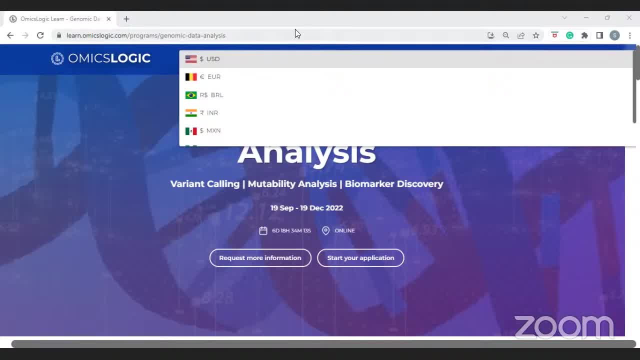 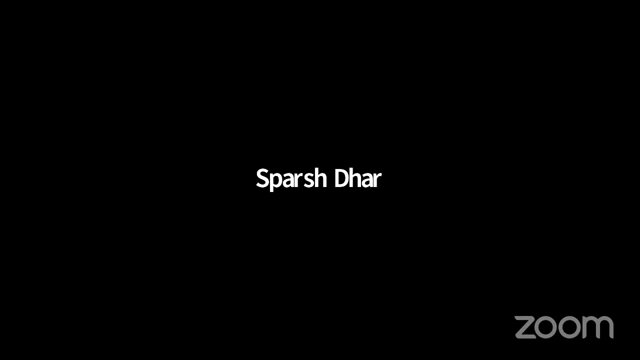 rest. uh, if anyone is having any queries related to the registration part or the resources part, please mention it in the chat box and i'll be here to answer your queries. thank you, hello, sri gauri. all right, thank you, yes, yeah, okay, all right, thank you so much. so, if anyone has any, 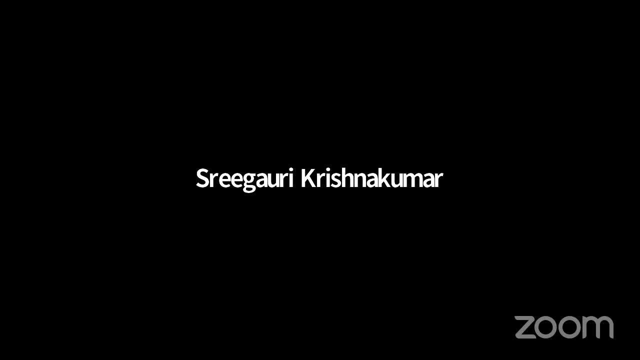 queries, please put them in the chat box and i hope to see you all at the genomic data analysis program. thank you, yes, parash has also shared her contact number in the chat box, so if you have any queries, please share in the number provided as well. we do have a query: will the program involve pack bioanalysis and illumina? 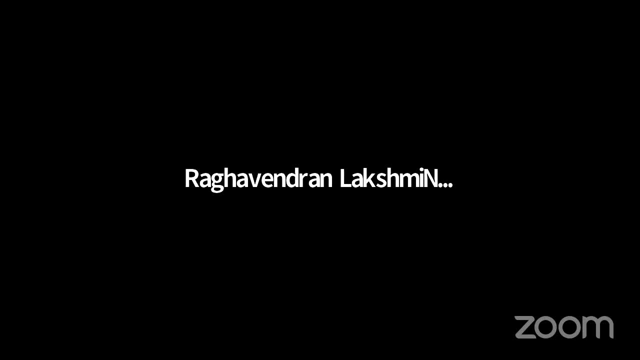 yeah, hello, stella. most of the data analysis will actually, uh, not, uh, consider long read, sequencing analysis or long read, long reads, um, but the logic is actually same. so we are focusing mainly on the short reads, uh, and that are from the illumina and from many, many other methods which